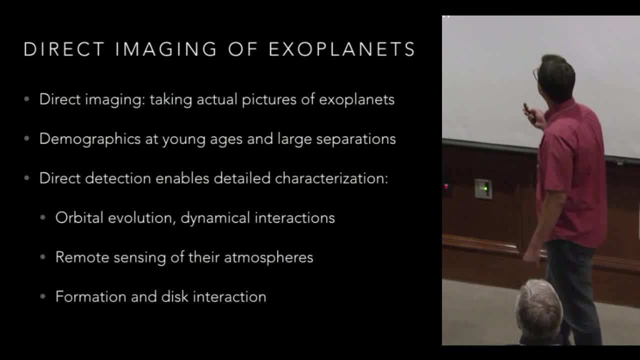 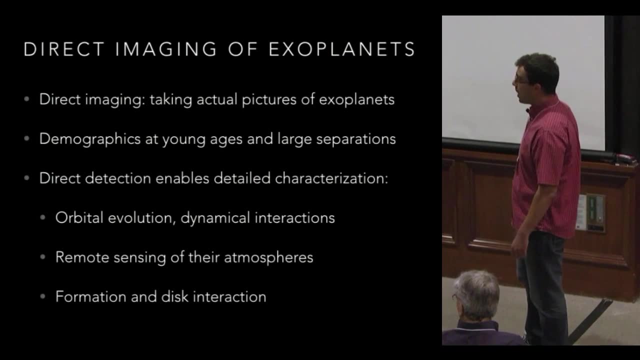 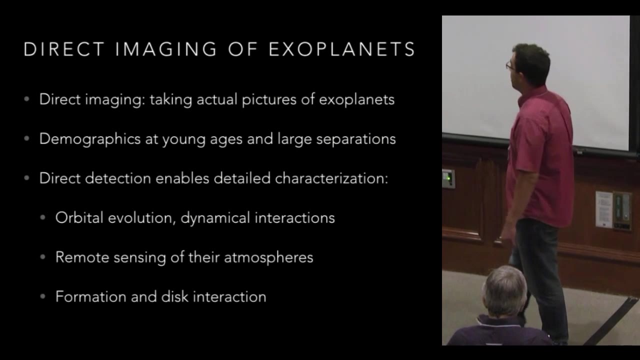 Alright, so why direct imaging? Direct imaging is, of course, beyond taking pretty pictures of exoplanets- For now we are interested in demographics at young ages and large separations. But above all, direct detection enables us to do a lot of things. 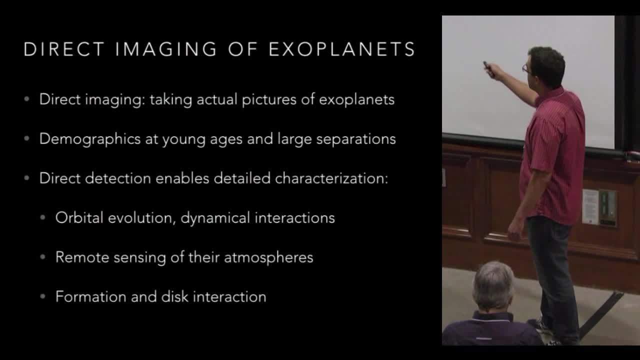 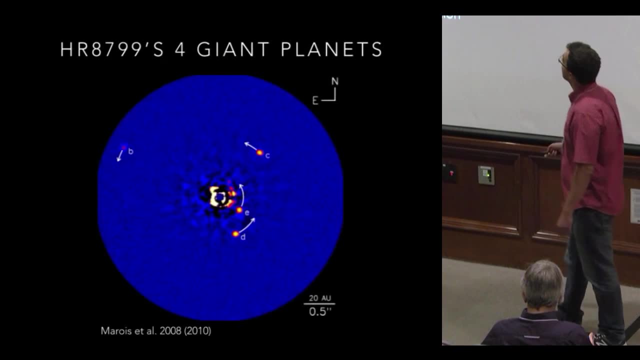 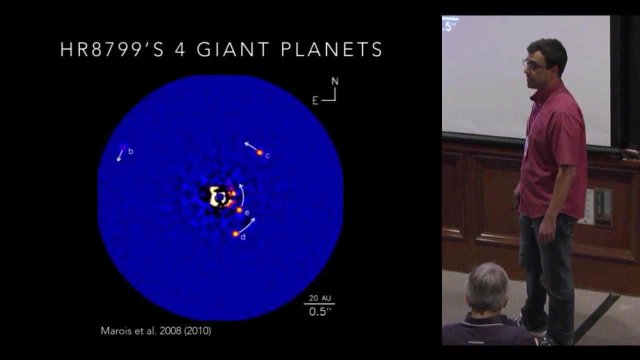 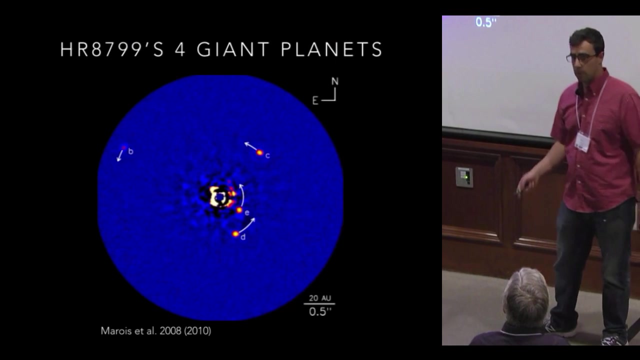 First detailed characterization. So I mean orbital evolution, dynamical interactions, remote sensing of atmospheres and disk interactions. Okay, so a few pretty pictures here. You are all familiar with this famous picture of HR8799.. B, C, D and E, Discovered in 2008 and then E in 2010 by Christian Marois using the Keck telescope. 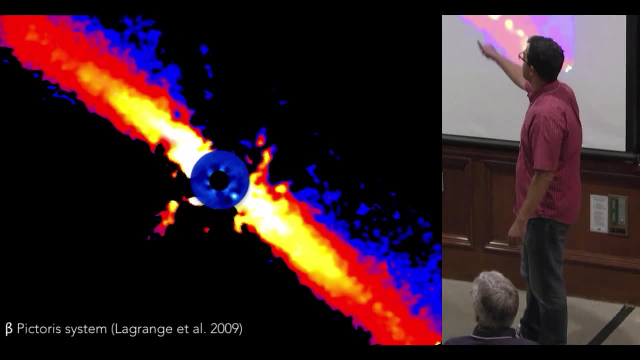 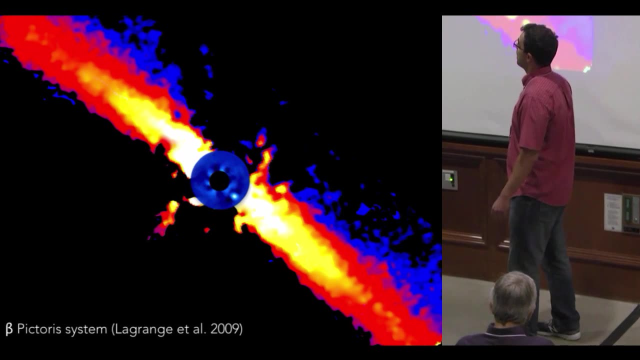 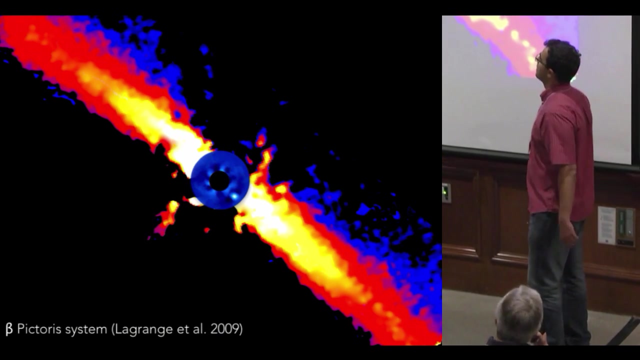 Here is another one. This is a montage, So you see here the debris disk from Beta Pictoris, Famous system discovered in 1986 with a small ground-based telescope showing this giant disk of dust and some gas. And the disk was discovered to be warped about 10 years ago. 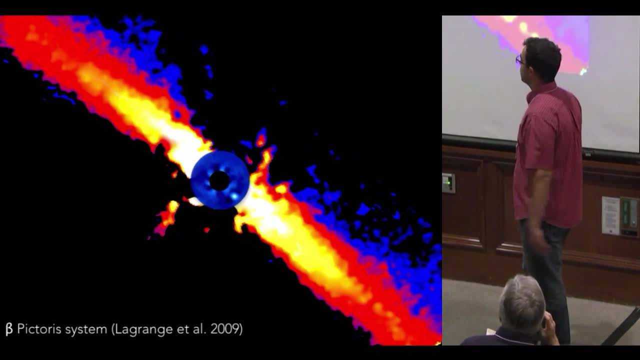 And that pushed us to infer the presence of an exoplanet that was discovered in 2010.. Okay, And then in 2009 by Anne-Marie Lagrange at the Very Large Telescope in Chile. So this is here based on the same and unique data sets processed in two slightly different ways. 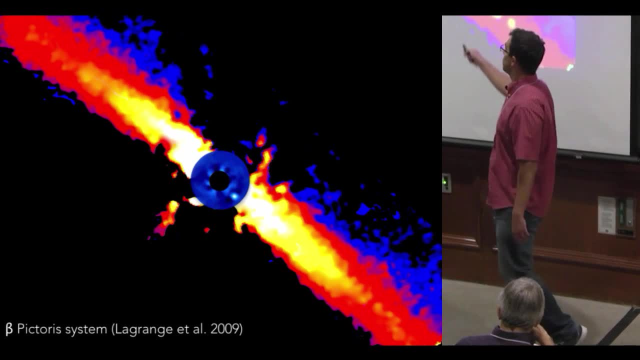 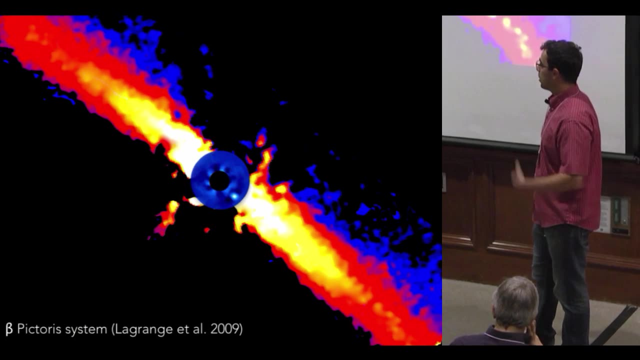 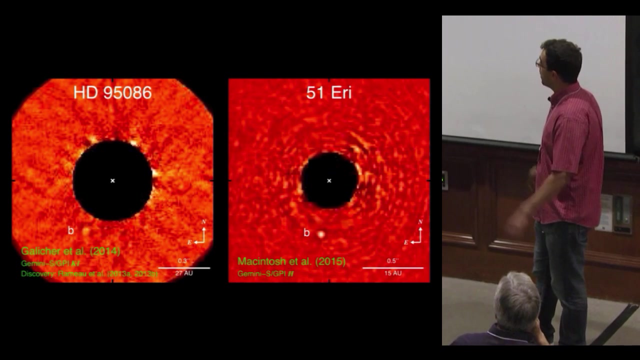 One to make low spatial frequencies emerge from the image and one to make point sources emerge, And those two were assembled together to show this picture of the whole Beta Pictoris system. A few other examples of young giant planets discovered by direct imaging over the past 10 years. 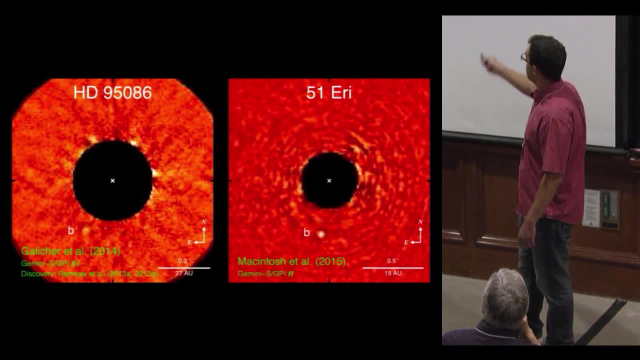 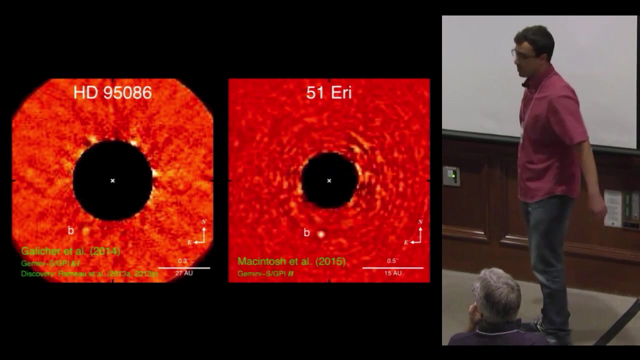 Direct imaging over the past 5 years and this one more recently last year. So this is HD 95086. And this is a very low mass companion here And you see the striking resemblance to the 51 area image. So the challenge in these two data sets was the faintness of the exoplanet here. 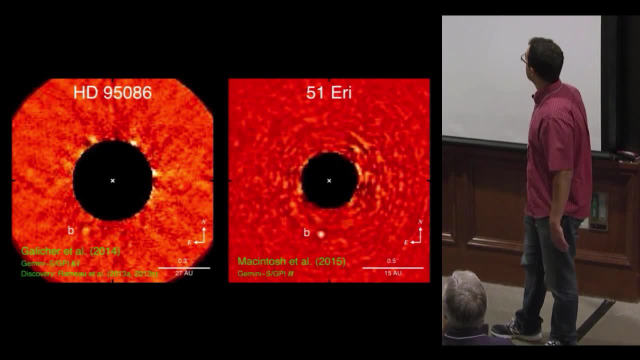 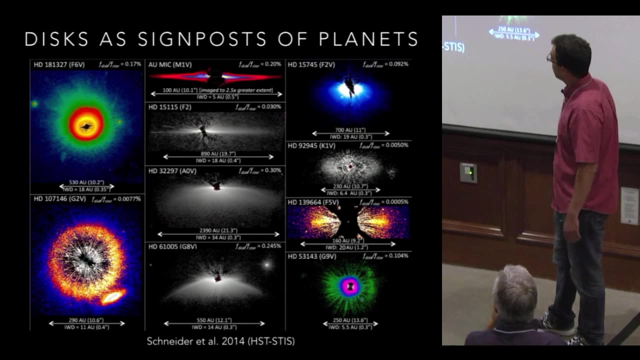 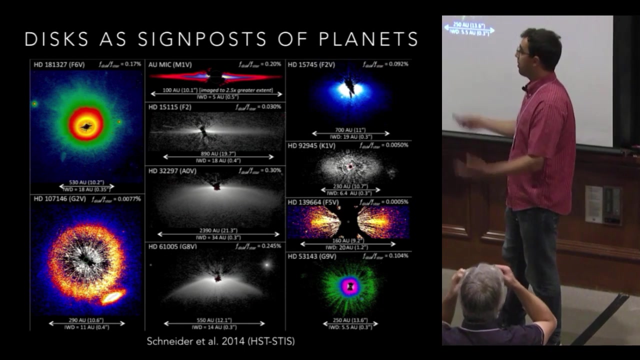 Which is just of a few Jupiter masses and a few million years old. And you see, here it's very above the noise. And this is really the challenge of direct imaging here. I'll go over this in more detail later. So, of course, direct imaging allowed us to discover a wealth of debris disks. 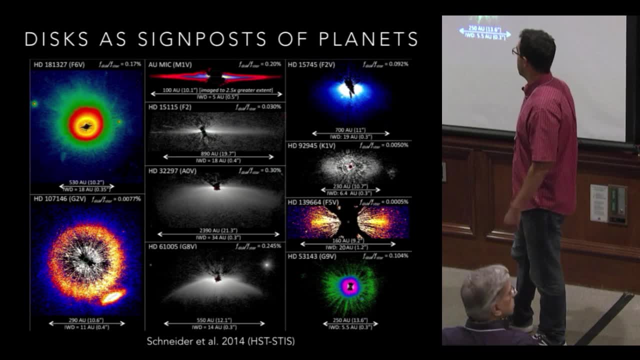 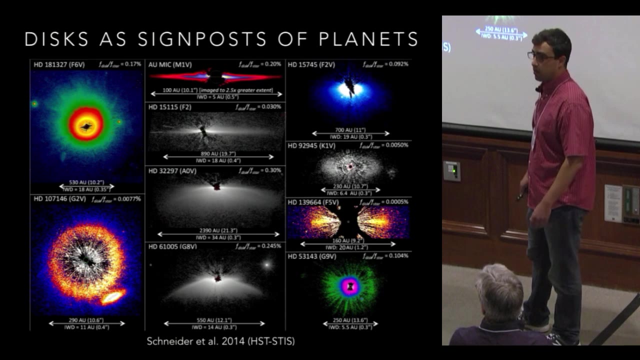 And this montage is from Glenn Schneider, using mostly STIS on the Hubble Space Telescope and modern post processing techniques. Many disks were discovered this way and these can be really interpreted as signposts of exoplanets. So debris disks are stirred by unseen planets that make planetesimals mash into each other. 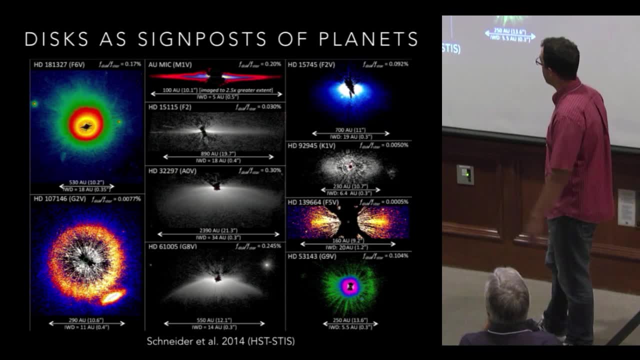 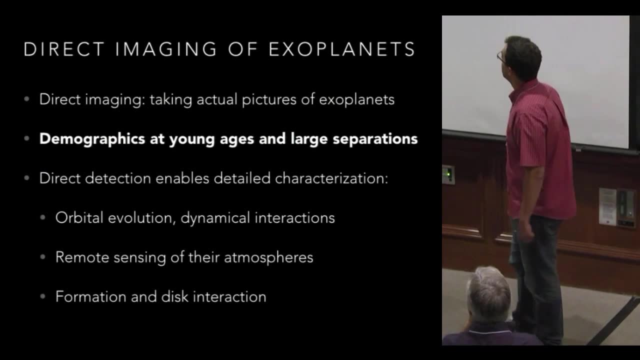 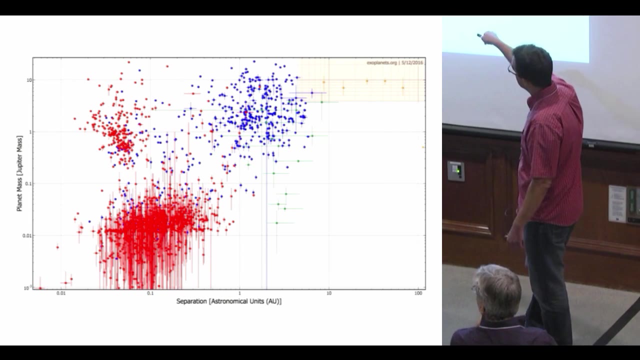 and create this dust population that replenishes over time. Alright, so direct imaging again for now is focusing on demographics at young ages. So you are all familiar now with this plot that you have seen probably a hundred times this week. So this is a log-log plot in planets. 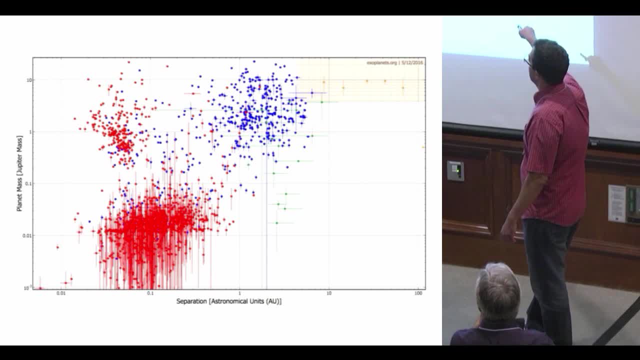 Planet mass and separation in astronomical units. You see the planets from transit and Doppler spectroscopy. You see planets from microlensing And you see here in this corner, for massive and large separation objects. you see the planets discovered by direct imaging. 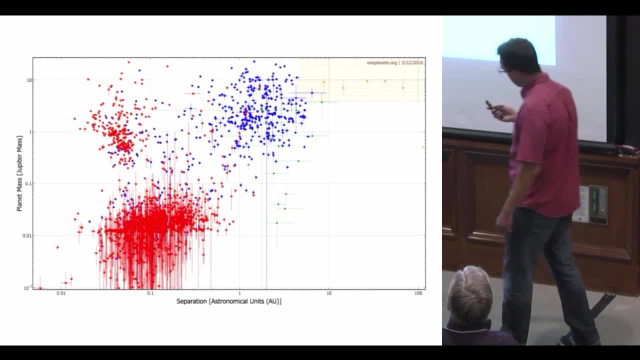 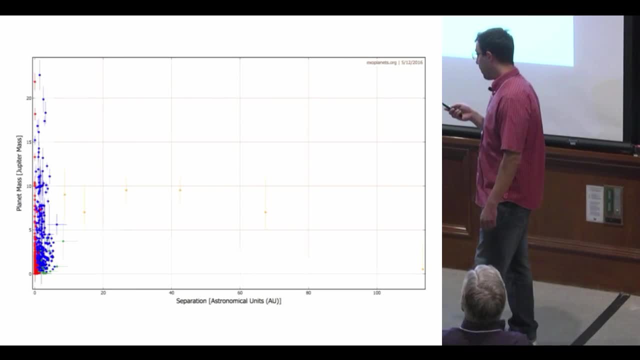 I find this plot a bit unfair. It's always presented in a log-log space. Actually, the ground covered in volume by direct imaging method is much larger. The fact is that we don't see many planets there, And the reason is simply that nature does not produce planets. 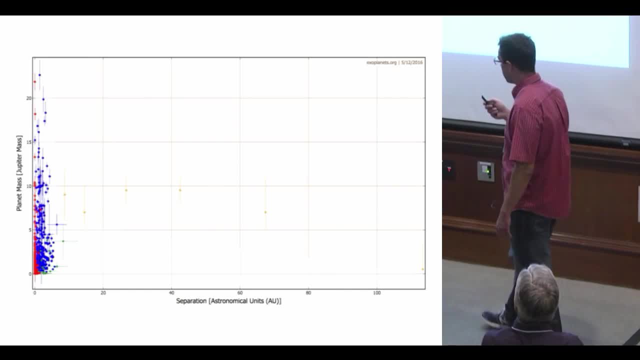 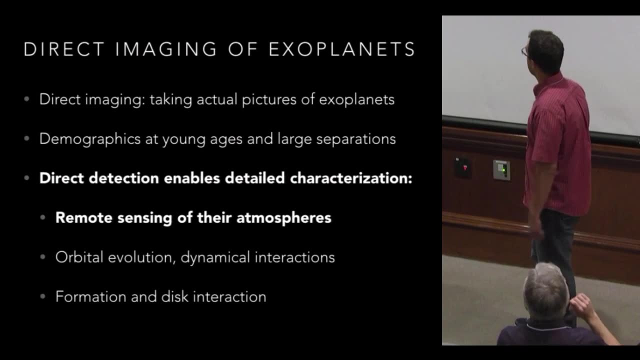 that are massive at large separations. That's what we've learned basically over the past 15, 20 years by direct imaging. But direct imaging when one finds a planet is very powerful in that it allows us to do direct spectroscopy. 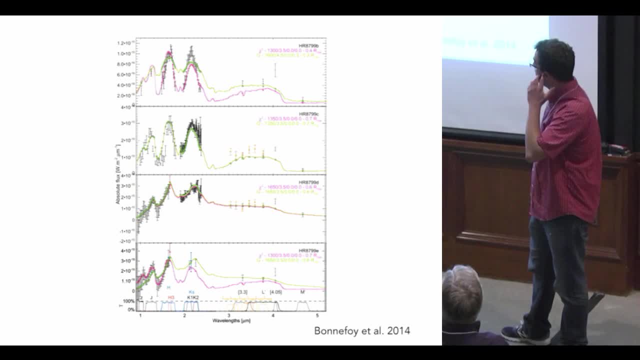 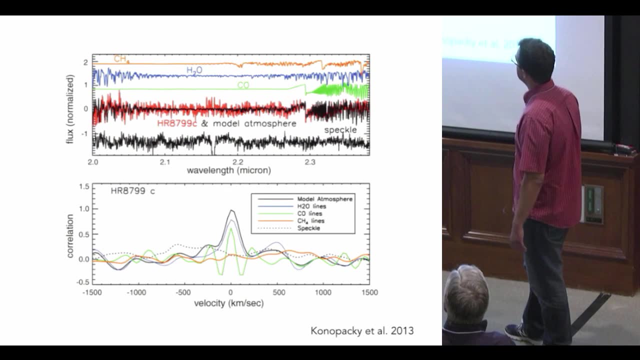 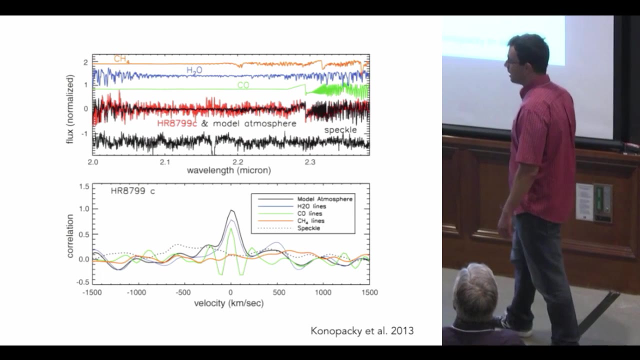 And this is here a panel showing the spectral energy distribution of all four planets around nature. This is HHR799.. This is here one in particular, done at medium to high spectral resolution. This is HHR799-C spectrum in K band made by OSIRIS at the Keck telescope. 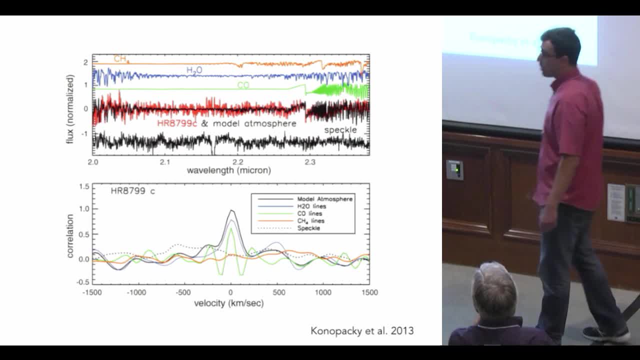 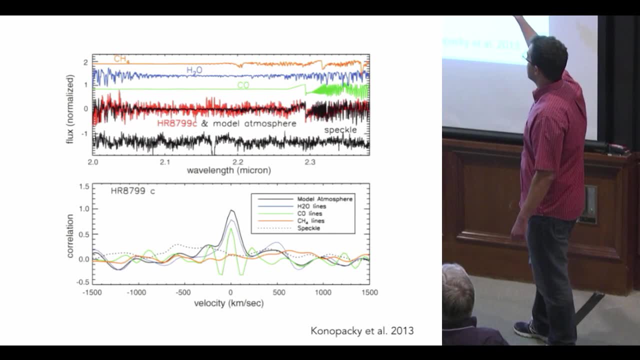 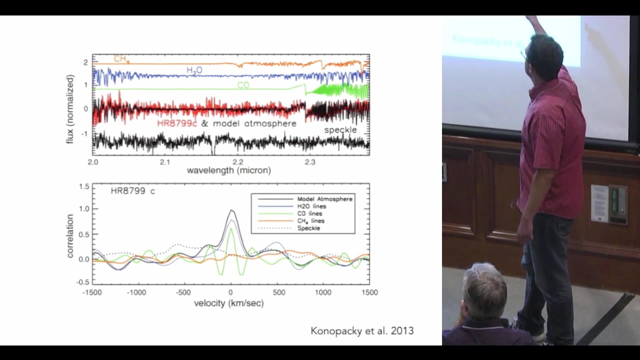 And you see here, this is not noise at all. These are real spectral features. You can see that molecules like methane, water and carbon monoxide are all represented in this spectrum, except maybe for methane, but it's still under debate. So when you cross, correlate these templates of high resolution molecules. 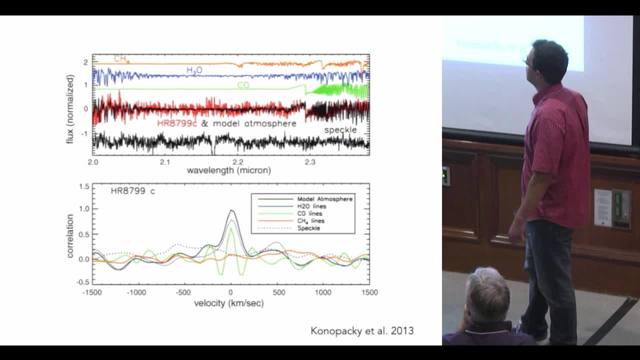 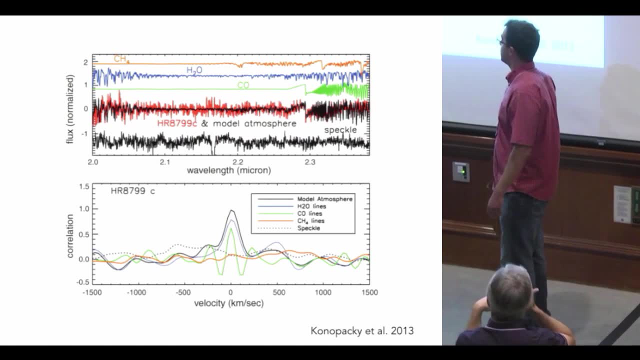 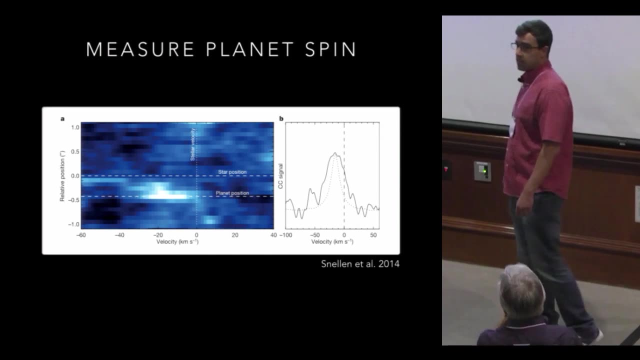 seen by high resolution spectroscopy. you see these correlation peaks that emerge in the data that are very good and very powerful indicators of the presence of these molecules in the atmosphere of exoplanets. So high resolution spectroscopy is extremely powerful and very promising. 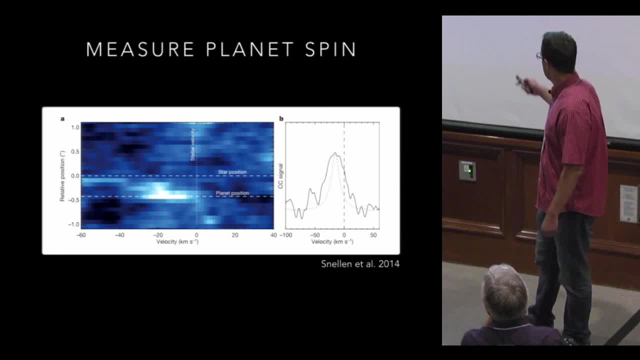 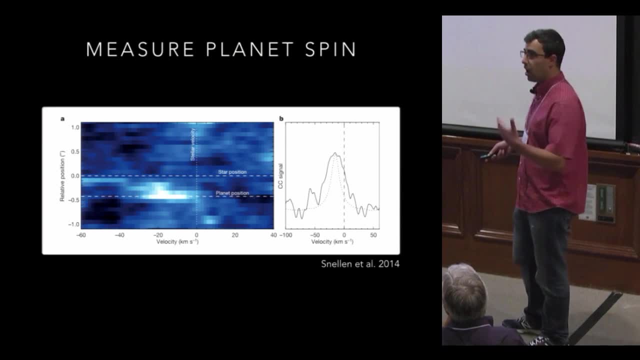 There are only a handful of objects that have been studied with this technique- And this is here a very famous, very nice result from Ignaz Celan- using cryo-arrays at the VAT. Cryo-arrays are over 100,000 spectrographs behind an adaptive optics system. 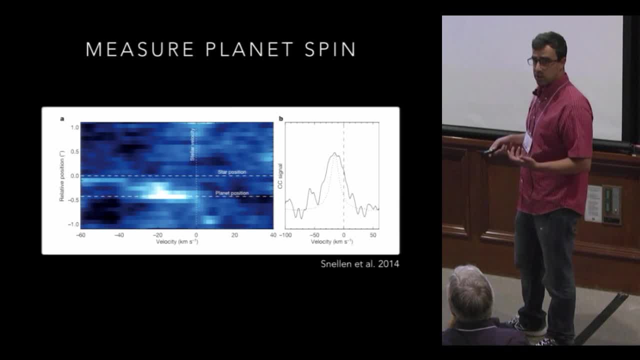 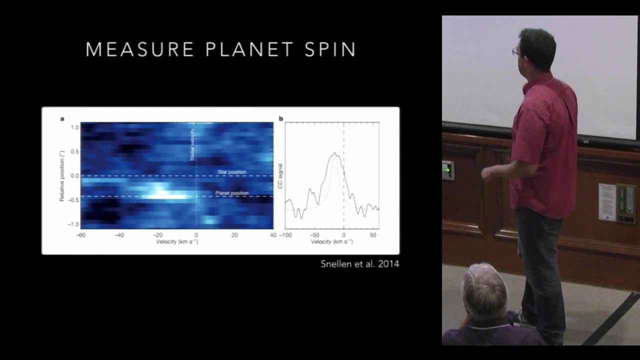 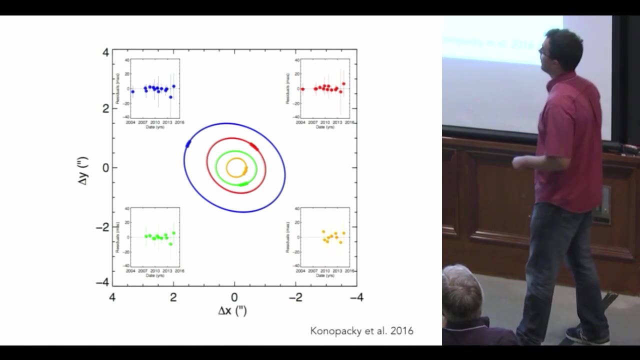 that enabled Ignaz and his team to measure directly the spin of Beta Pictoris B, which is quite awesome. So not only the spin here, but the orbital velocity. Talking about orbits, These are the currently characterized orbits of HRD 799 planets. 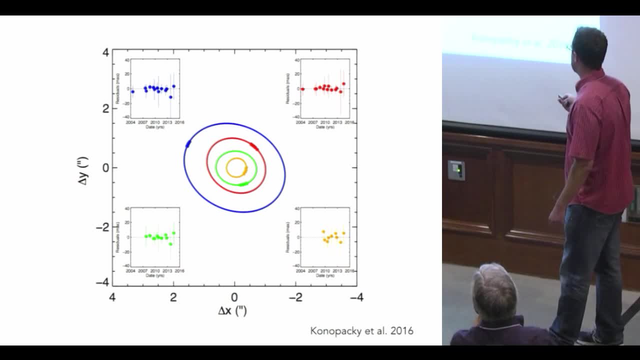 So this is the most recent paper on this object by Quinn Konopaki, using Keck NERC-II data only. So this is key here to this analysis, because using data from multiple telescopes is very challenging due to systematics that are hard to calibrate between instruments. 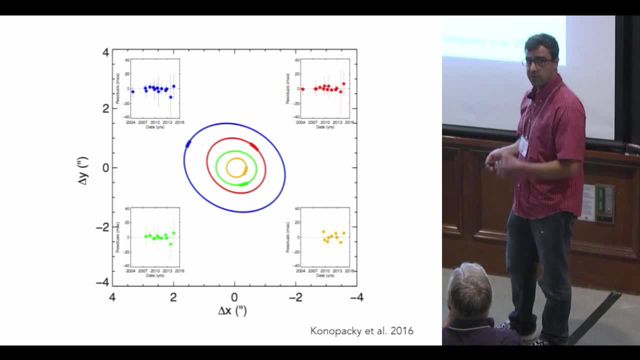 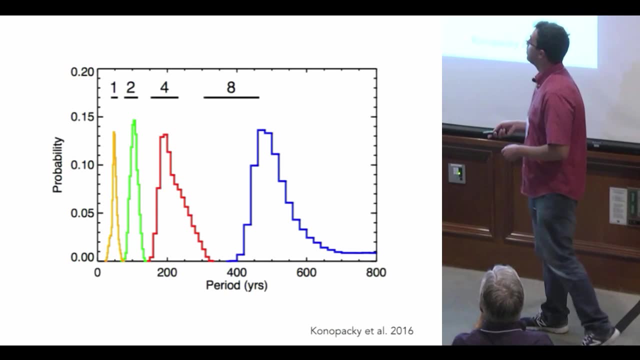 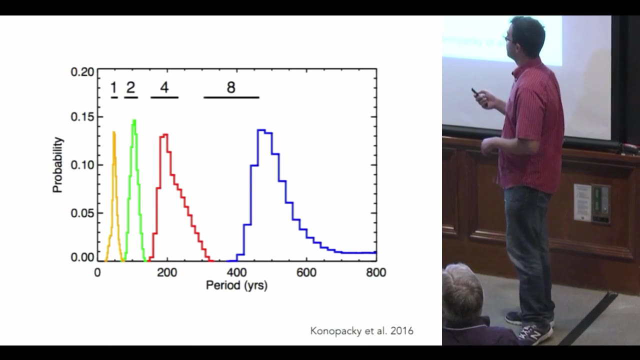 This data set is very homogeneous because Keck NERC-II is a very stable instrument. It hasn't changed in 15 years And that enabled Quinn to infer that these planets were in resonances, as can be seen in this plot, with very high confidence. 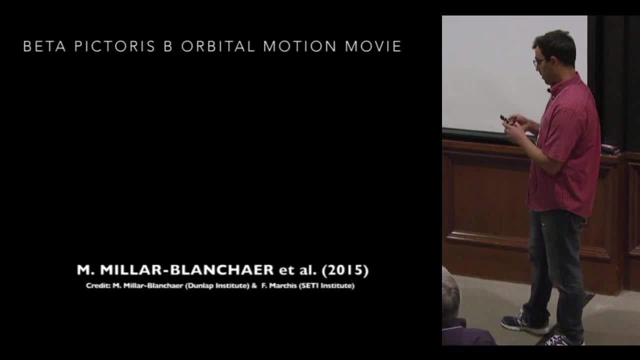 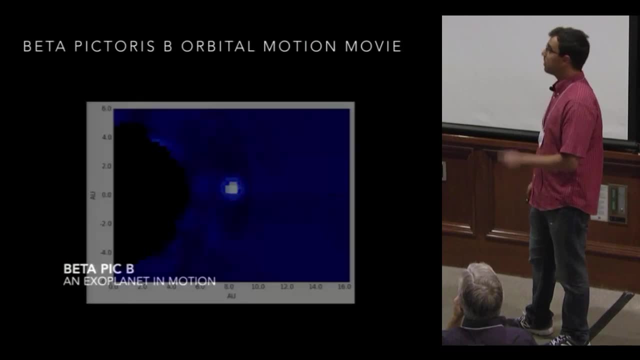 All right, so orbits. So this is a very awesome movie, I must say, made by Max Miller, Blanchard and Frank Marchis, showing the orbit of Beta Pictoris around this star as a function of time. So direct imaging allows us to directly see planets. 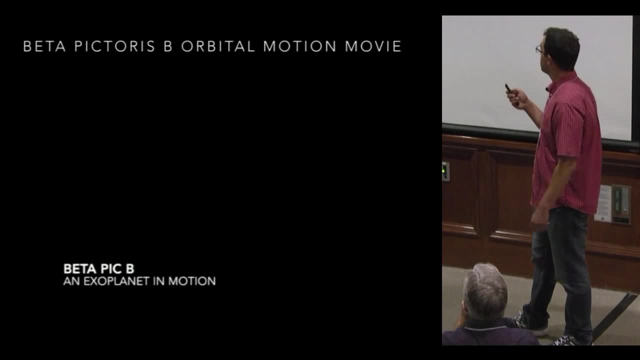 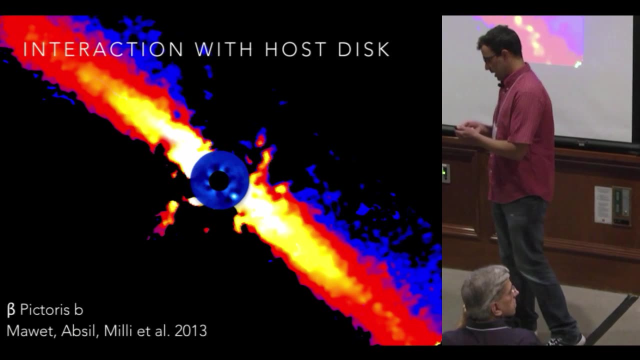 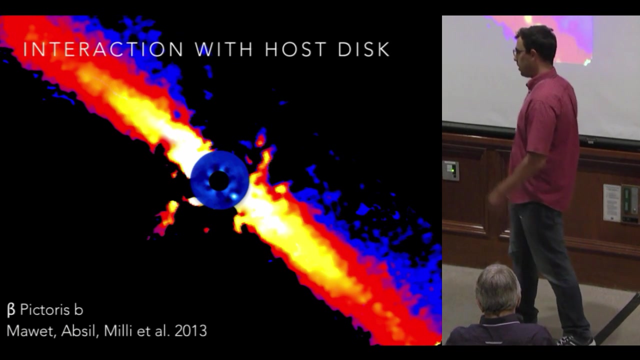 orbit around their stars, which is pretty awesome. All right, last but not least, So again focusing back on Beta Pictoris, this system. So you see the disk here that is slightly bowed here, And this bow is due to the inner disk being warped, that is seen at short wavelengths. 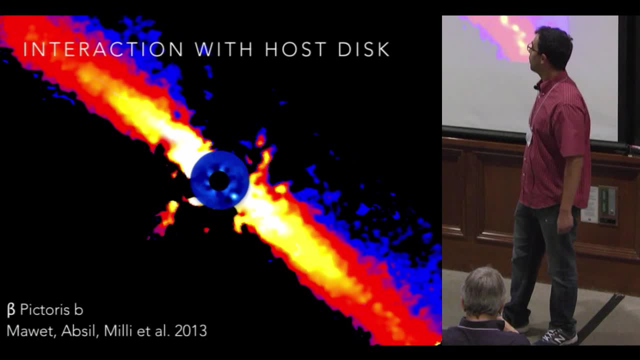 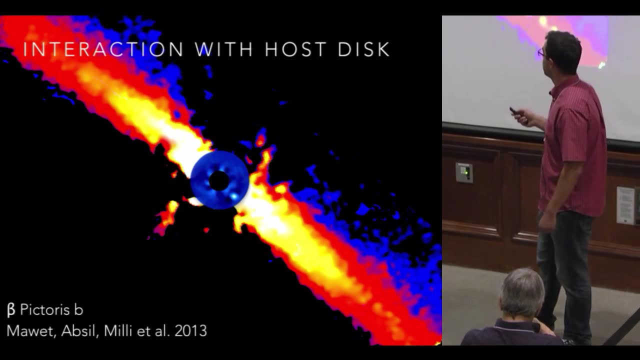 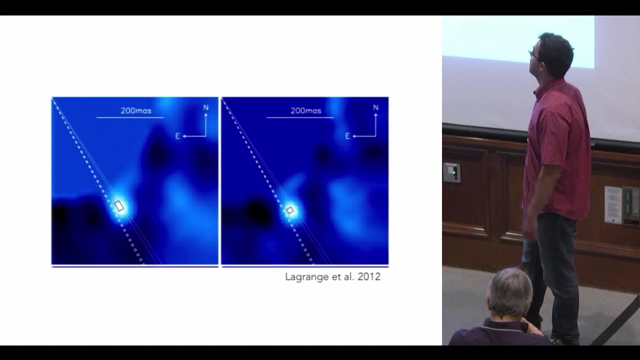 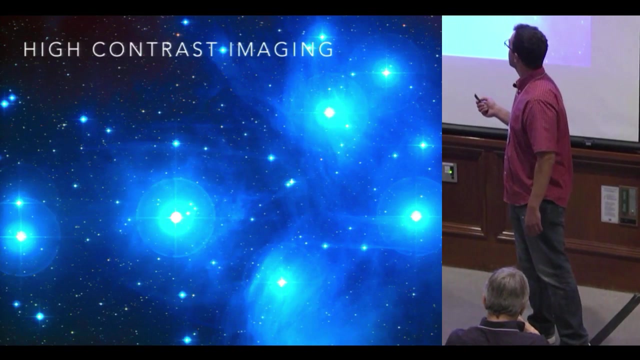 And this warp is due actually by the gravitational influence of this giant planet that is almost 10 times the mass of Jupiter. So one can measure the inclination of the orbital plane with respect to the disk and infer interactions, gravitational interactions, between the host disk and the planet that is currently steering it. 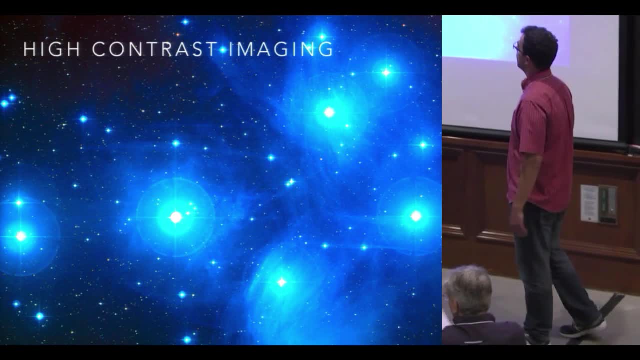 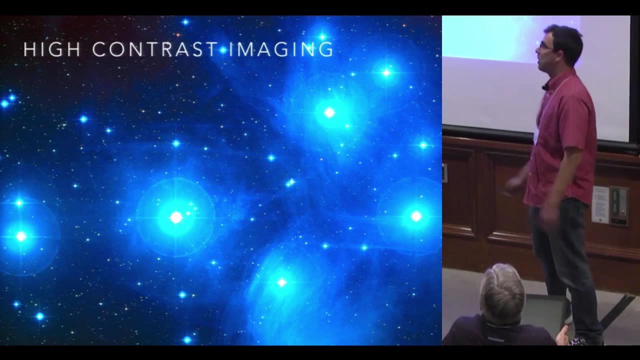 All right. so these are the results, highlights of direct imaging. And direct imaging unfortunately has not produced that many results so far, because it's hard. So I just took here a field, a very famous field. You must recognize this. 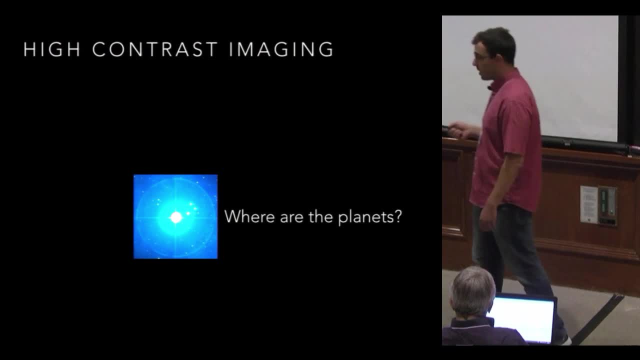 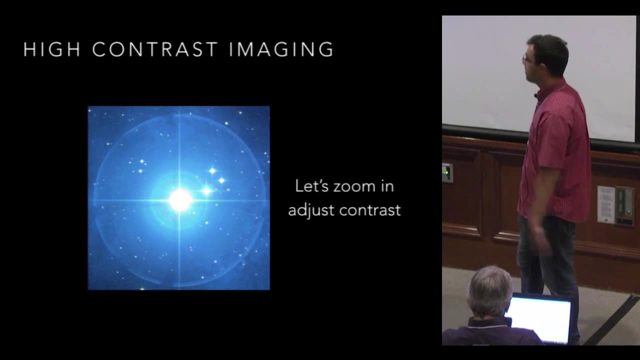 This is the Pleiades, And I just focused on one star. I'd like to know if there are planets around that star. Let's zoom in, adjust the contrast. So this is a beautiful image, a very high-quality image, perhaps one of the best we can do about the Pleiades. 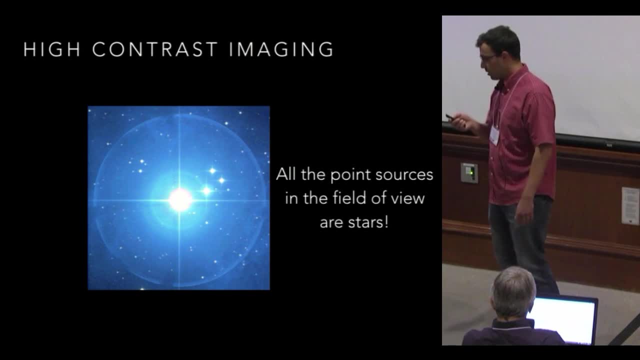 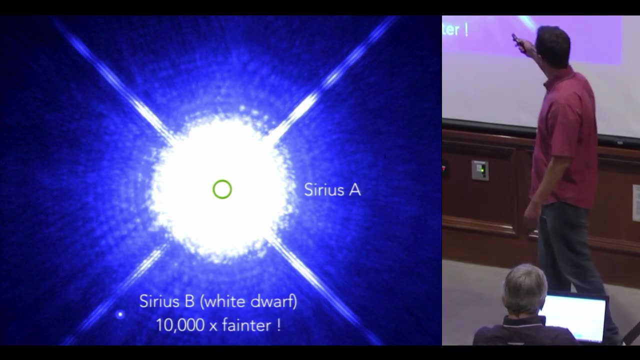 And I don't see any planets there. All the point sources in the background are stars, background stars. Problem is, stars are bright and planets are faint. This is another example here. This is Sirius A and B. Sirius B is a white dwarf that is 10,000 times fainter. 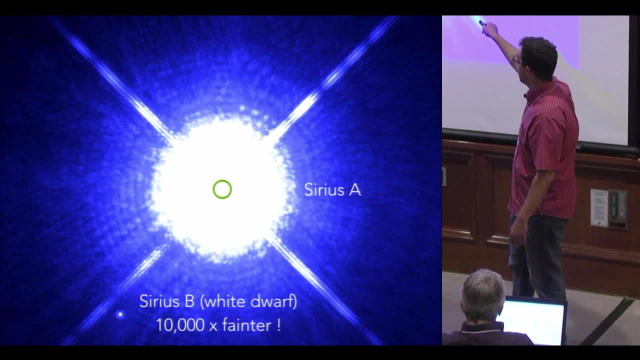 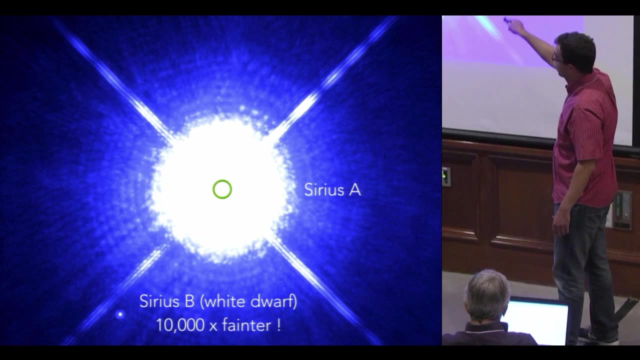 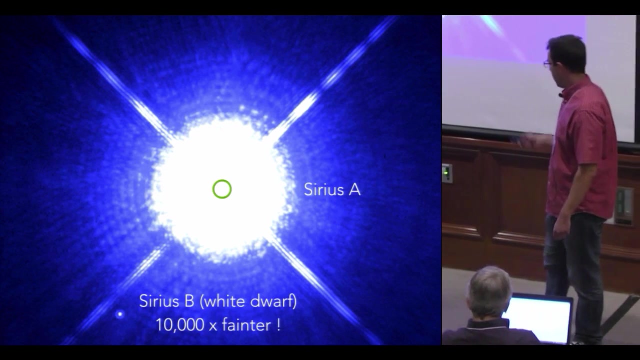 And yet it orbits at more than 50 AU from Sirius A. This is here the orbit of the Earth around the Sun as projected around Sirius A, And you see that is extremely close into the star. So imagine now taking Sirius B and putting it at 1 AU around Sirius A. 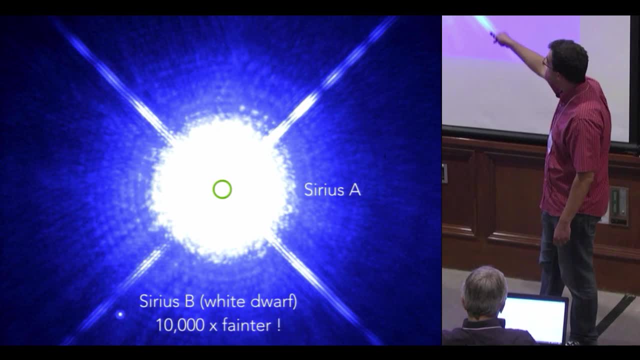 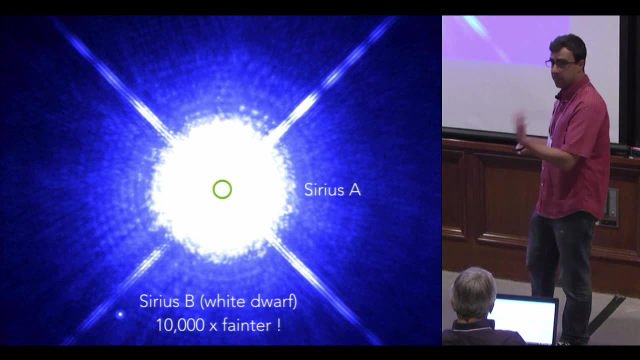 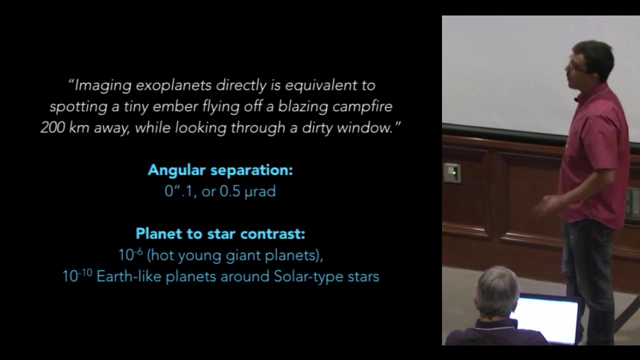 And that is indeed very, very hard to see there, because all the light from Sirius A is scattered over the image and creates this ocean of artifacts here due to diffraction and scattering that prevents us from seeing faint planets. So imaging exoplanets directly is equivalent to spotting a tiny ember. 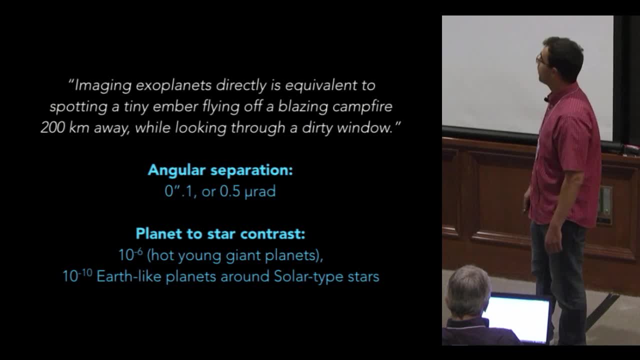 flying off a blazing campfire 200 kilometers away while looking through a dirty window. So, in more quantitative terms, the angular separations one has to deal with is a tenth of an arc, second or 0.5 micro radian. The planet-to-star contrast ranges from a few million to one. 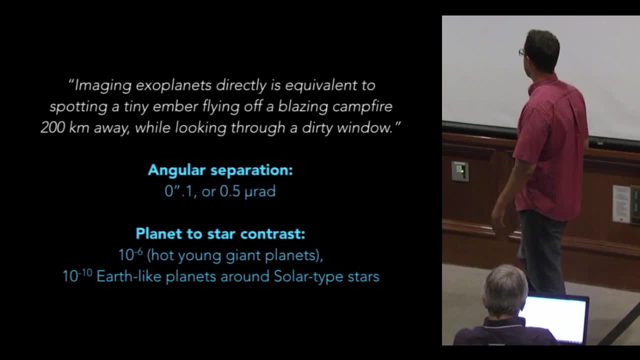 to a few billion to one in the case of Earth-like planets around solar-type stars. So remember, Sirius B is only 10,000 times fainter than Sirius A, And yet it is very hard to see if it were close to the star at these kind of separations here. 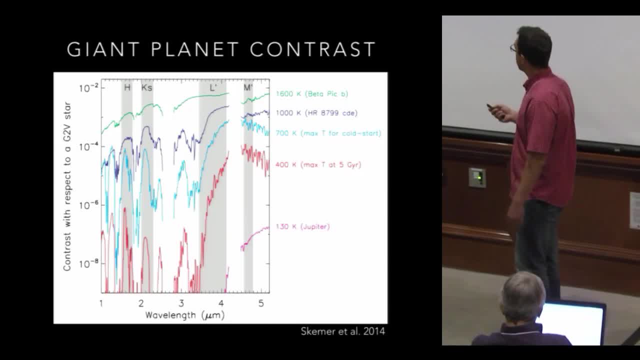 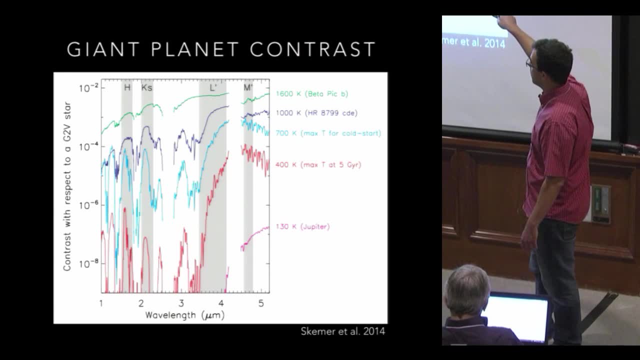 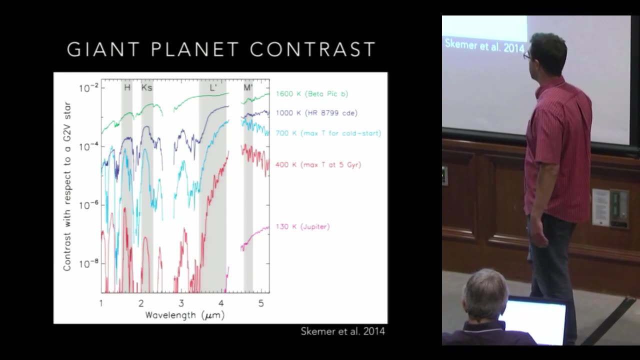 But planets are orders of magnitude fainter than Sirius B. So for giant planets the contrast range from, as I said, a few million to one, In some cases that are favorable, like young hot exoplanets, the ones we've imaged so far. 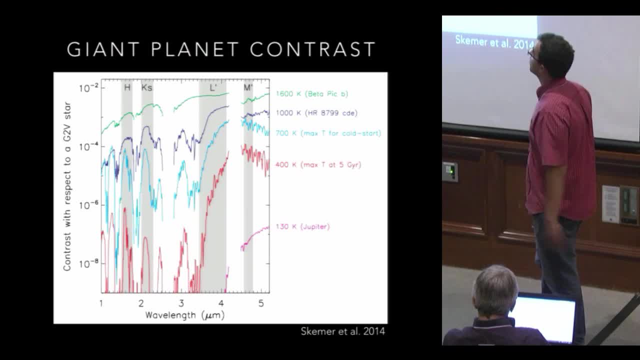 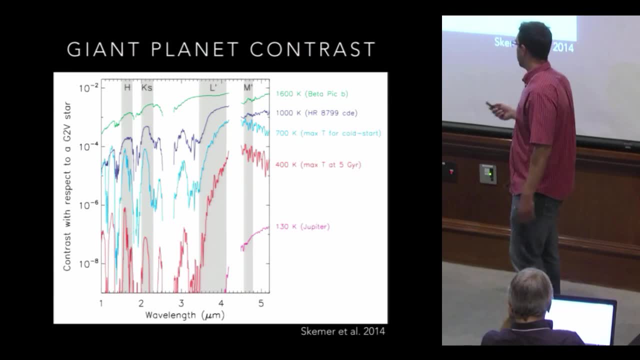 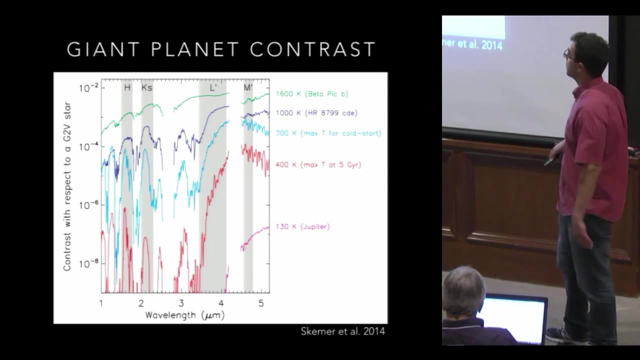 the contrast ratio is relaxed to maybe a few thousandths to one, So Jupiter here in this corner it's typically a few billion to one contrast ratio. So you see in this scale here that the reason why we've only imaged very young exoplanets so far. 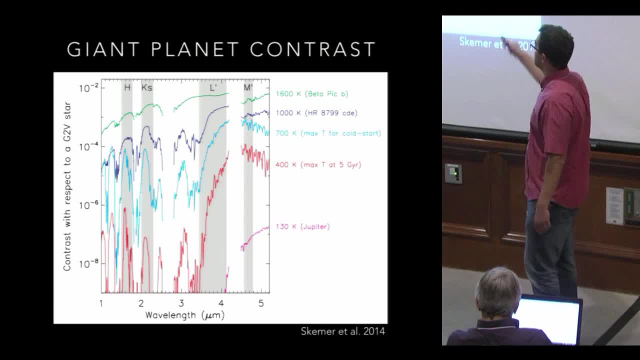 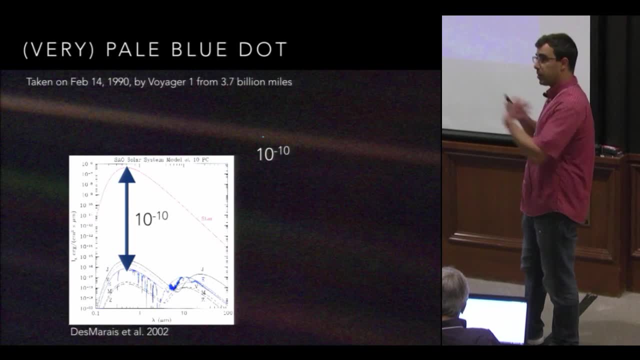 They are indeed much brighter because they are hot and their blackbody emission peaks in the infrared, So in the visible it's much, much harder. So one looks at the reflected light of the exoplanet and the contrast ratios here are extremely challenging. 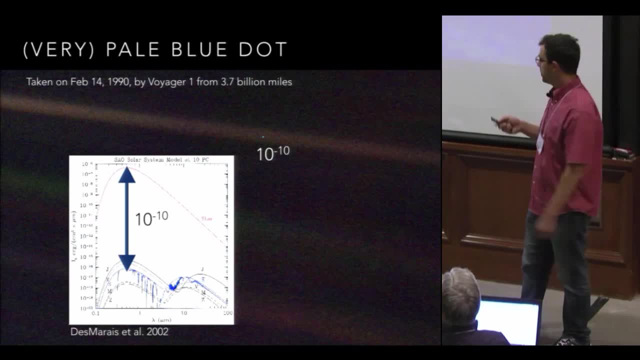 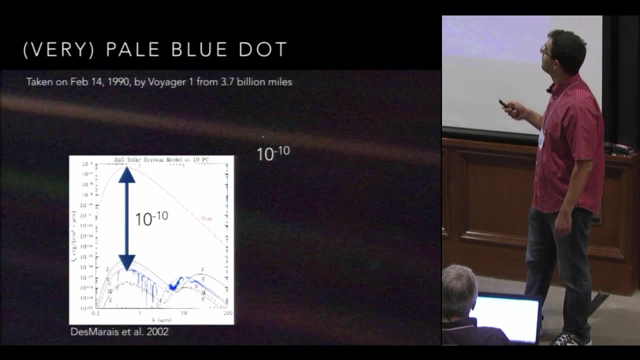 And that is the reason why we are working so hard to develop the technologies that are, in the future, going to enable us to image these very, very faint, very, very faint exoplanets. Okay, so here I'm going to go over the four pillars of high contrast imaging. 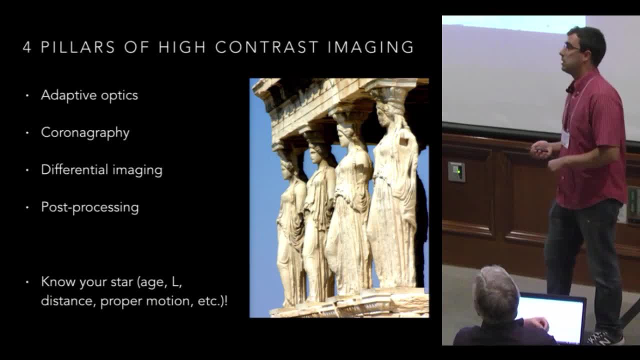 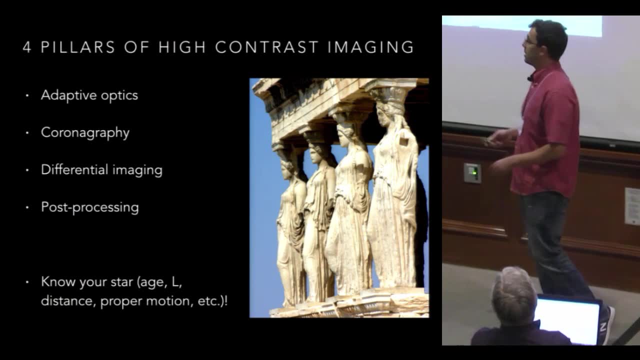 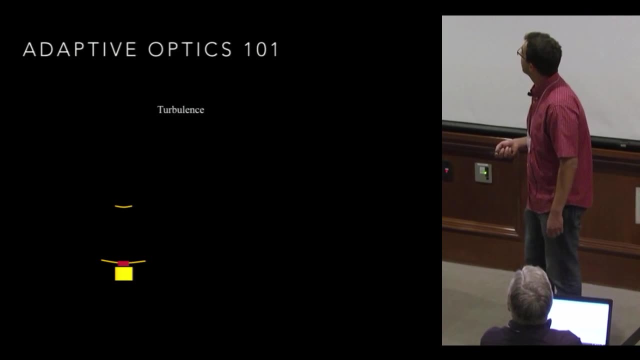 And these are applicable to ground-based high contrast imagers and space-based imagers as well. So all these ingredients are in some ways adapted to the specific platform one has to observe with. So let's start with adaptive optics. So quickly, adaptive optics 101 here. 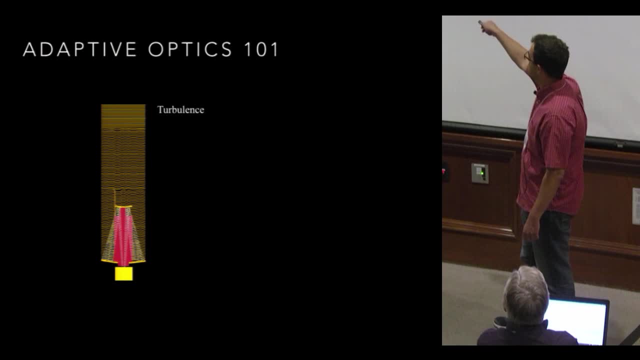 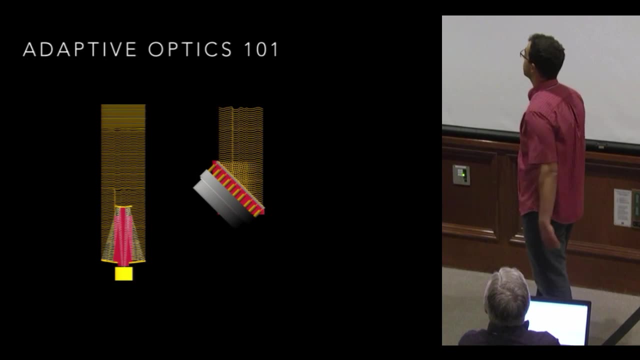 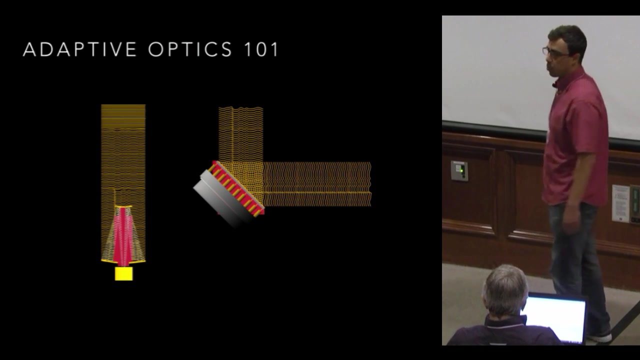 So this is a ground-based telescope. Okay, so this is the 90 or 100 kilometers of atmosphere that disturb the wavefront of the starlight propagating through it. So you see, here the flat wavefronts in space are disturbed, corrugated by propagation. 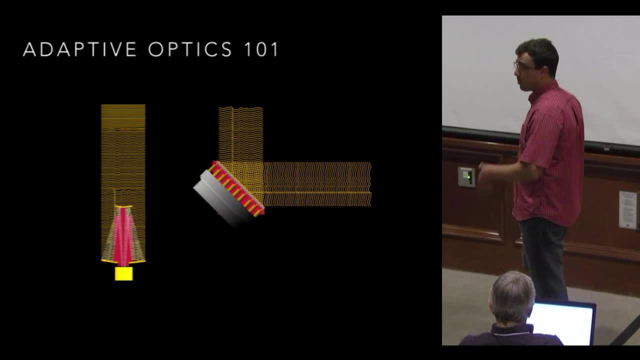 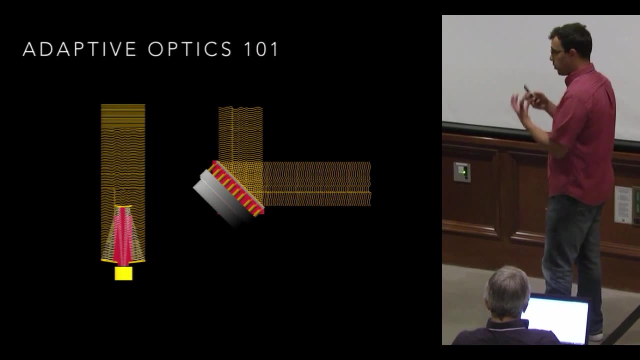 through the turbulent atmosphere They enter the telescope. they pick up more aberrations as they propagate through the telescope optics. So in adaptive optics one uses a small mirror. It's a small mirror. We don't use the primary mirror to do that. 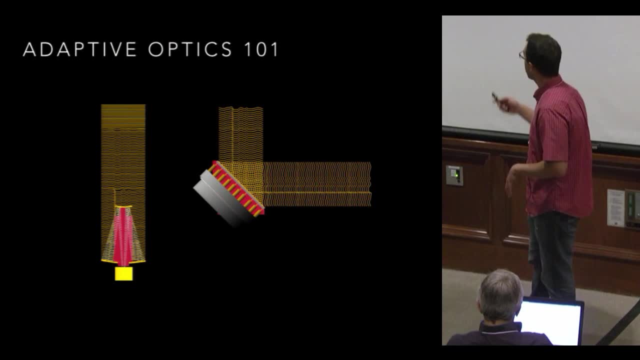 We use a small mirror- It's perhaps a few inches in diameter- that is equipped with actuators at the back that push against a face sheet that is the reflective surface of the mirror. So there are typically from a few hundred to a few thousand actuators. 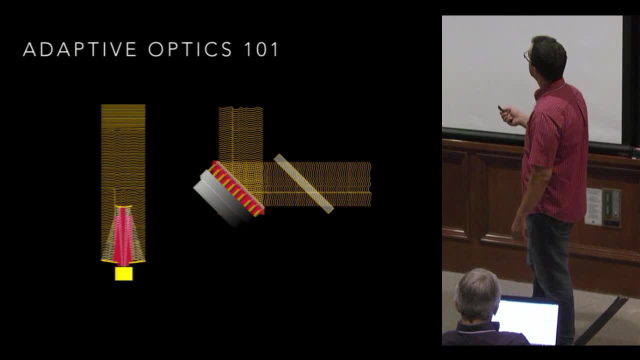 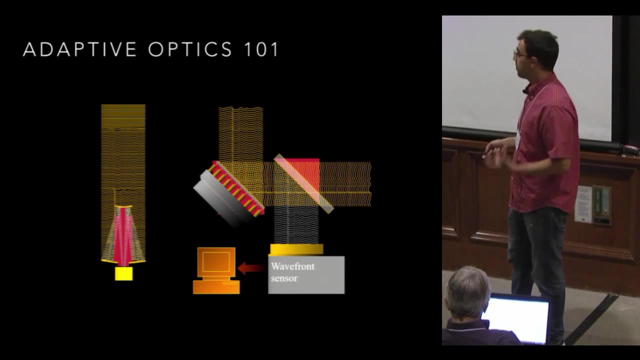 behind the surface of this small mirror. So the mirror doesn't know what to do, so we have to measure the disturbance, so the corrugation of the wavefront, using a device called a wavefront sensor. There are many kinds of wavefront sensors. 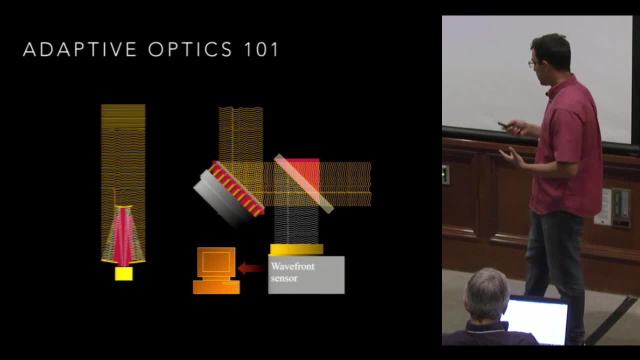 but the goal is always the same: to measure these disturbances as fast as possible. So the wavefront sensor feeds back its measurement to a computer that is going to send the commands to the deformable mirror so that it will make the wavefront flat again. 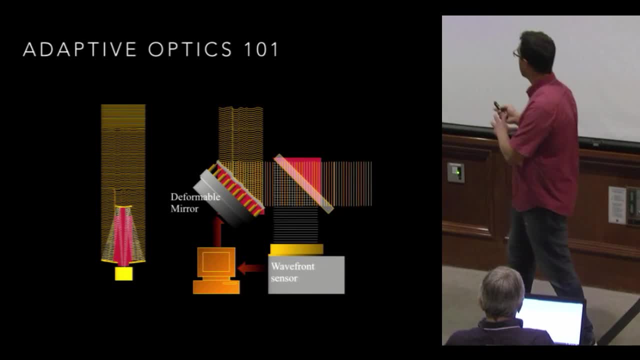 And this is how most adaptive optics systems work. So they measure corrugation of wavefronts in real time and feed back these measurements to a small deformable mirror that one tries to actuate as fast as possible. How fast is that So for ground-based telescopes? 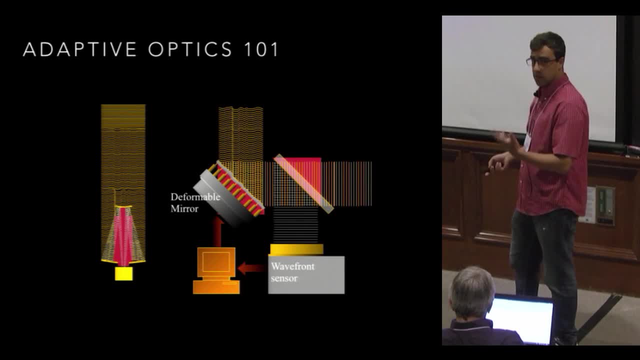 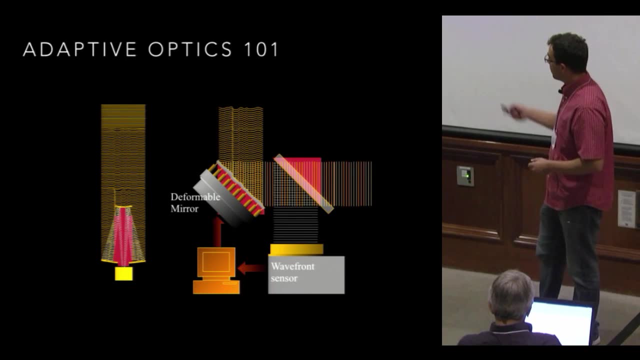 typically that's one kilohertz, So the mirror surface here is refreshed a thousand times per second. In space, of course, there is no atmosphere, there is no turbulence, and one has to deal only with the aberrations in the optical train. 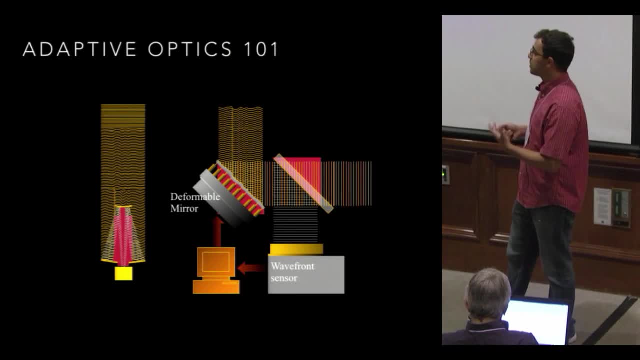 and so the refresh rate can be much, much slower. Space telescopes sometimes don't point very well, and so that entices us to go to faster speeds as well. That is the case for WFIRST. So the dramatic effect of adaptive optics. 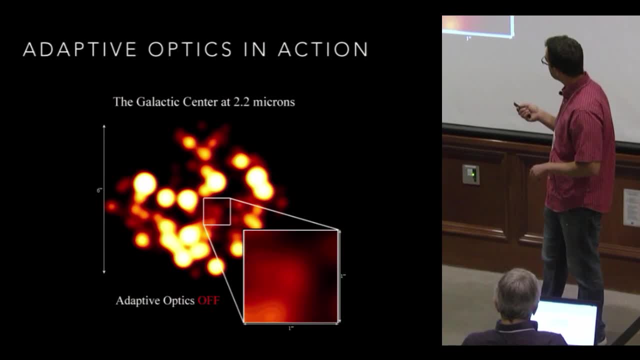 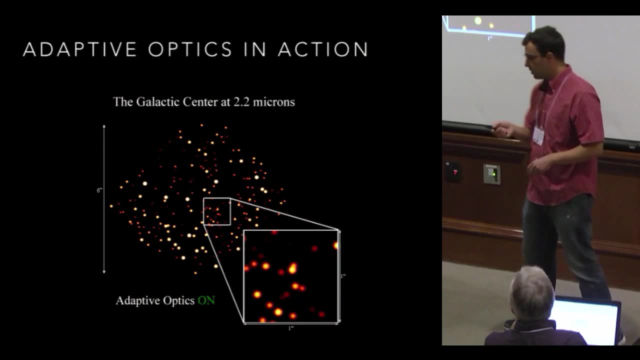 can best be seen in this image. I think This is an image of the galactic center, and this is without the adaptive optics system. Now I'm going to turn the adaptive optics system on and see that it recovers the diffraction limit. 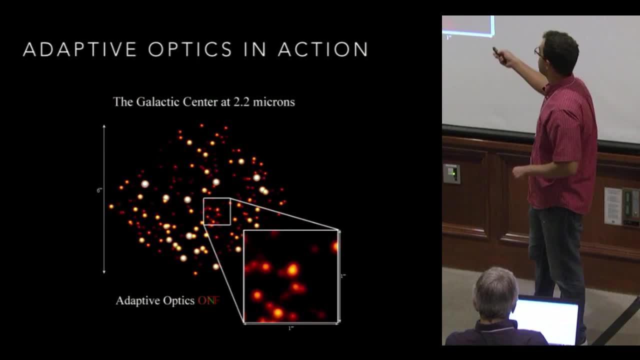 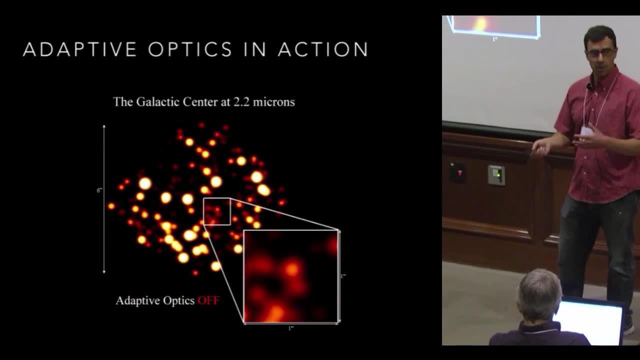 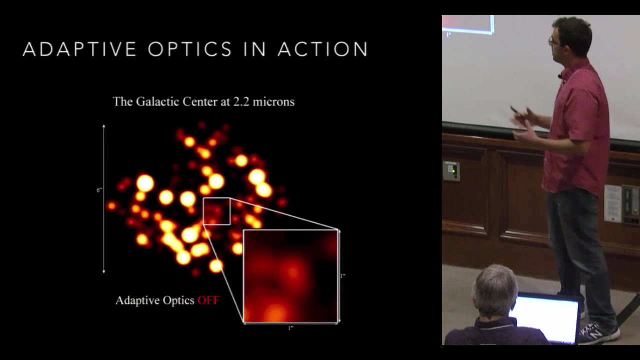 of, in that case, the Keck telescope. So the effect of adaptive optics is amazing on the quality of images that are provided by ground-based telescopes. One goes from seeing limited images that have very poor resolution, no better than a 20-centimeter telescope. 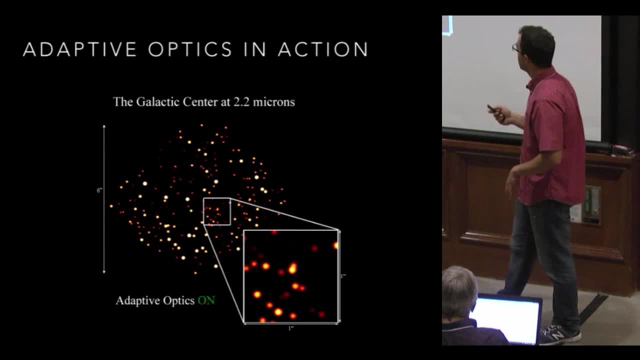 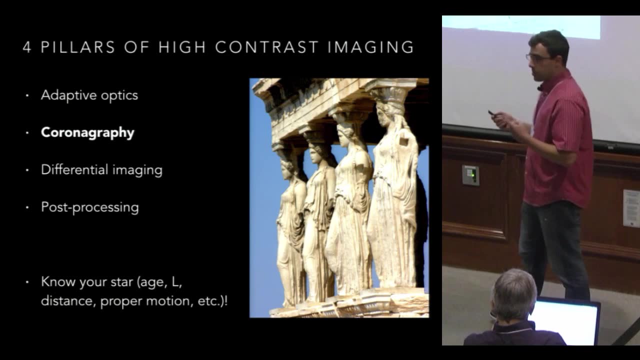 to the full diffraction power of a 10-meter telescope, So this works extremely well. It has been used successfully for more than 20 years. This is ingredient number one for direct imaging. The second one is called chronography, So chronography is very simple. 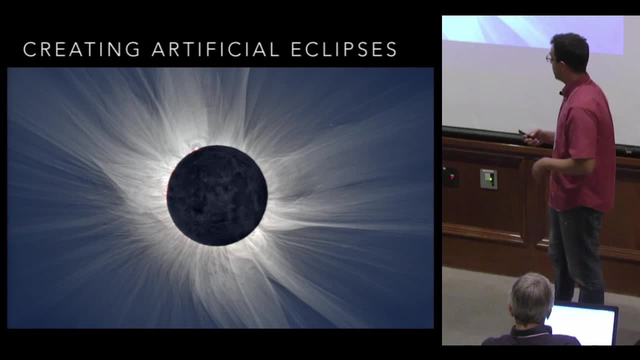 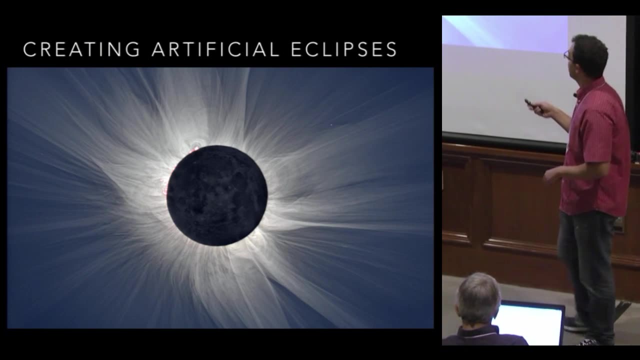 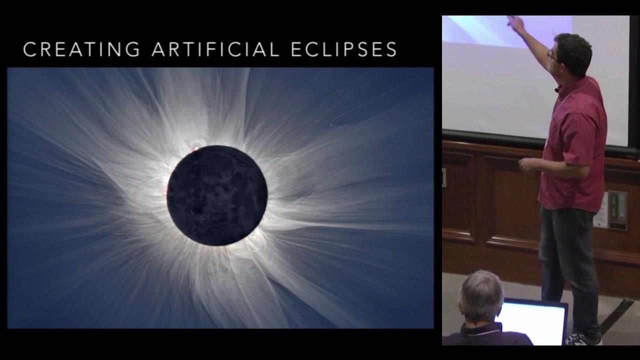 This is a way to enhance contrast in images when the bright object is present. So the best chronograph maybe is the moon. So this is a picture of the solar corona during a total eclipse of the moon, And you see here how striking this image can be. 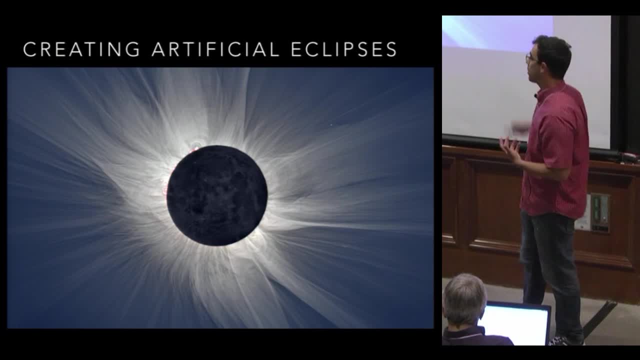 You have to know that the solar corona is about 10 million times fainter than the photosphere of the sun, So the moon is indeed a very, very powerful corona. Unfortunately, it's not very efficient nor easy to steer around. 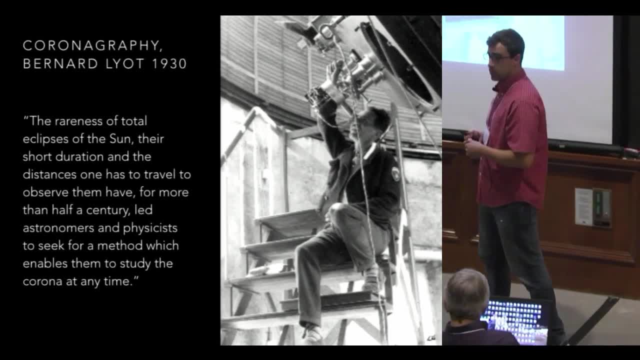 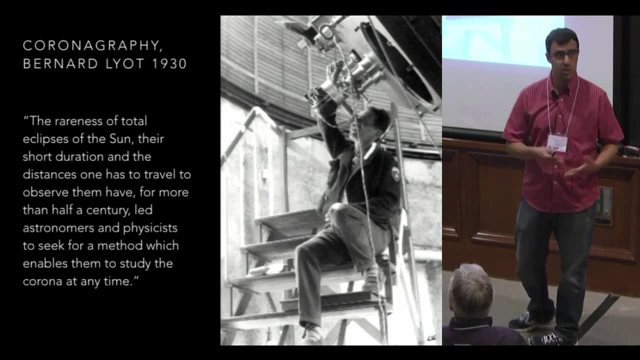 And that is the reason why Bernard Leo, a French astronomer, invented this device called the chronograph. So the name comes from the first application of chronography, which was to image the solar corona. And so astronomers at the beginning of the last century. 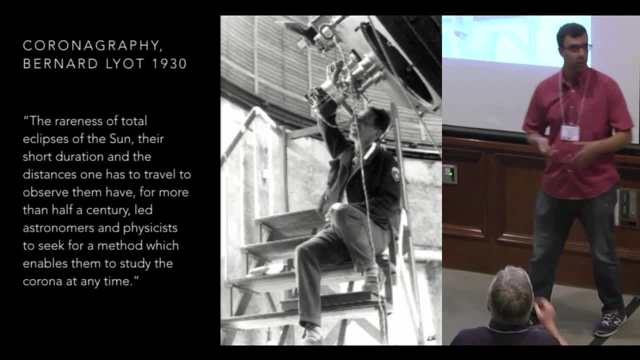 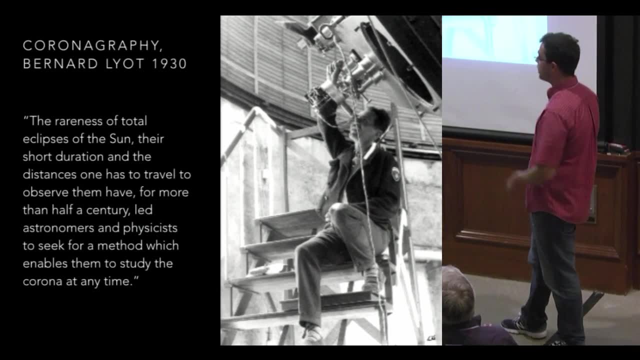 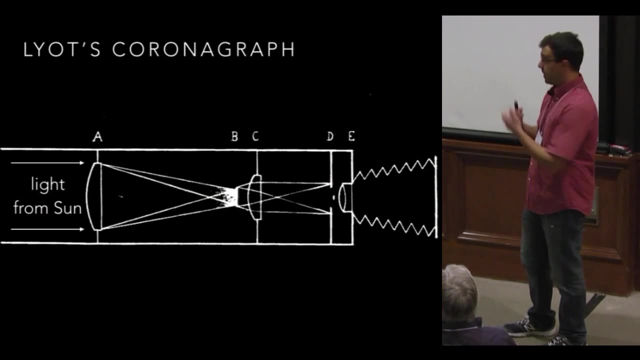 were extremely tired of traveling around the world. Apparently, it's not the case anymore, And so Bernard Leo invented a chronograph to allow him to study his preferred astrophysical object at any time. So this is a schematic made by Bernard Leo himself. 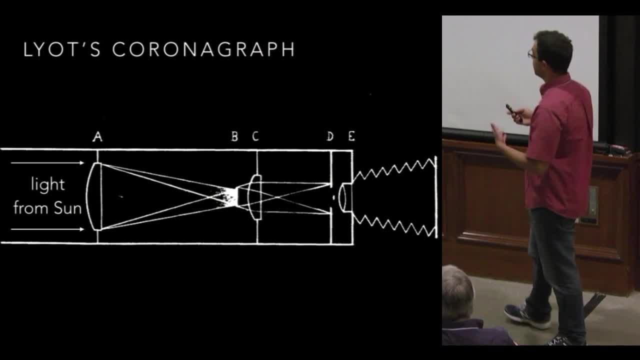 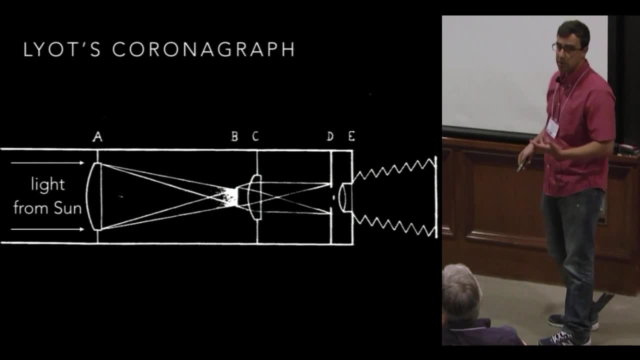 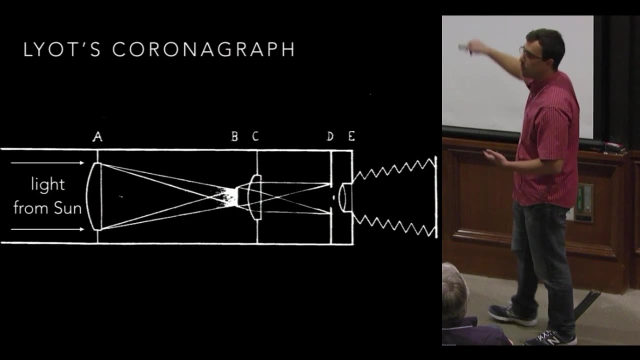 so in the 1930s, showing a telescope and its modification to image the solar corona. So light from the sun enters the telescope. This is here the entrance pupil of the telescope, so where the focusing lens sits. So this could be the primary mirror. 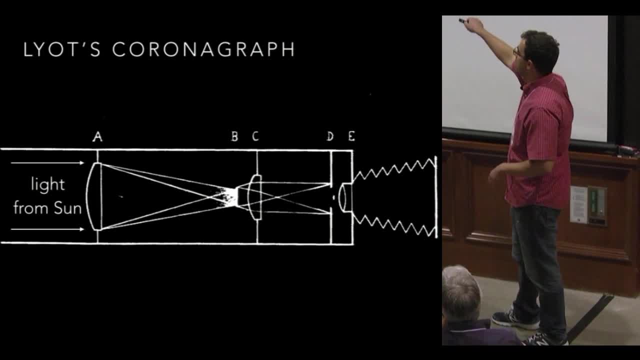 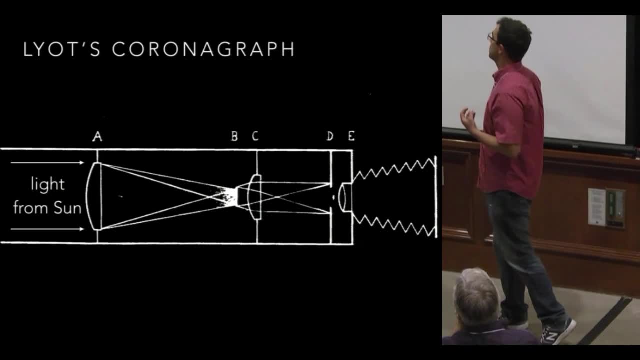 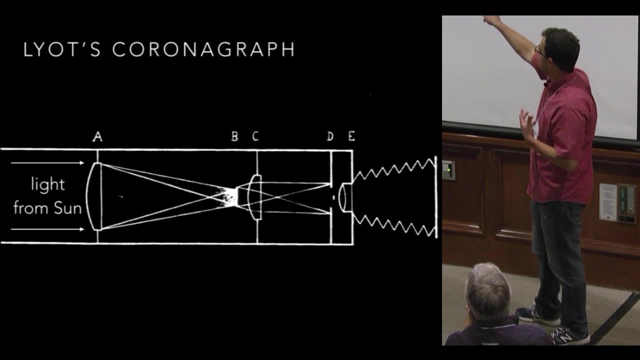 of a modern telescope. So this mirror or lens here focuses the light of the photosphere of the sun onto a blocking mask which is the apparent size, apparently size- of the sun, And so all the light from the photosphere is blocked by this mask. 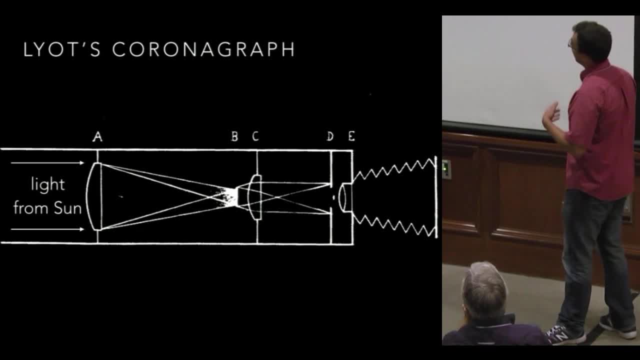 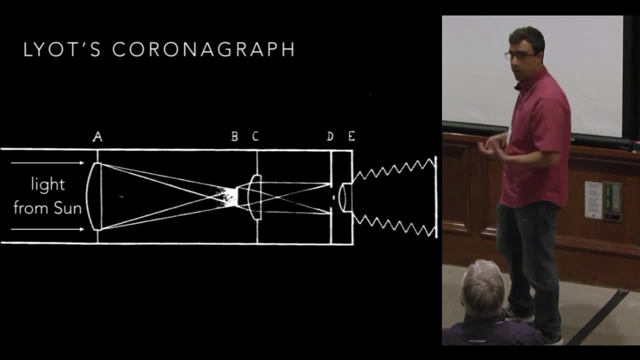 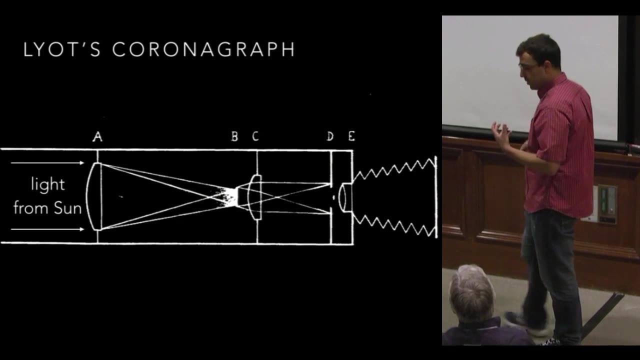 People have tried to do that for many years and quite unsuccessfully, the reason being diffraction. So diffraction around the mask here, due to the wave nature of light propagation, makes some light spill over the mask, And so the trick here and the genius contribution. 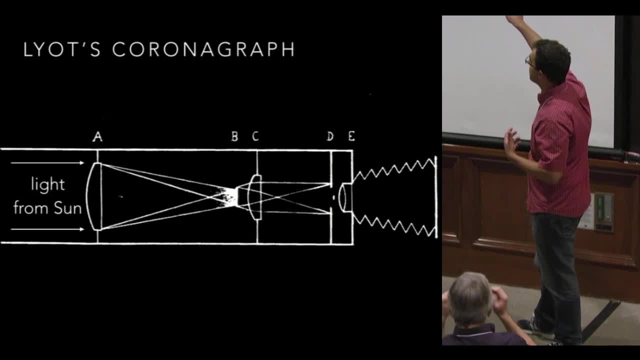 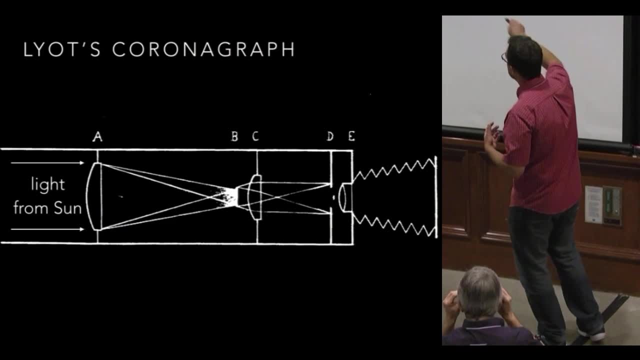 of Bernard Leo was to put a field lens C and a diaphragm in the pupil plane. That is an image of this plane here. So the key contribution of Bernard Leo is these elements C and D, So these additional optics in the system. 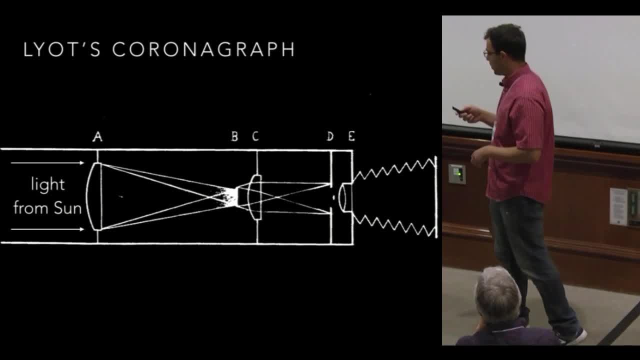 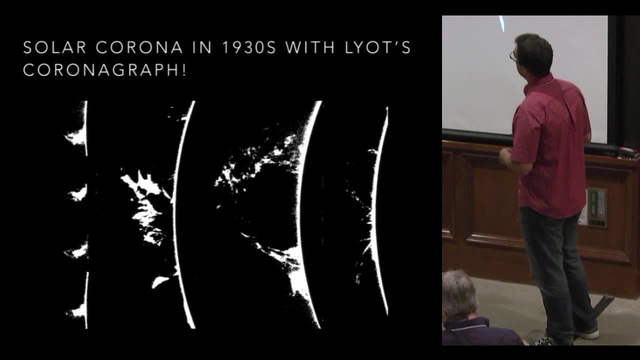 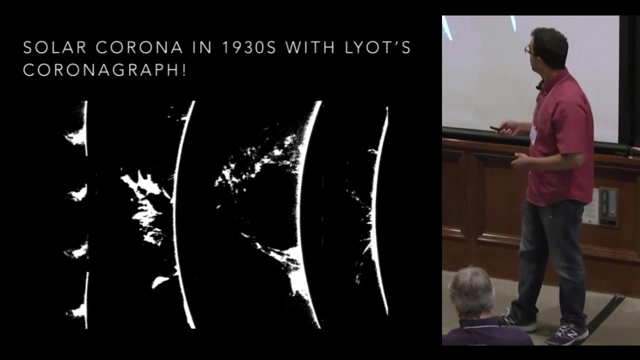 which made diffraction control much more manageable. And Bernard Leo, with this device called a coronagraph, made these amazing pictures of coronal mass ejections in the 30s And he could study them with spectrographs, with polarimeters. So this was a key contribution of Bernard Leo. 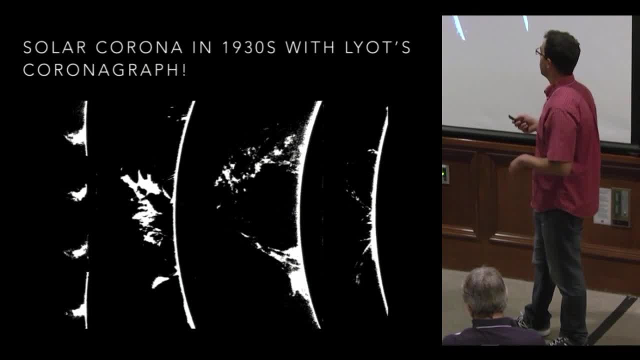 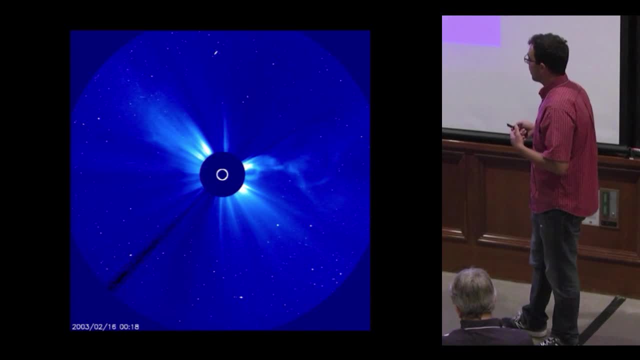 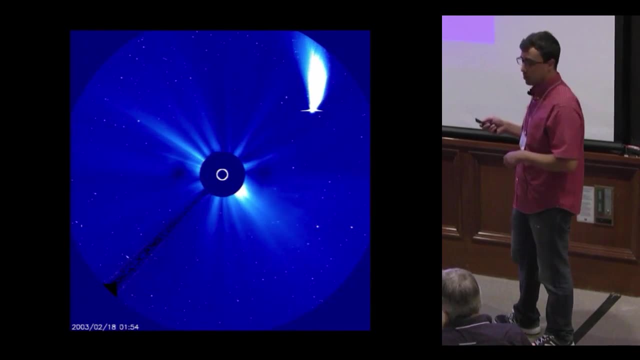 to solar astrophysics and modern eye contrast imaging exoplanets. So Leo coronagraphs are used 24-7.. This is a movie from the SOHO satellite that is monitoring the sun 24-7. And that is equipped with a Leo coronagraph here. 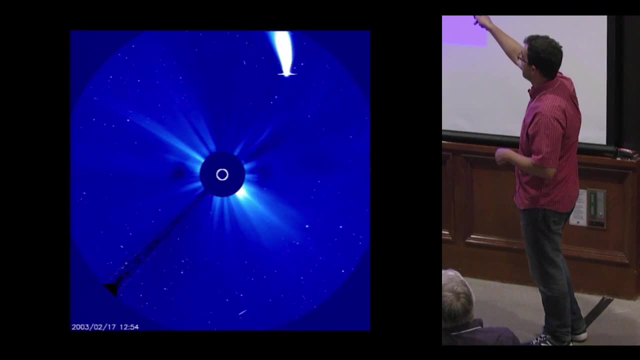 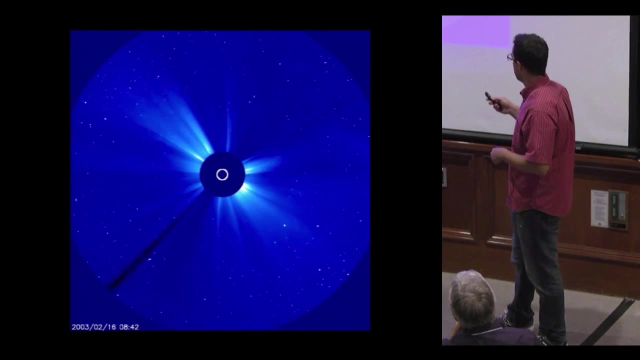 So the angular size of the Leo coronagraph is roughly this big mask here And the sun's photosphere is here noted by this white circle. So you see, the coronagraph is extremely powerful. One can even see the background stars in this image. 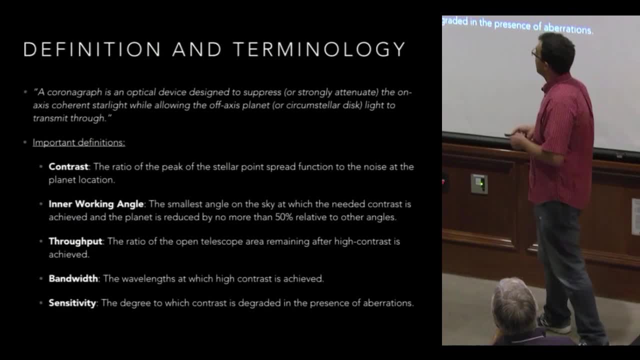 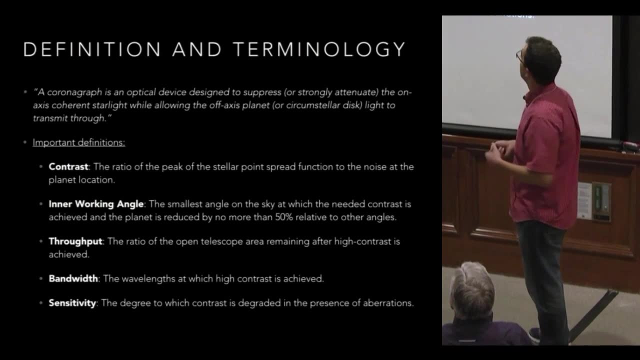 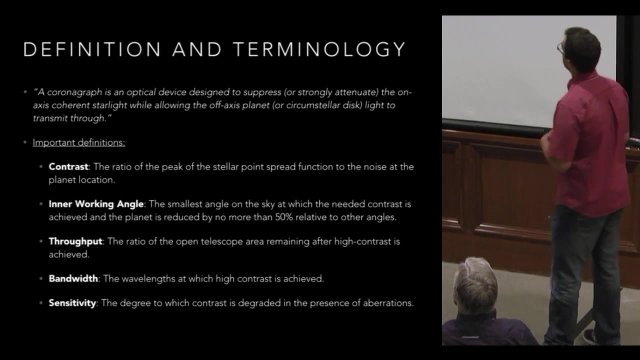 and the comet fly by. OK, so this is the modern definitions of coronagraphs. So coronagraph is an optical device designed to suppress or strongly attenuate the on-axis coherent starlight, while allowing the off-axis planet or circumstellar disk or coronal features. 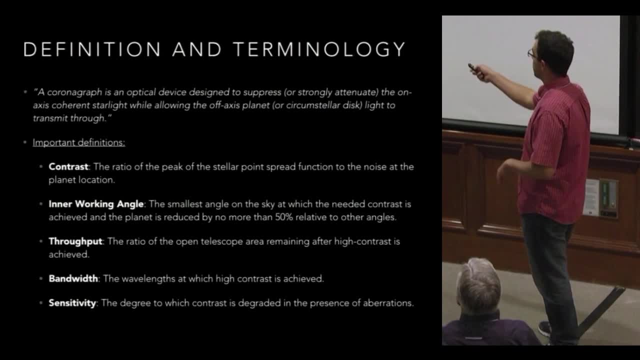 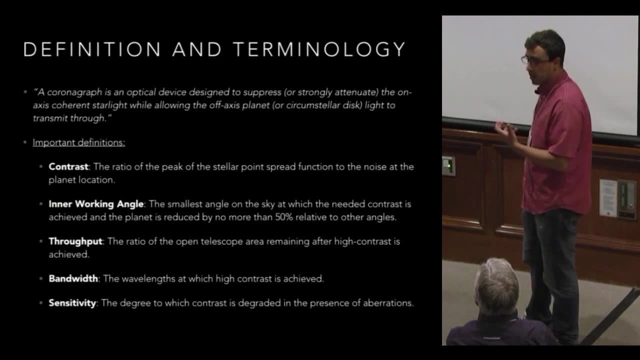 to transmit through. So the contrast definition is the ratio of the peak of the stellar point spread function to the noise at the planet location. The working angle is a key term in coronagraphy. That is the smallest angle on the sky at which the needed contrast is achieved. 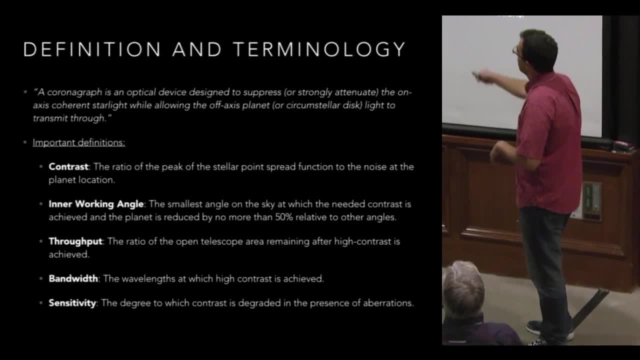 and the planet is reduced by no more than 50%. Throughput is the ratio of the open telescope area remaining after high contrast is achieved. Bandwidth is the wavelength at which high contrast is achieved. Sensitivity is the degree to which contrast is degraded. 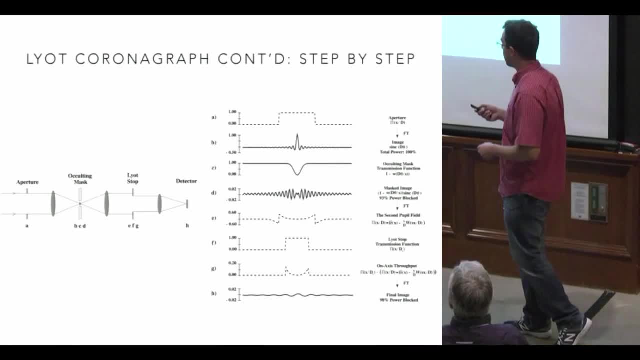 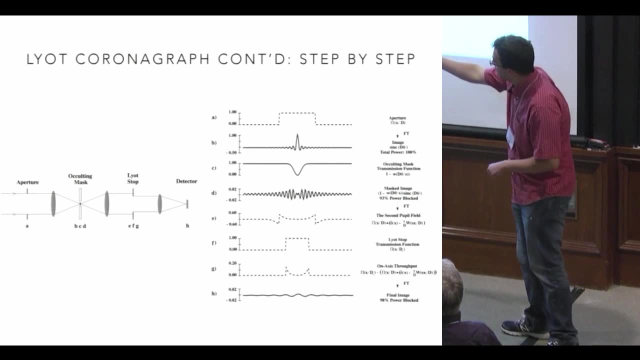 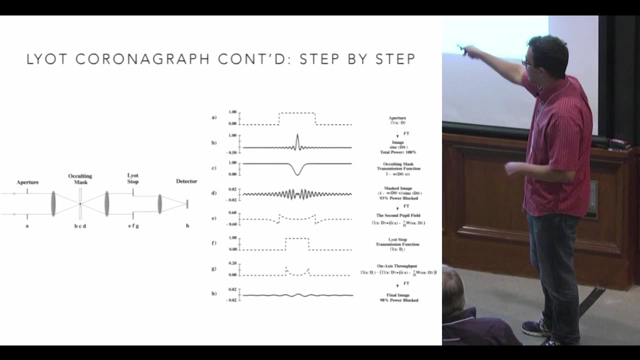 in the presence of aberration, And that subject will be covered by Laurent in detail. This is here a flow chart of coronagraphy. So you recognize here this three-plane design from Bern or Leo, And one goes from a pupil plane to an image plane by means of a Fourier transform. 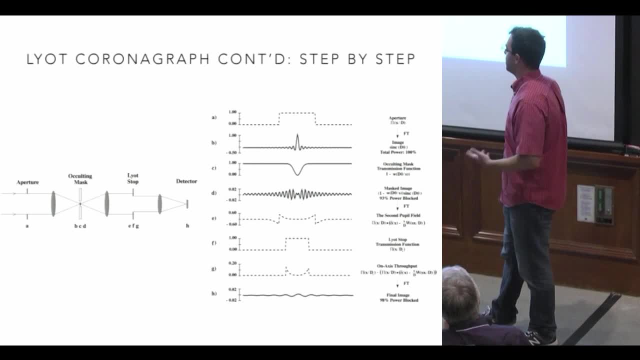 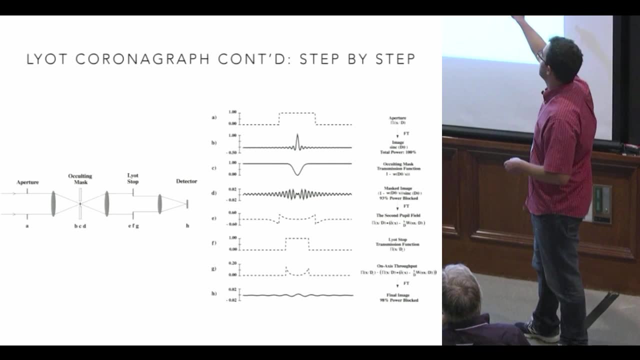 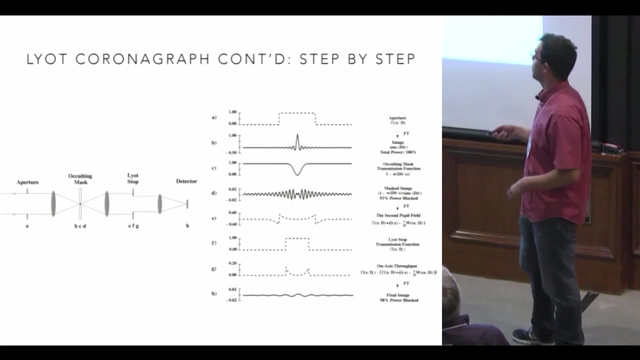 So this is applying Fourier optics here at phase value. So one cannot do coronagraphy without Fourier optics. So the entrance aperture is this flat-top function. So the Fourier transform of a flat-top function is a sinc function. So basically this is what we call a Nary function. 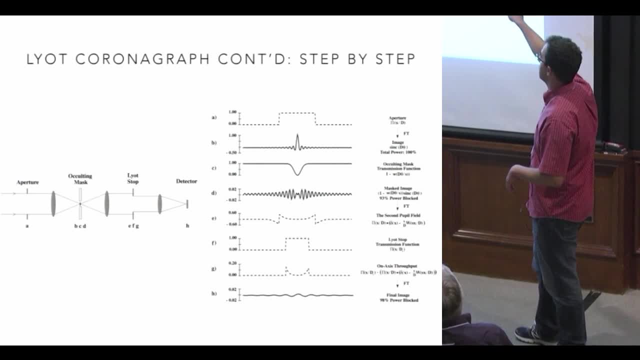 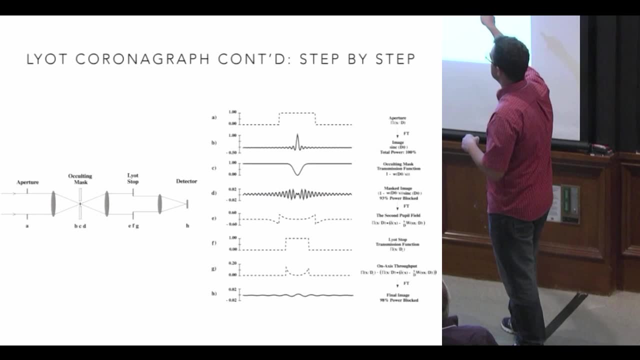 The mass transmission. here the occulting mass is a Gaussian in that case. So multiplying the Gaussian by the point spread function of the telescope here yields this function. You see, the central peak has been attenuated by the coronagraph. Another Fourier transform allows us to go. 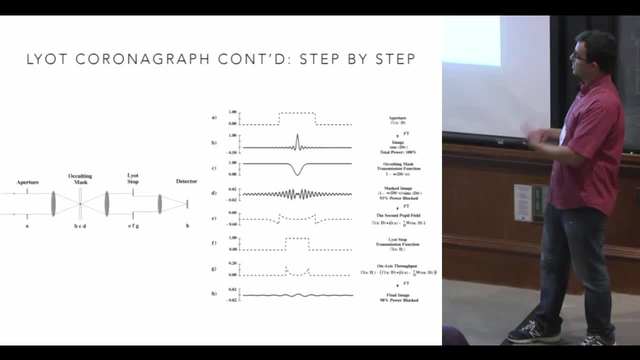 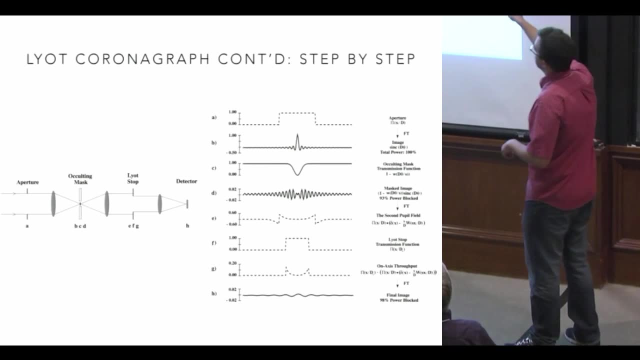 in this plane that is called the Leo plane because that is the contribution of Bern or Leo to reimage the entrance aperture to another plane called the Leo plane. So the Fourier transform of this product of the mass transmission function by the point spread function yields this function in the Leo plane. 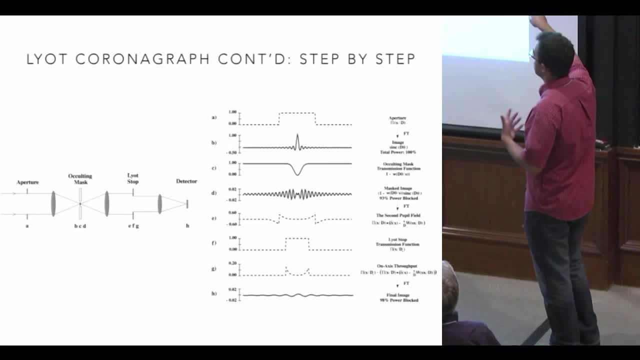 You see that most of the light is gone If you compare it to the entrance aperture. most of the light is gone here, but there is some diffraction residuals around the edges of the pupil. So a Leo stop is just this transmissive diaphragm. 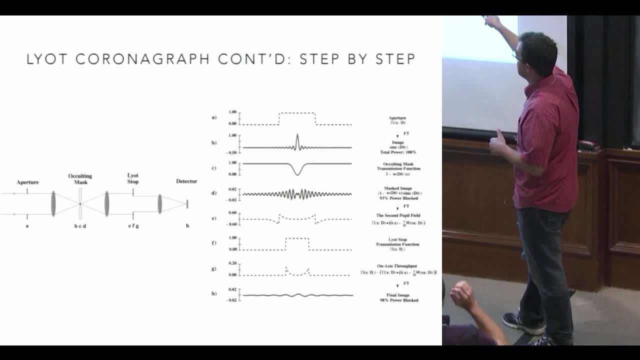 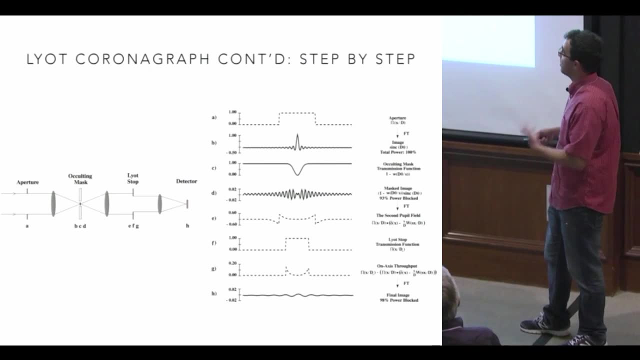 that we place there, that cuts off these edges here. So after the Leo stop, here we are left with these residuals due to diffraction, And these residuals here create this final image at a much smaller, with much less light. So you see, here the scale is about 2%. 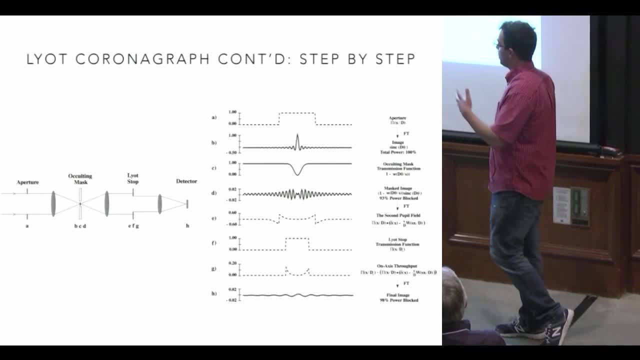 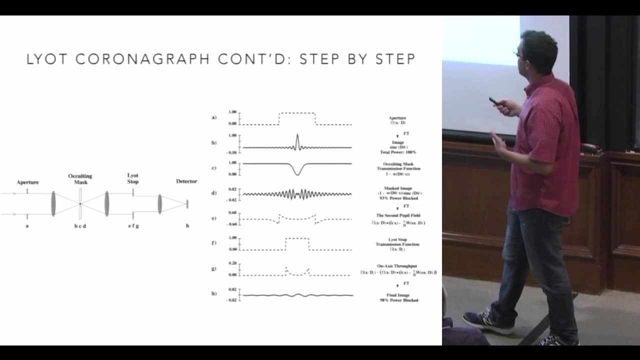 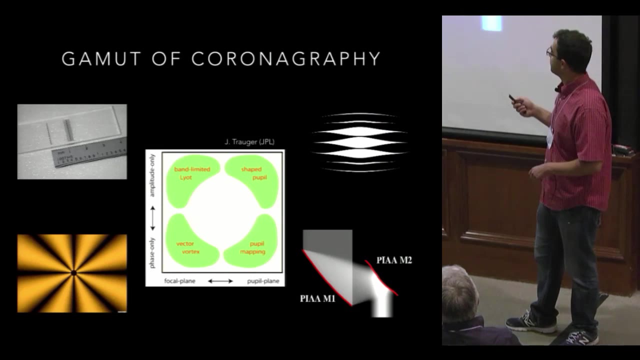 of the initial scale. So more than 98% of the light has been suppressed by the coronagraph. This is not a perfect coronagraph, of course, and there are many ways to many functions one can put there to improve coronagraph performances. 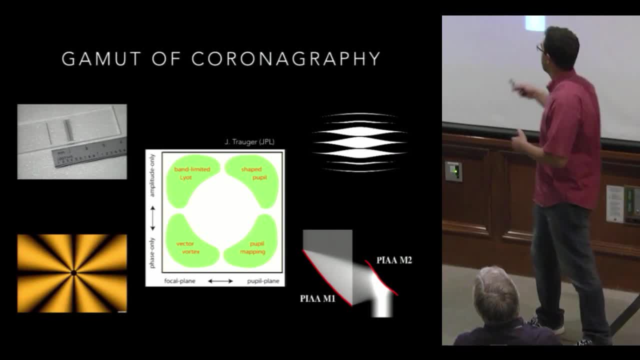 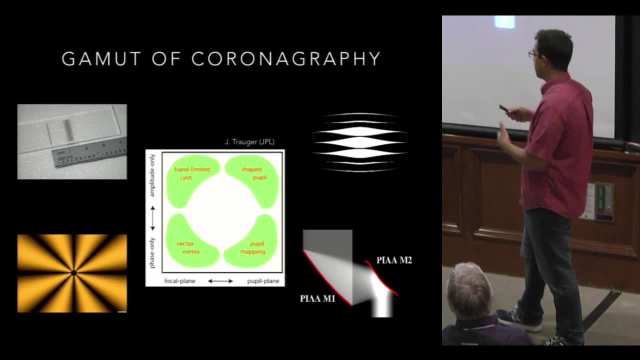 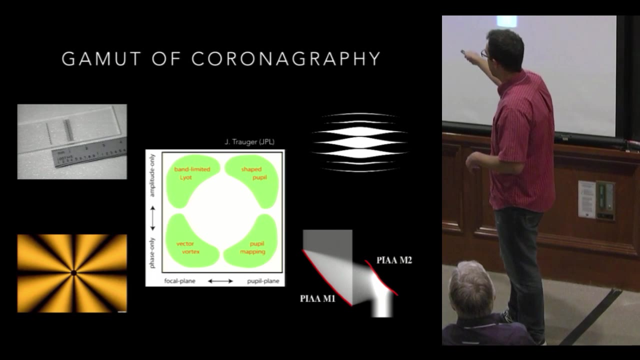 So this is the modern gamut of coronagraphy. So it is divided in this 2D space between the way we act on the light, so either amplitude or phase, and where we act on the light, either in the focal plane or in the pupil plane. 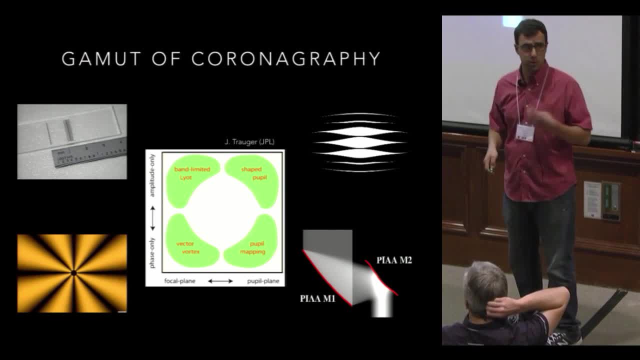 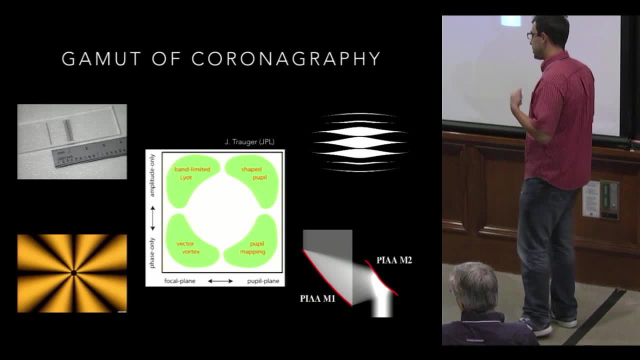 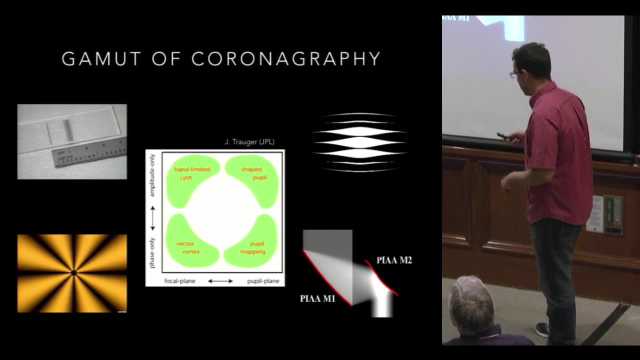 So there is basically four big families of modern coronagraphs that occupy corners of this gamut. So most recent developments actually try to hybridize coronagraphs by exploring this entire space, and perhaps the best solution for complicated telescopes like WFIRST sits right in the middle of this space. 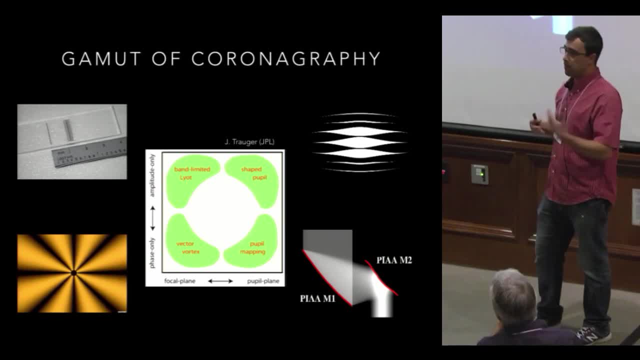 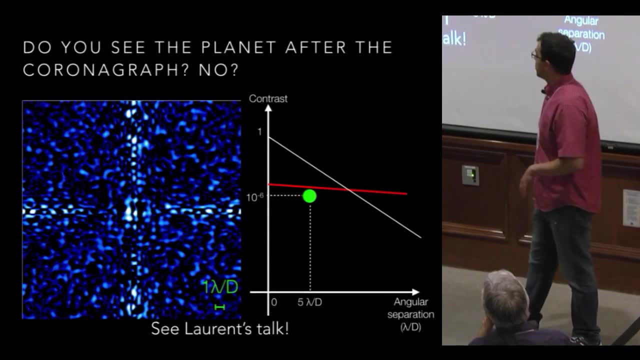 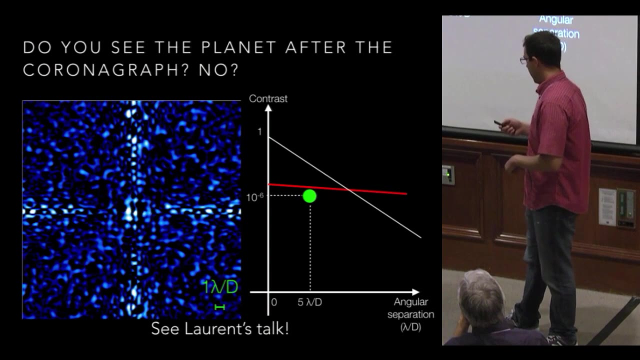 So these coronagraphs use a mix of phase and amplitude modulation in either the focal plane and or the pupil plane. So a coronagraph would remove the diffraction from the system very efficiently. so the coherent part of the wavefront. and so now I've put my coronagraph. 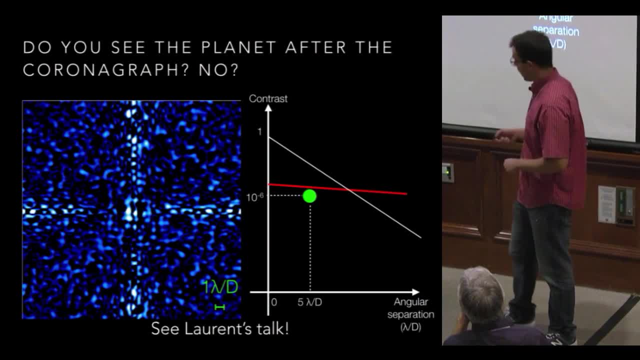 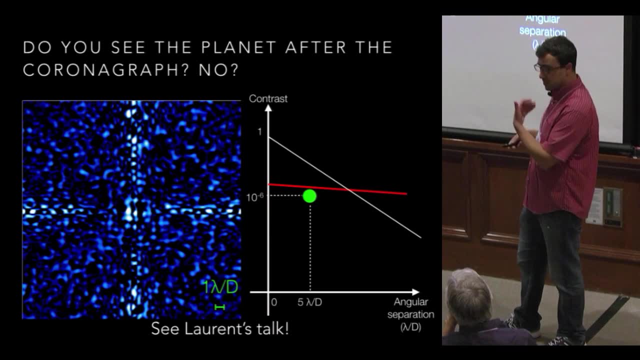 in my super-duper adaptive optic system. so do I see now the planet finally, after all these efforts? So unfortunately I don't see the planet. The planet here in this fake data set is about a million to one at the million to one contrast ratio. 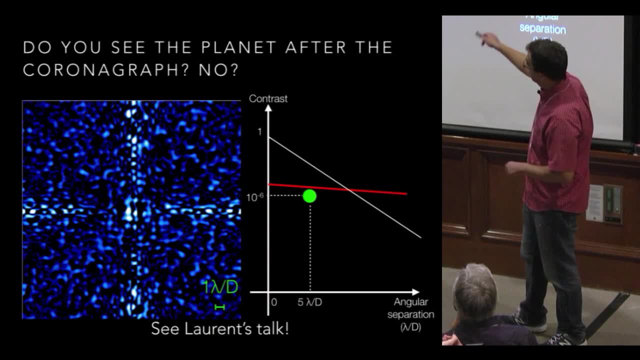 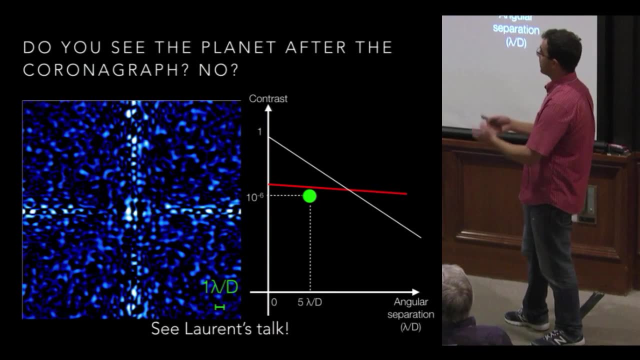 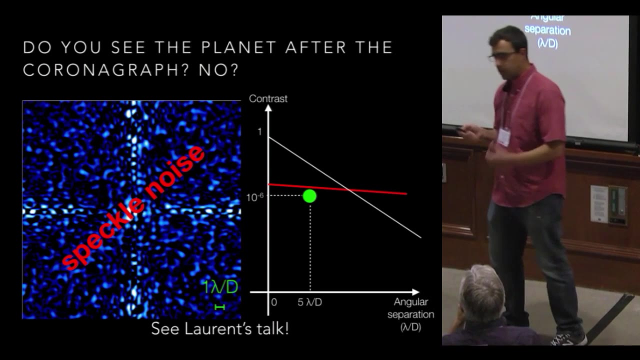 with respect to the central star. So most of the features you see here are residual from the starlight that interferes with itself to propagation effects in an imperfect topical system. These features are called speckles, And speckle noise is the number one issue. 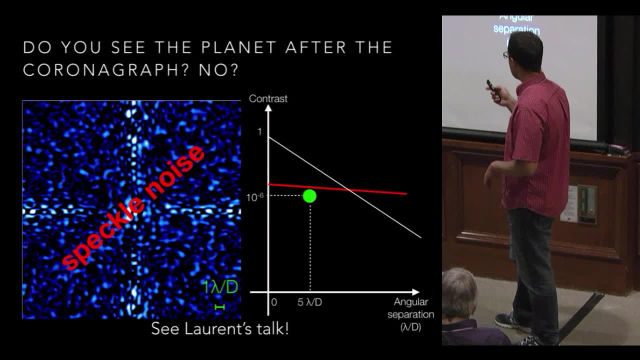 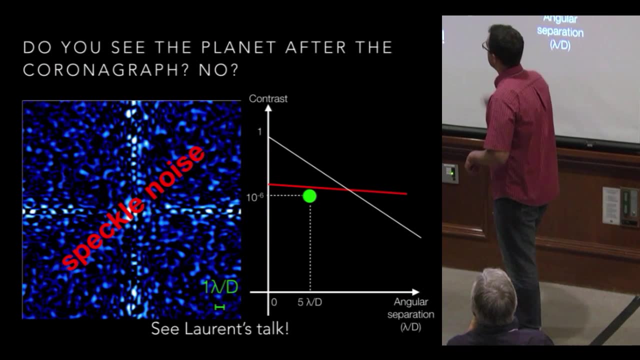 in direct imaging. So you see, speckle noise here prevents us from seeing the planet because it is above the contrast ratio of the planet itself. So the planet could be one of these dots, but there is no way we can tell which one is a real planet. 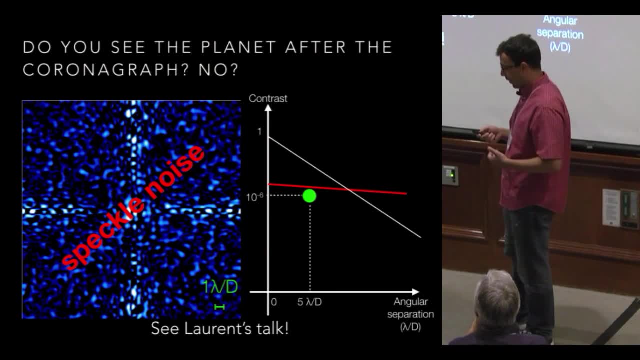 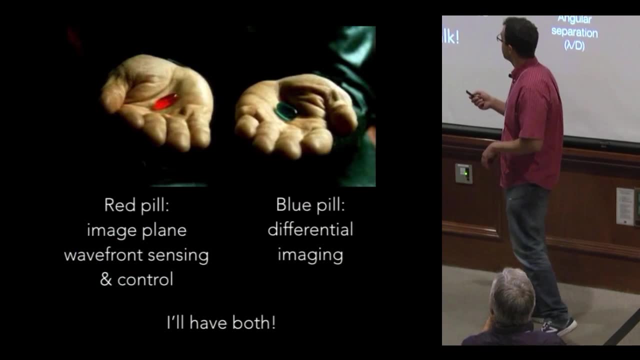 versus a speckle, because they both have the characteristic size of the diffraction, which is one lambda over d. lambda is the wavelength and d is the diameter of the telescope. Okay, so two choices here. We either try to push the adaptive optic system. 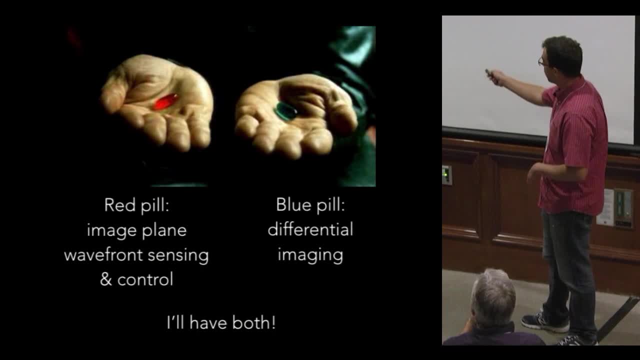 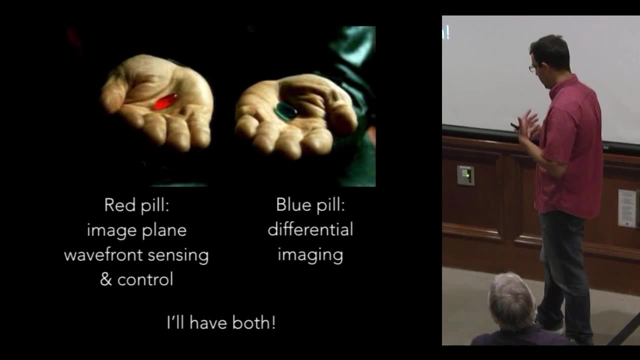 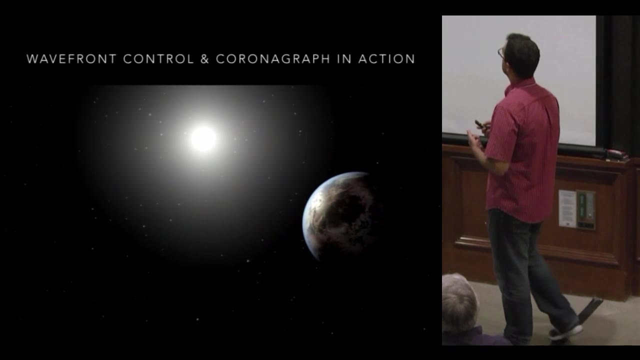 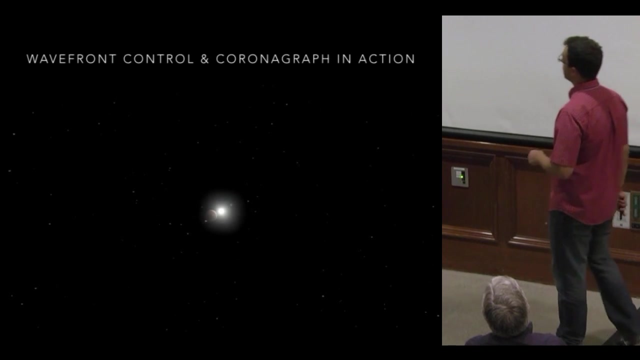 to kill those remaining speckles. so that is wavefront control or we implement differential imaging. In practice we use both approaches to kill this speckle noise. This is another movie showing an example of wavefront control. So this is here an extrasolar, planetary system. 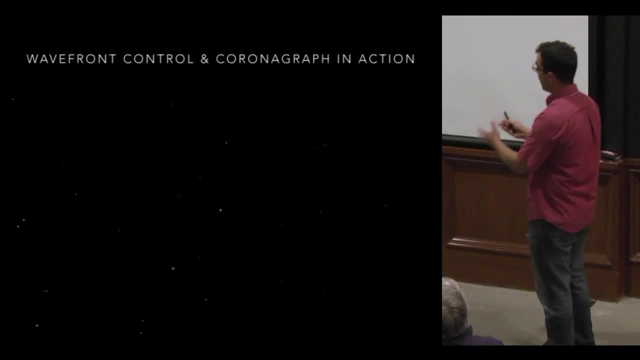 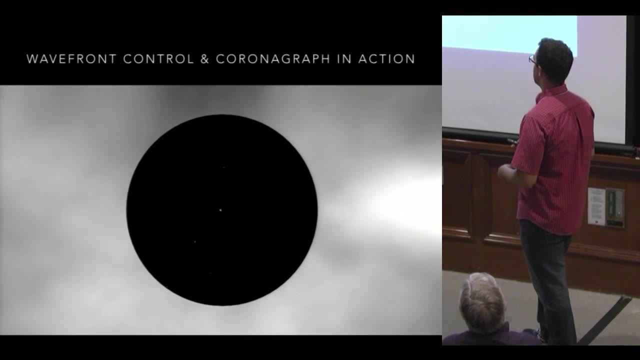 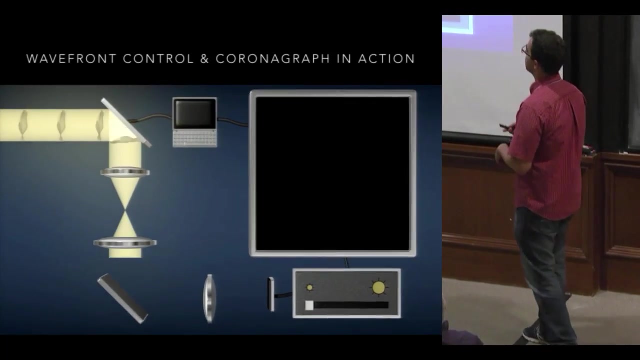 with two planets. So, seen from the Earth, everything is blended together. So this is a space telescope. So the wavefront from the system enters the telescope. the wavefronts pick up aberrations as they propagate through the imperfect optics of the telescope. 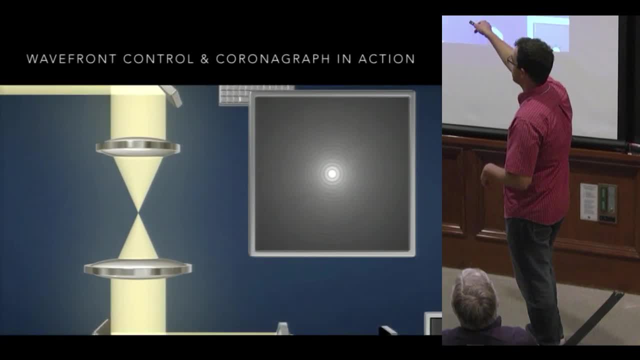 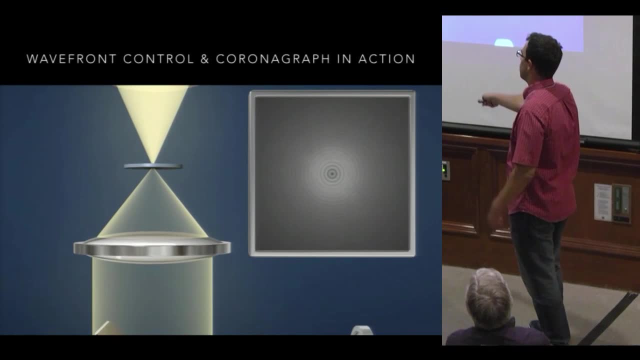 This is here the entrance lens of the chronograph instruments. at the focus We are going to put this chronographic mask. This is the field lens that is going to produce an image of the entrance aperture where we put the LEO stop. This movie, by the way, has been made. 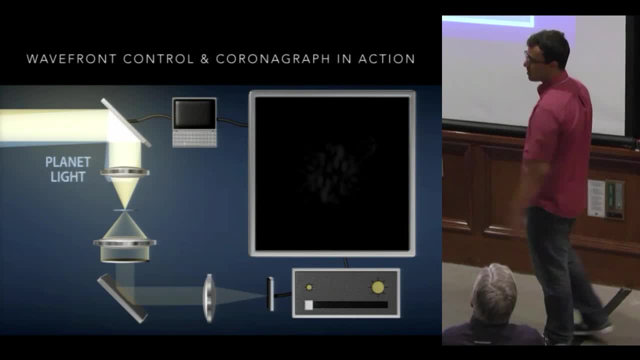 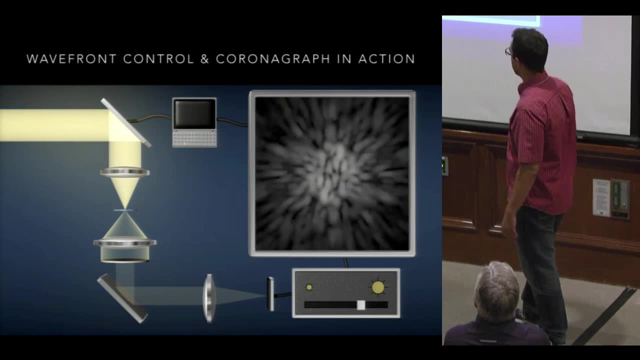 for WFIRST. as an illustration of WFIRST, and you see here most of the ingredients, if not all the ingredients- of the original LEO chronographs are in WFIRST. So we finally make an image and you see these speckles again. 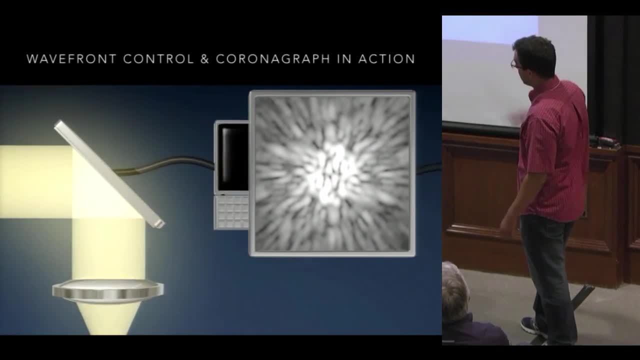 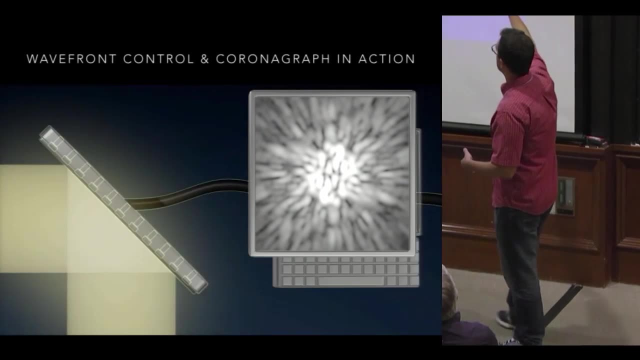 So first way to kill them is to actually push the adaptive optics system to kill them. So again, we will move the actuators of the deformable mirror to try and control these speckles. and there are many ways to do that, based on the image, science, image itself. 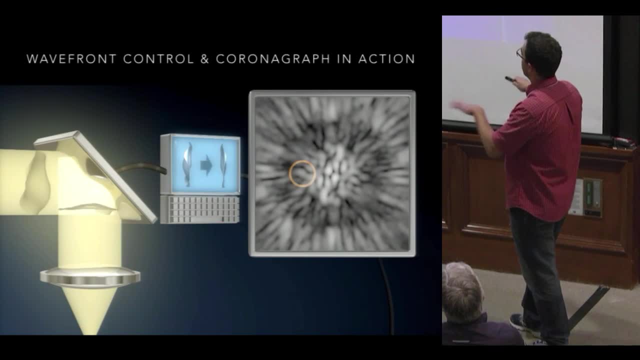 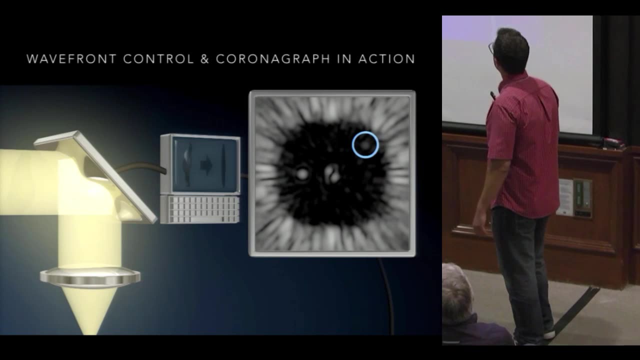 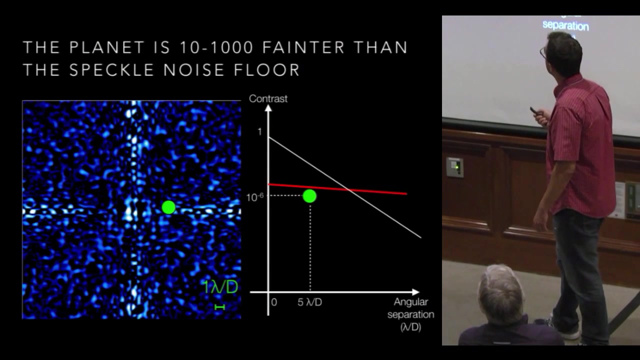 And so the deformable mirror will flatten the wavefront in a way and kill those speckles and reveal the exoplanets. So this is technique number one. Technique number two is differential imaging And differential imaging. let's go back to our speckle, noise, image. 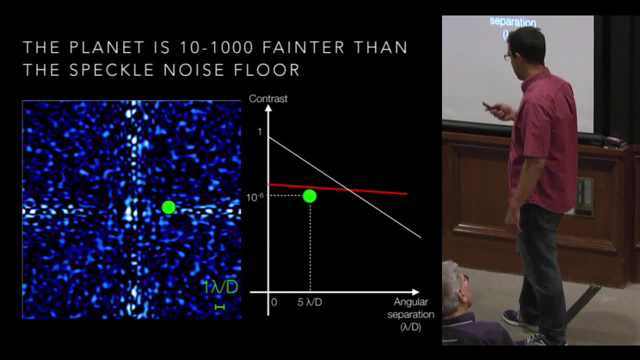 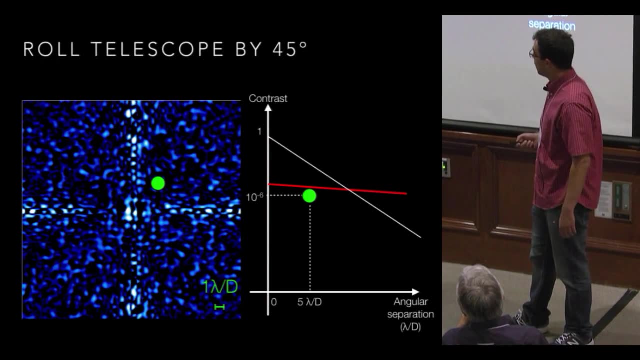 And so the planet here is this green dot. So I'm cheating, I'm telling you where the planet is, So I'm going to take an image here, image number one- Then rotate my telescope by 45 degrees around the optical axis. 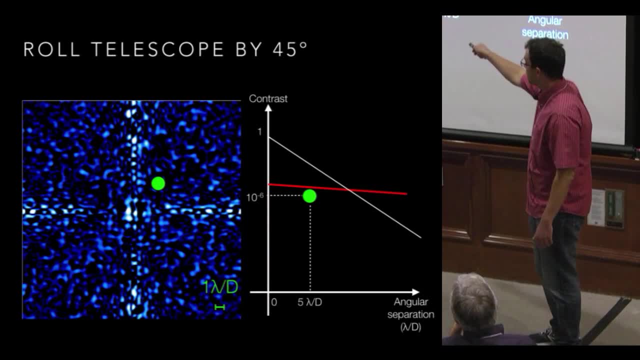 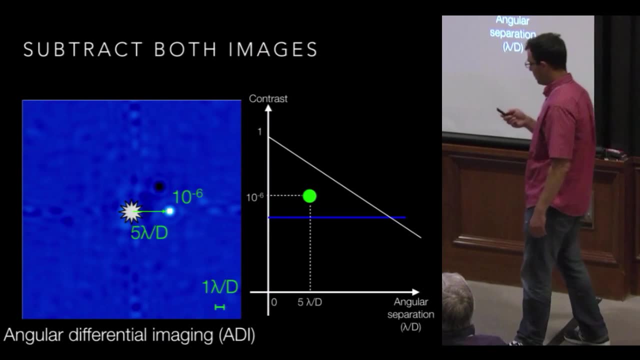 and take another image- And I'm hoping that these speckles are stable enough so that they won't move, they won't change between these two images- Then I subtract both images and that indeed reveals the planet. This technique is called angular differential imaging. 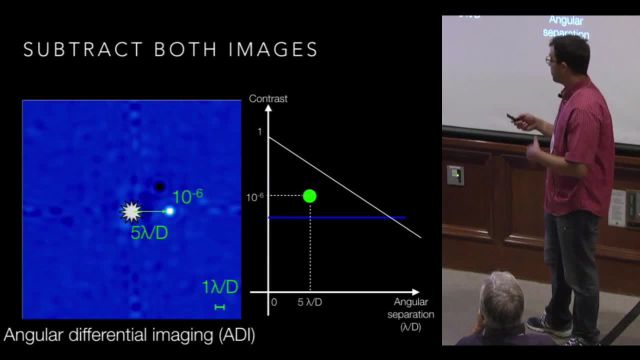 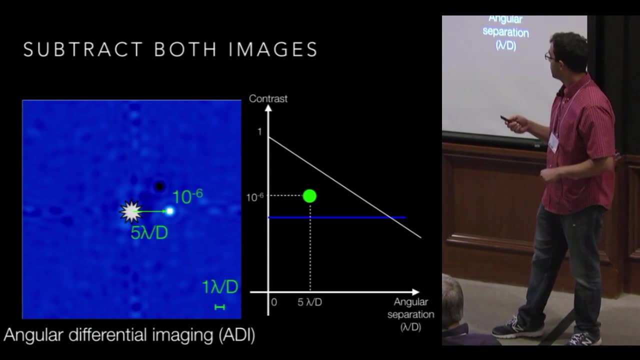 or roll angle differential imaging, And this is the technique that has been used to make all these images that I showed at the beginning of my presentation. So this is a very powerful technique indeed. This is not perfect, because there is a time delay between the acquisition of these two images. 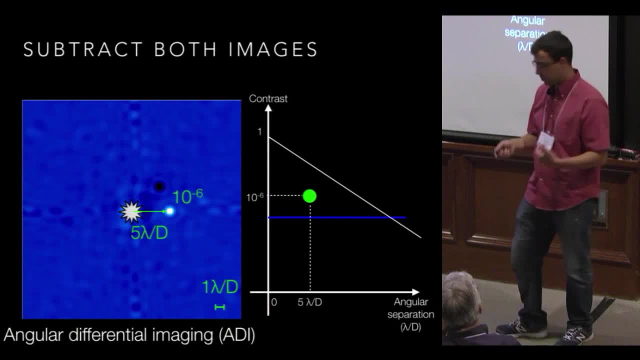 that make the speckle slightly evolve in the background, And the reason speckle evolve is because the telescope is subject to gravity vector changes or thermal changes, and that modifies the shape of the optics that create these small instabilities and that prevents us from subtracting. 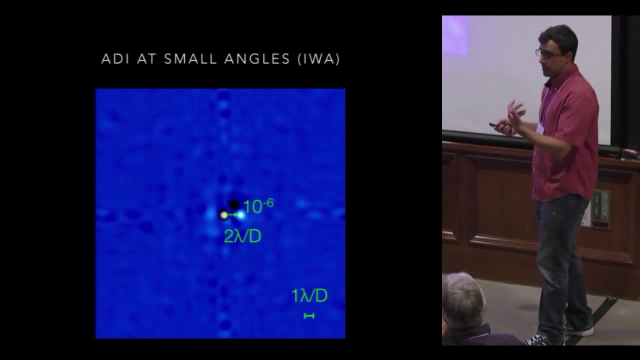 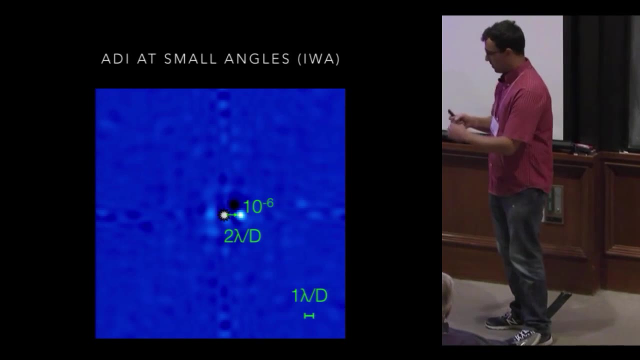 the speckle noise efficiently. There is another problem with this technique: angular differential imaging, that is, if the object is very close to the axis. the amount of displacement of the object for a given roll angle is becoming smaller and smaller, and one gets closer and closer to the star. 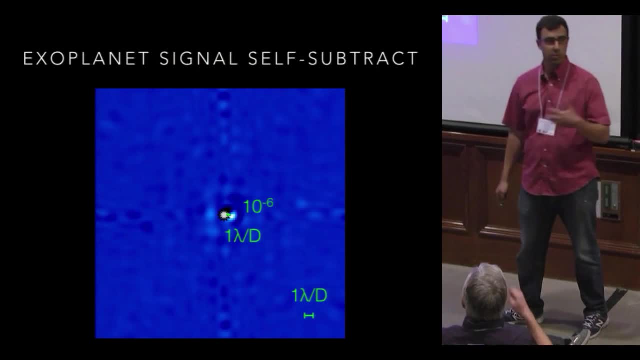 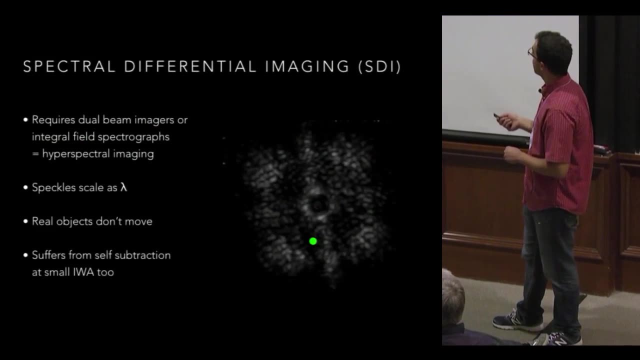 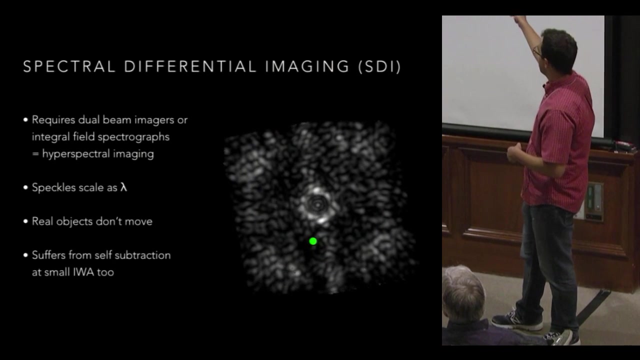 So that is a technique that is affected by what we call self-subtraction or self-attenuation phenomenon, and that is a function of the angular separation. There is another differential technique here, which is spectral differential imaging, so this is what we call a data cube. 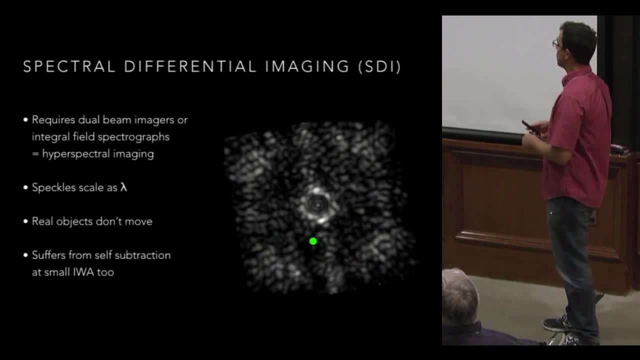 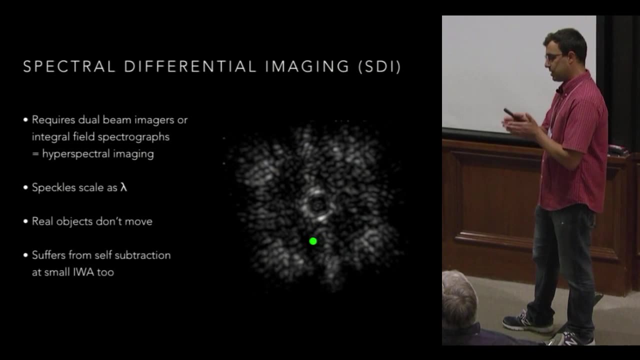 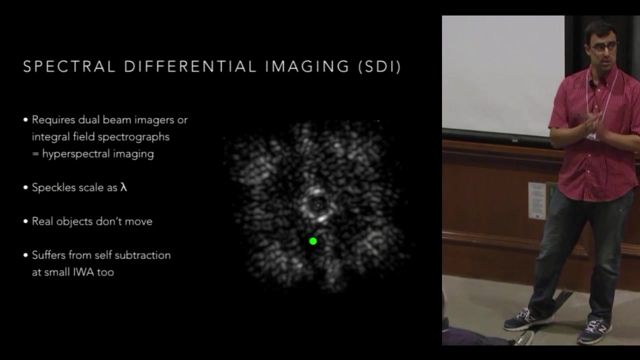 made by the SPHERE instrument at the very large telescope in Chile, So that uses what we call integral field spectrograph that takes images at different wavelengths simultaneously, And here we can use the fact that speckles remember. the scale of speckles is lambda, over d. 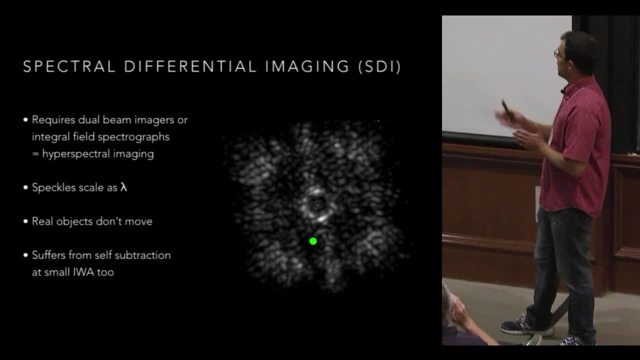 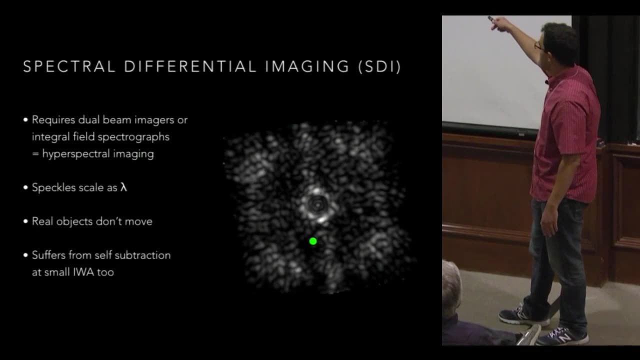 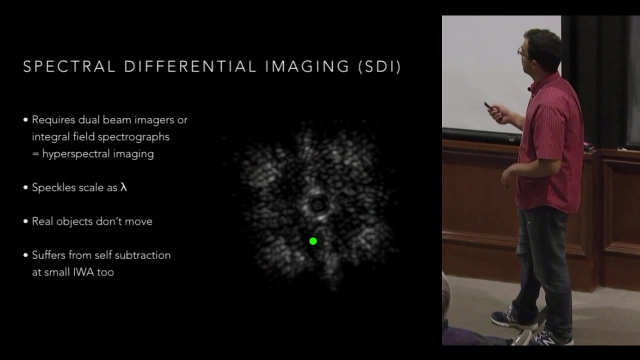 so it's proportional to the wavelength. so the speckles scale with the wavelength, And so why the planet does not? So using that fact and this radial modulation, we can actually disentangle between real objects and speckles. The problem with this technique is that 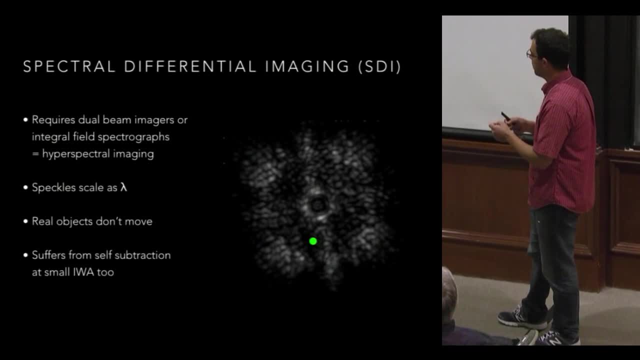 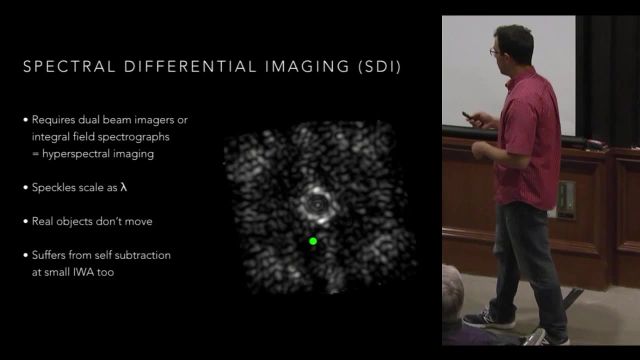 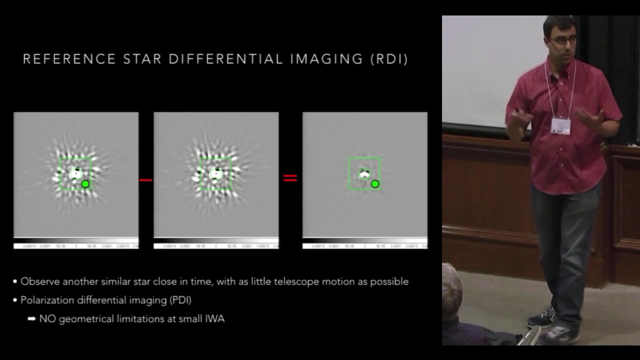 instead of using radial azimuthal modulation, like angular differential imaging, one uses radial modulation, and both are affected in roughly the same ways by self-subtraction phenomenon. Another technique that is extremely simple is just to observe another star without the planet and subtract it from the target itself. 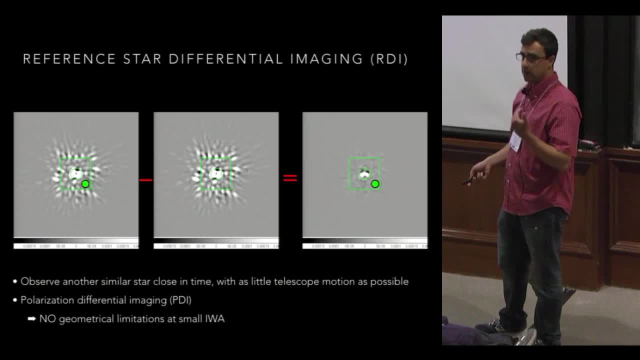 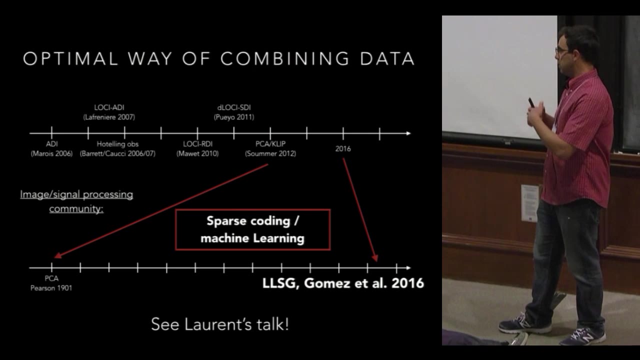 So that is a powerful technique, but again, that assumes that there is no evolution or substantial evolution of the wavefront or the speckle field between the two images. And finally, when you got your data set of images, hundreds of images sometimes- 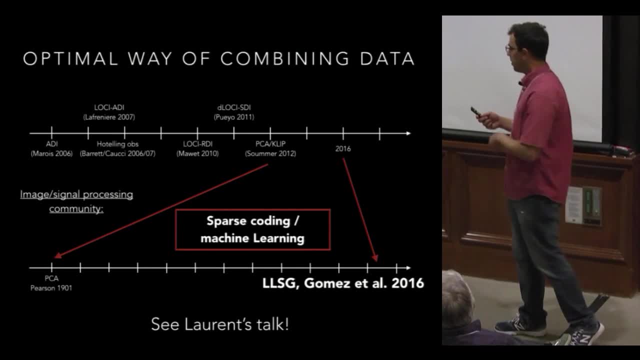 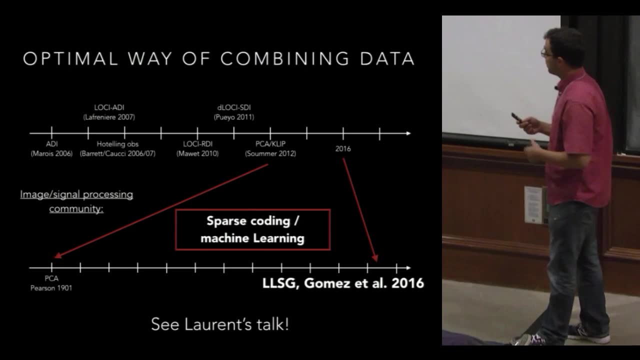 what is the best way to combine them, And I think I'll defer everything to Laurence Stoke, who is going to go in detail over this. The current state of the art, or the widespread method used in direct imaging method, is principal component analysis. 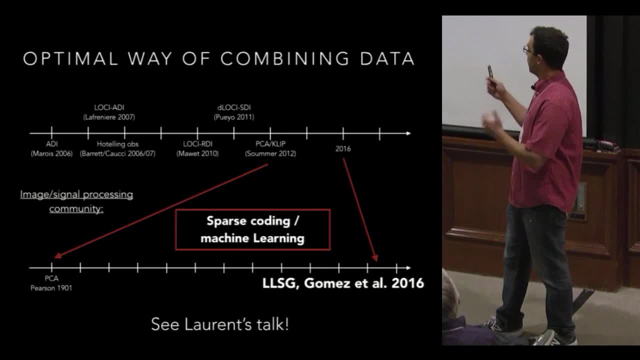 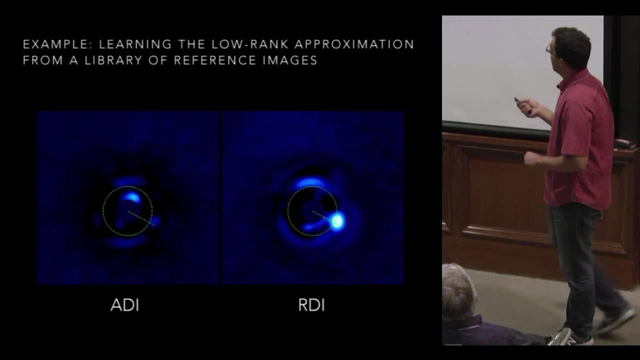 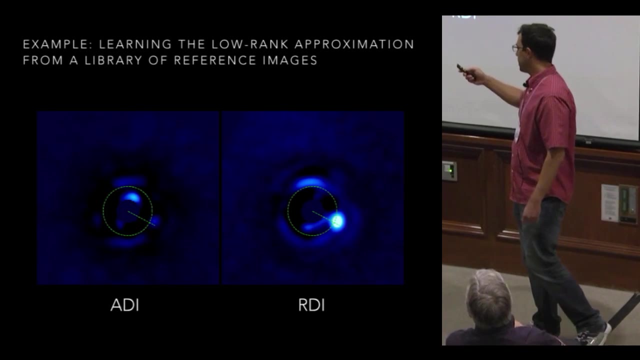 So that's what we use to subtract these speckles from target objects. Okay, so I'm just showing you this because I like that very much. So that shows you why ADI basically doesn't work very well at small angles. So this is here a data set. 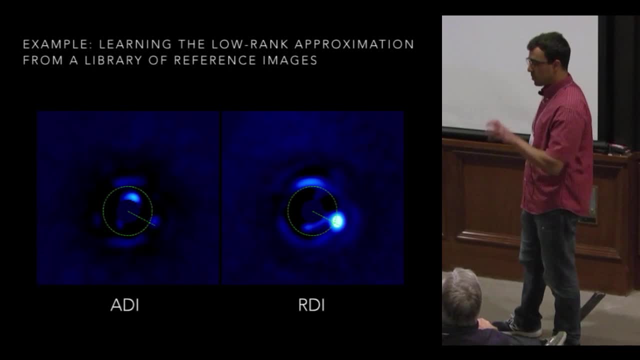 an angular differential imaging data set with an object that is at very small separation. So it's about 2 lambda over d, so 2 diffraction beam width from the central star. So an angular differential imaging data set here completely attenuates the object that is here. 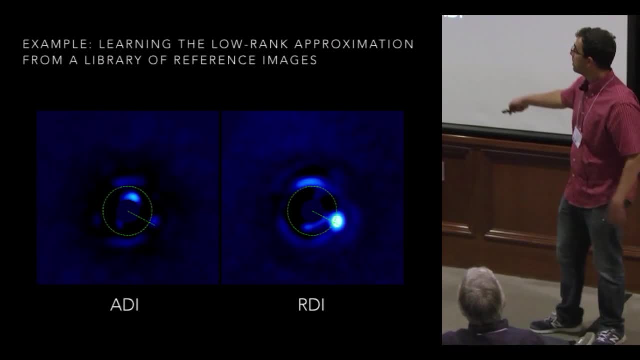 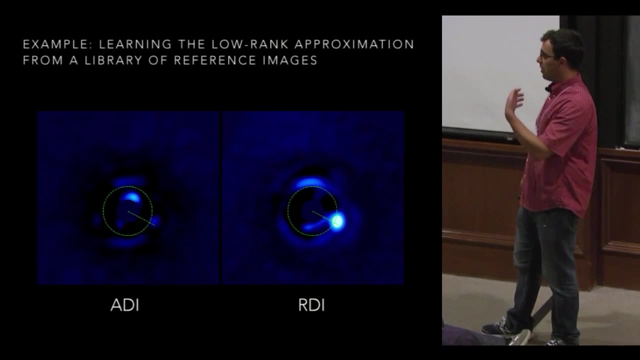 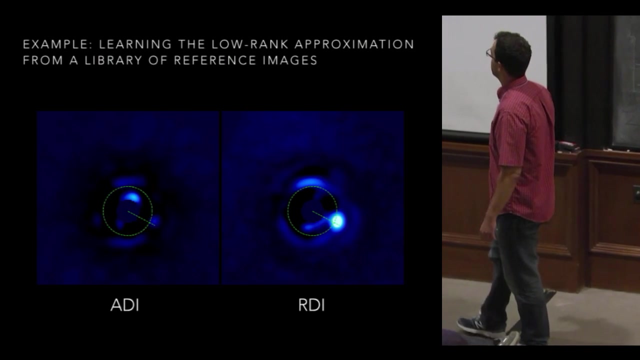 And based on this data set alone, there is no way you can actually affirm with high confidence that there is indeed a planet as opposed to a speckle. Using this reference star subtraction and PCM methods, you can actually recover the companion with very high confidence here at very small angles. 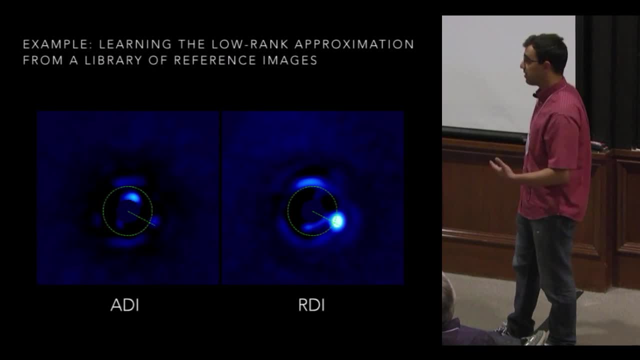 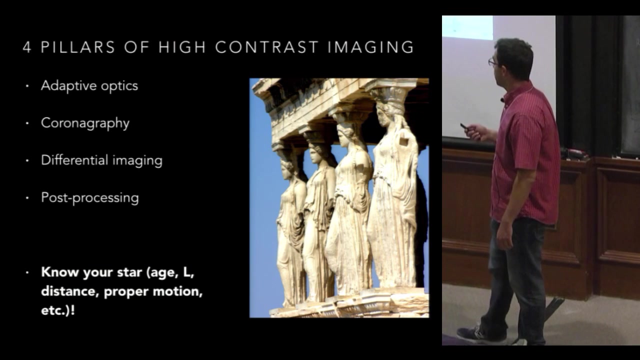 So these reference star differential imaging methods are not affected by self-subtraction. So that is, I think, the future of direct imaging, but that relies on good management of data and data mining techniques. Okay, so there is a fifth pillar that is hidden. 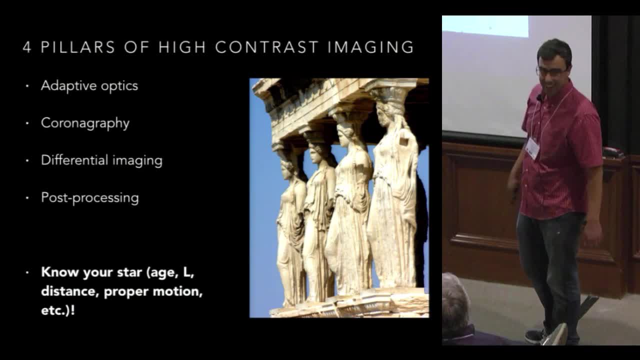 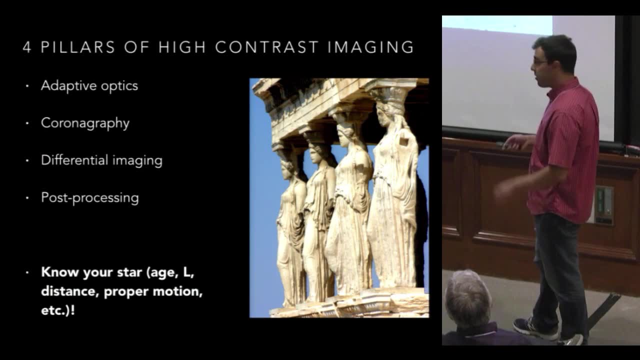 You see it here In the back. Okay, This is perhaps the most important one right now for direct imaging from the ground. So everything is related to the star, to the central star, So we base everything on it, So we base our inference of planet masses and properties. 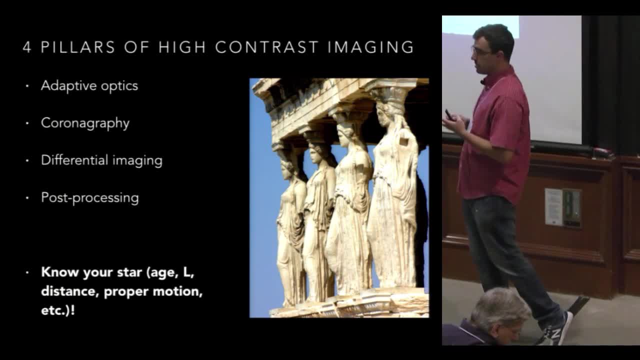 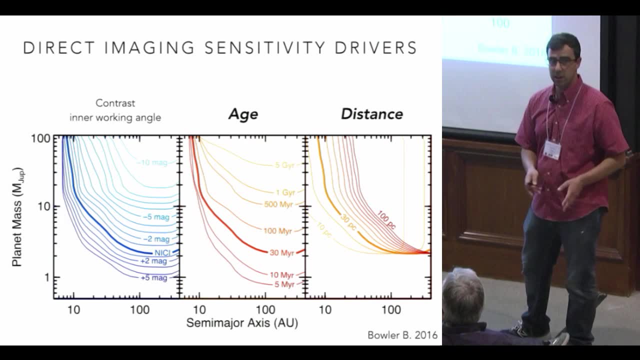 on the edge of the star, on the luminosity of the central star, its distance, its proper motion, Okay, And that is all. those factors about the central star have much more dramatic effects than actually changing the waveform sensor speed by a factor of maybe 20%. 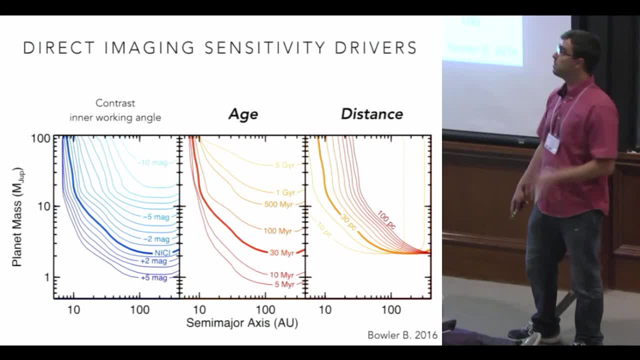 So this is extremely critical to current direct imaging surveys. So one has to know the properties of the central star extremely well, And this is here an example taken from this fantastic review by Brendan Bowler, which I really recommend you read. That's the most recent and the best review. 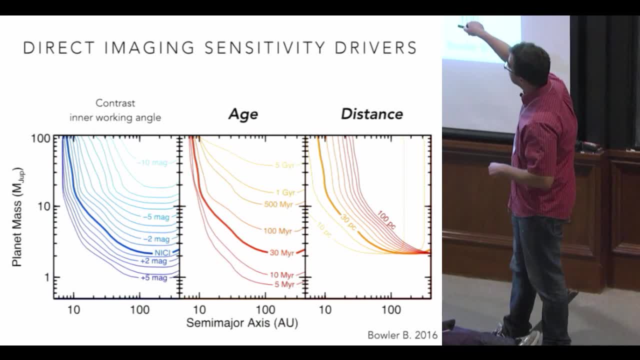 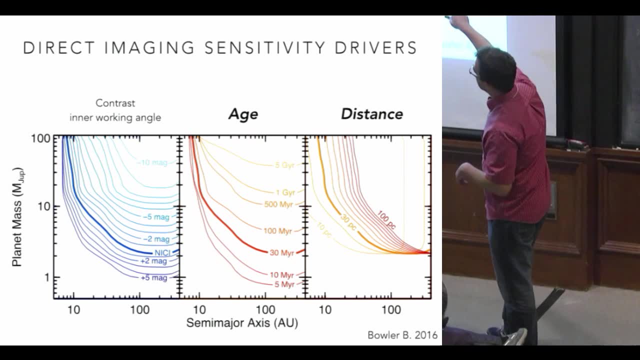 I've seen, for direct imaging surveys. So this is here again in this planet: mass versus semi-major axis space, in the log-log space, unfortunately. So this is from 1 to 100 Jupiter masses And this is here showing you the NIKI. 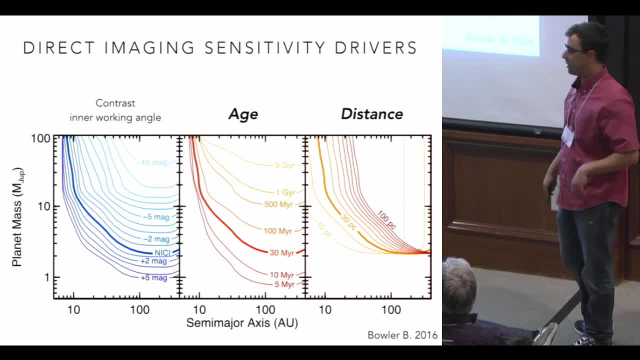 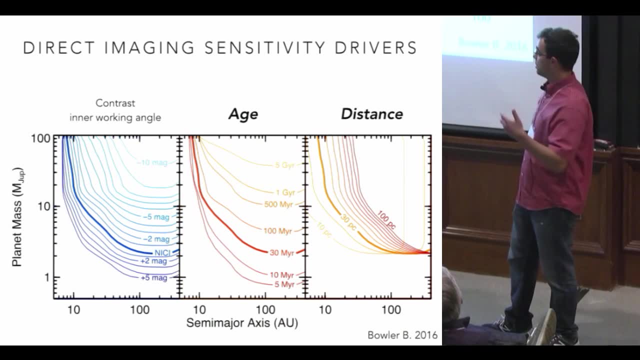 the performance, the average performance of the NIKI survey. So NIKI was this first generation adaptive optics system at Gemini, prior to the famous now G Gemini Planet Imager. And you see here the changes in contrast performance by NIKI by these values. 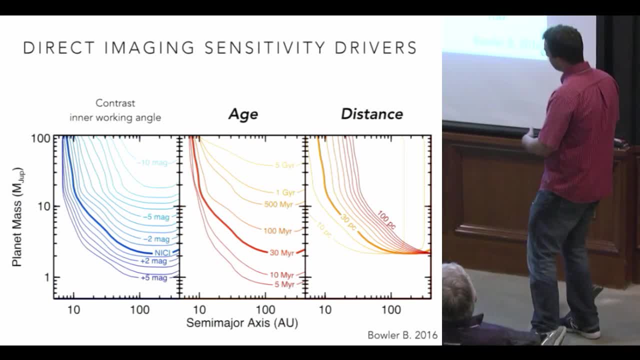 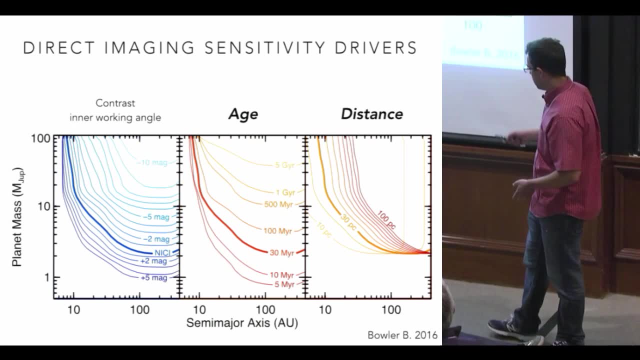 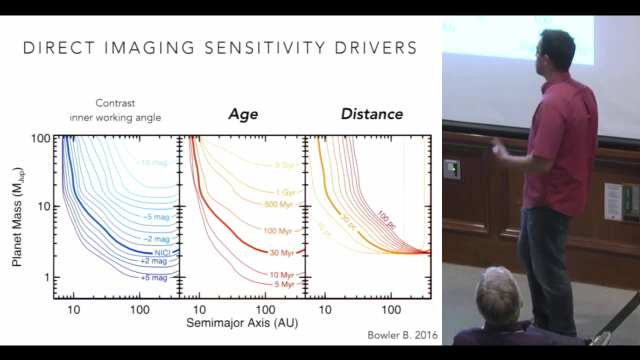 so a few magnitudes, which is which is huge. I mean that requires working extremely hard on the wavefront sensor, on the deformable mirror, all these technologies. You see that these changes here do not show up very advantageously in this planet. mass versus semi-major axis space. 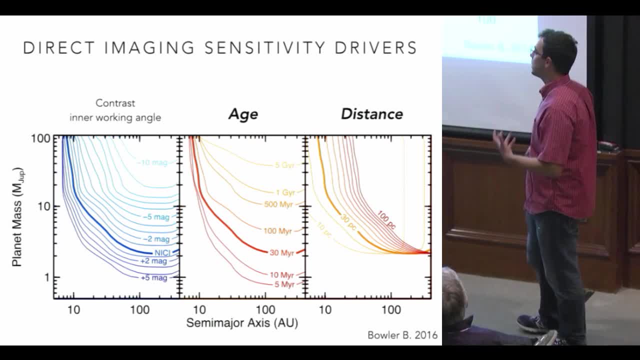 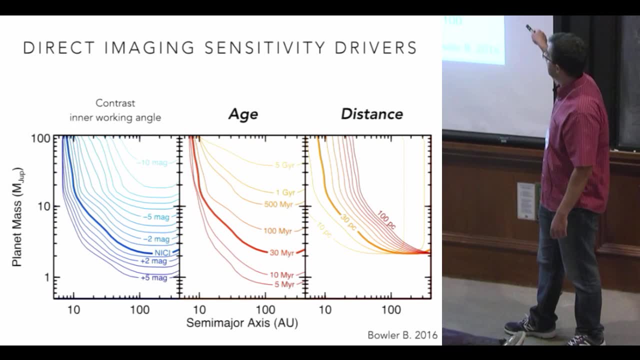 While the edge- here you can see that a factor of a few in edge has a much more dramatic effect on the sensitivity of direct imaging of young objects. And that is the same for distance here, which has an effect on the inner working angle of the chronograph. 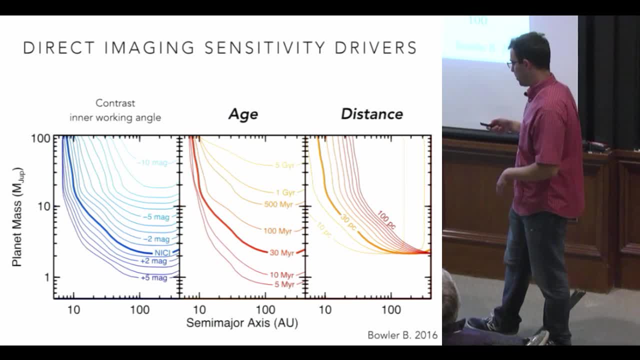 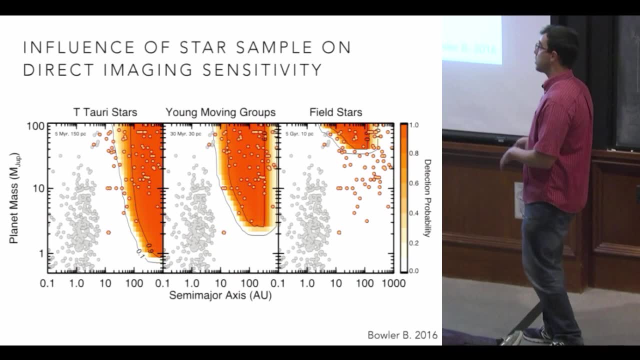 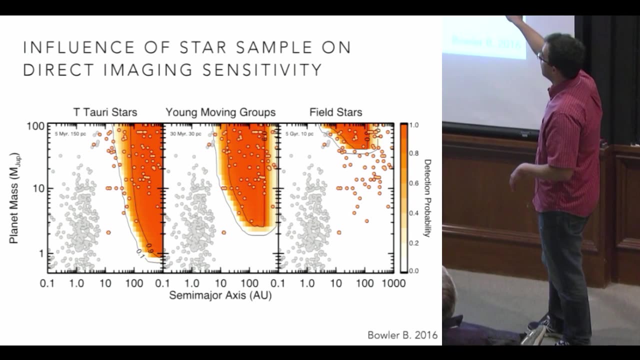 So age and distance are two of the key parameters for determining the sensitivity of direct imaging surveys, And that is the reason why we have focused on these very young and closest possible objects. So typical samples are teetering stars in star forming regions which are extremely young. 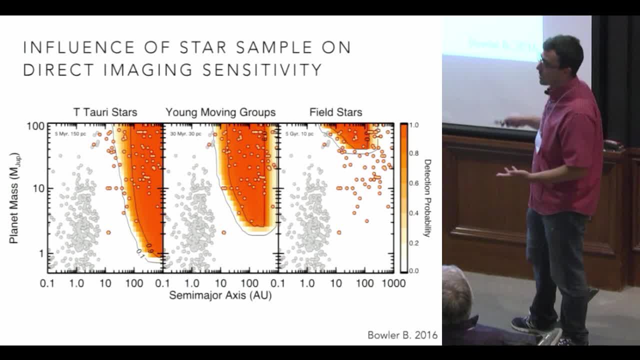 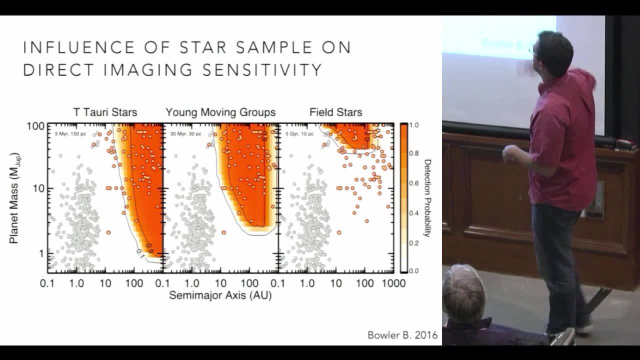 So the sensitivity here is very good. The inner working angle, unfortunately, is not very good because these objects are really far away. At the other end we have field stars which are much closer. so the inner working angle in principle should be very good. 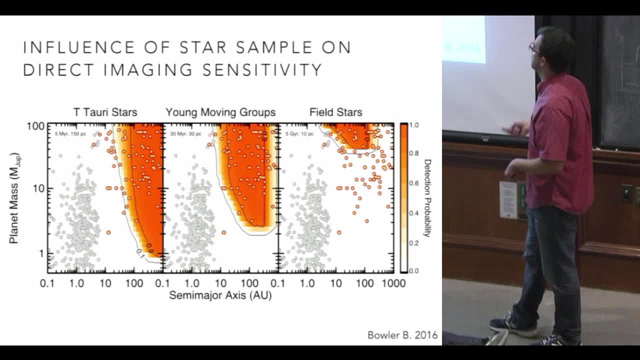 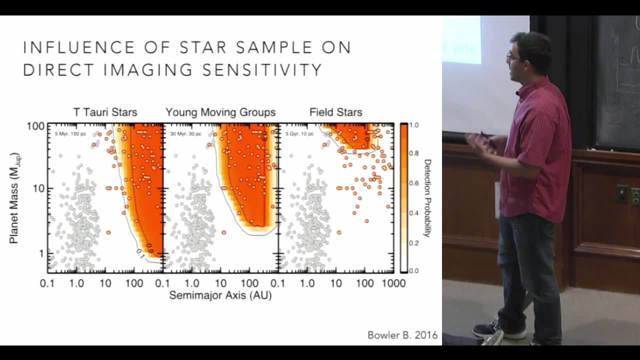 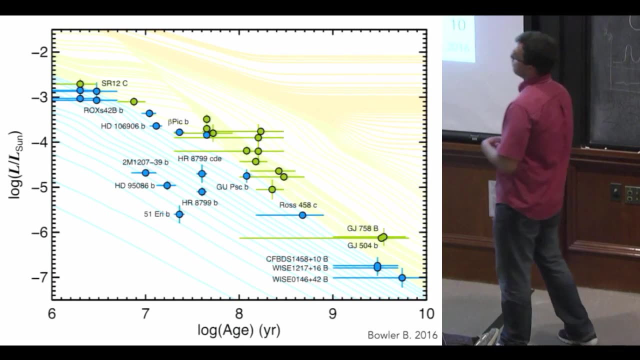 but these objects are generally old so their sensitivity there is not very good. So the sweet spot for direct imaging surveys are these young moving groups which represent the best compromise between distance and age. So the problem here with direct imaging, perhaps one of the most pressing problems. 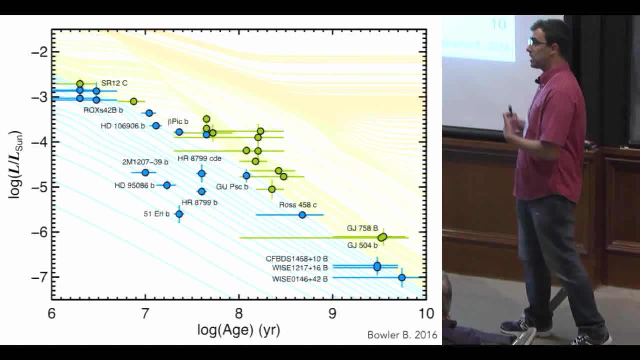 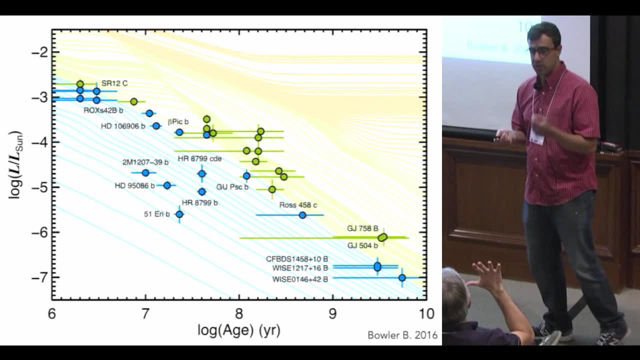 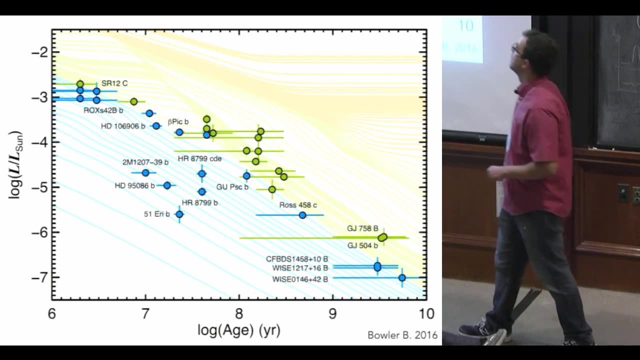 is the ambiguity to the process of mass and temperature inference. So the only thing that direct imaging currently measures is the luminosity, And the luminosity of young planets is a very steep function of age, And so that is why most objects here that have been discovered so far 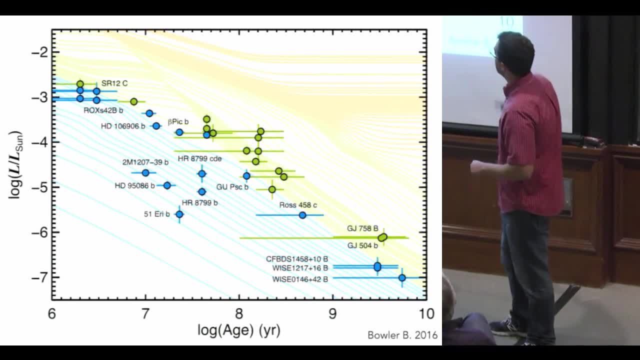 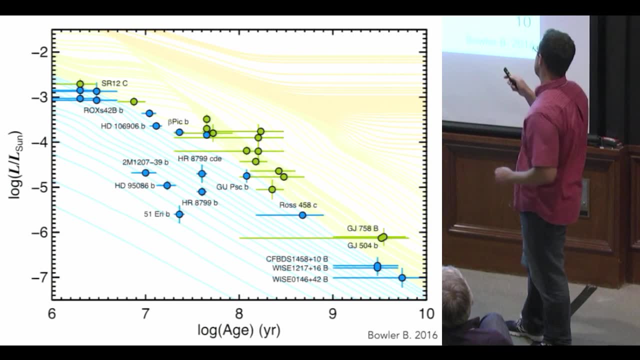 have these large arrow bars in X. The other problem is that there is a very steep separation between the planet mass regime and the Born-Roth regime And you see that these isomasses in this plot here are very tight and compact and close to each other. 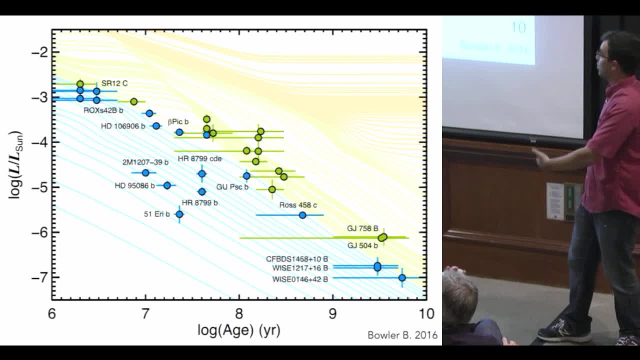 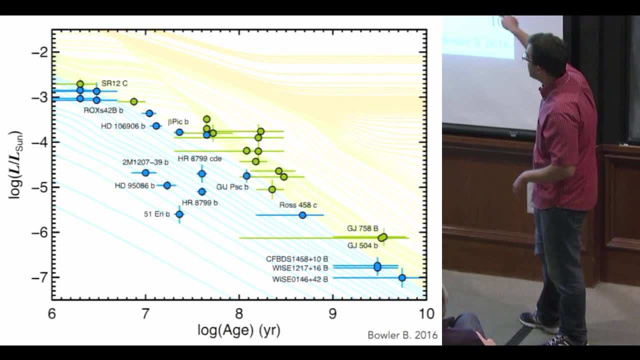 The transition between the planet regime and the Born-Roth regime, which is around 13 Jupiter masses, where the deuterium burning kicks in. And so you see here that there are many, many objects that have been discovered by direct imaging that lie right at the transition. 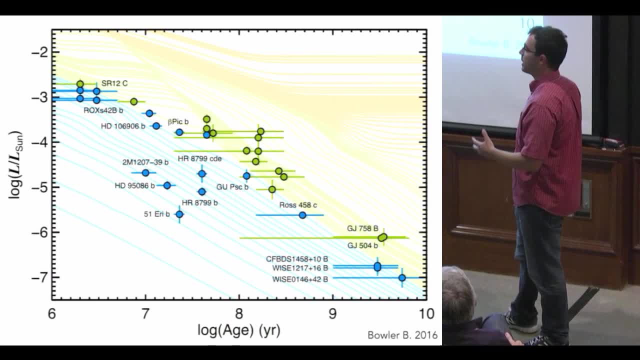 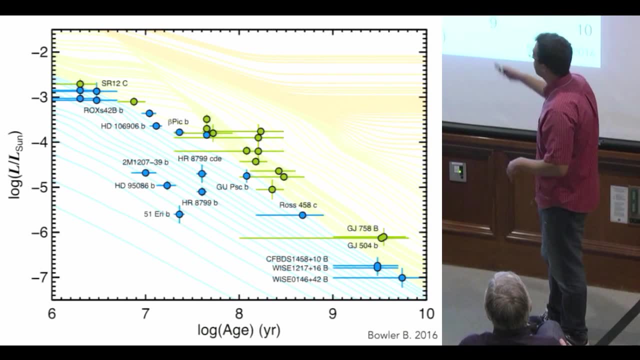 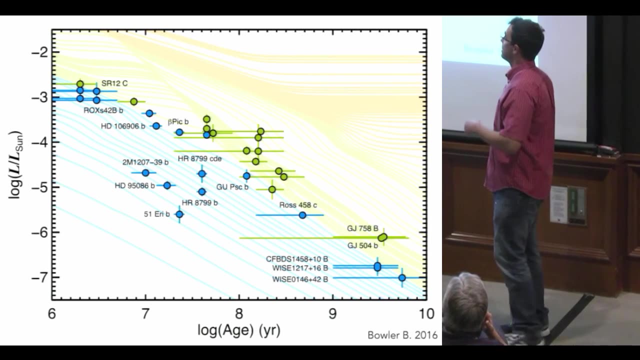 between these two regimes, And the uncertainty on the edge makes us very unconfident about the nature of most of these objects. So there are only a handful of bona fide exoplanets discovered by direct imaging, And most discoveries lie at this deuterium burning limit. 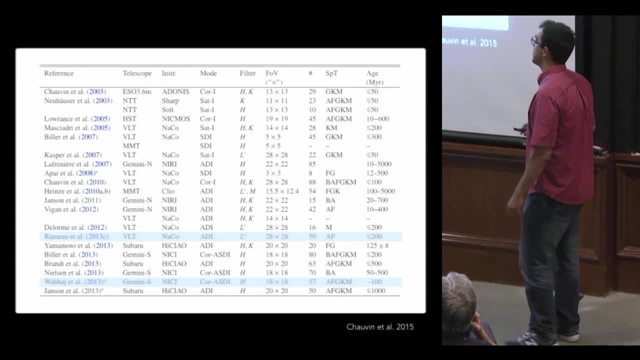 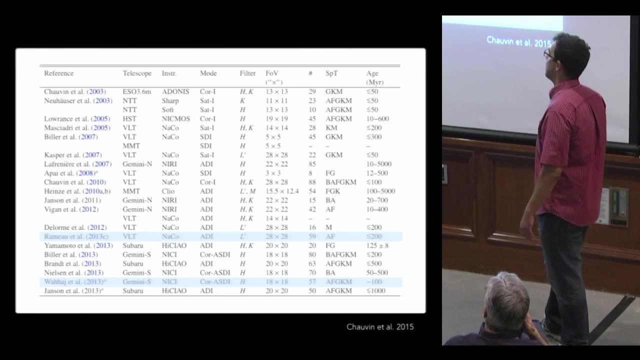 Okay, so I'm going to go quickly over the result of 15 plus years of direct imaging surveys. So this is here a non-exhaustive table showing all the surveys that have happened over the past 10, 15 years using different facilities here. 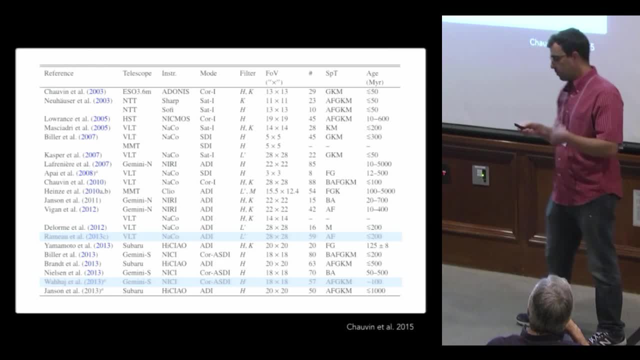 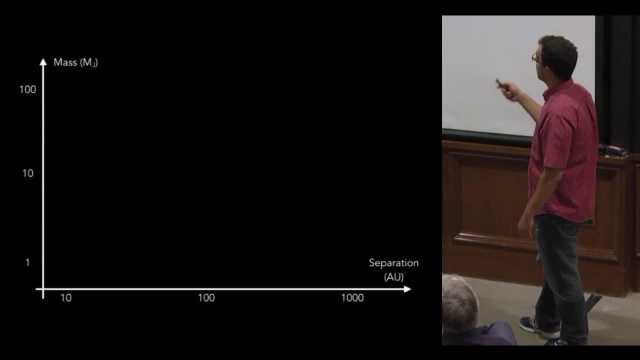 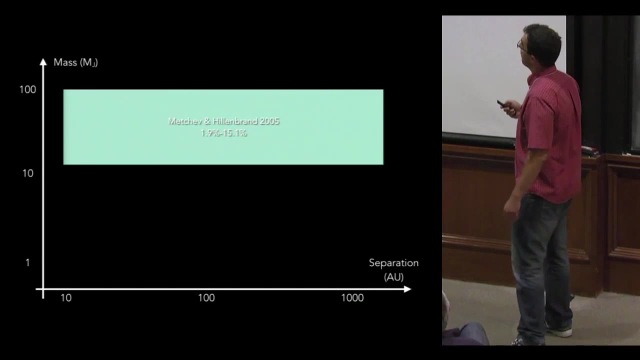 So that represents thousands of hours of telescope time worked by hundreds of people. And so this is here again in this mass versus separation diagram. So I'm going to plot boxes and results of the occurrence rate inferred by these teams as a function of time. 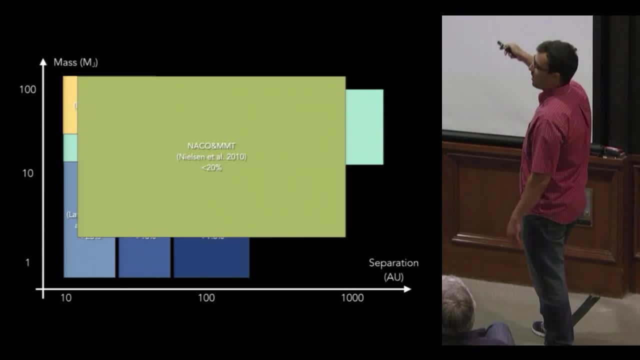 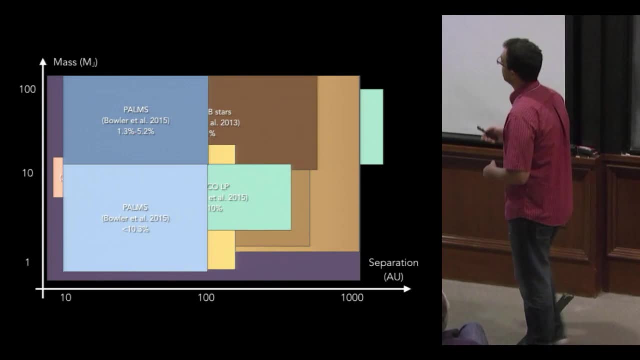 So let's start. It's going to go quickly, So I'm just going to give you the final word. But you see here the face coverage of most surveys over the past 15 years. So you see that they focus on different parts of this diagram. 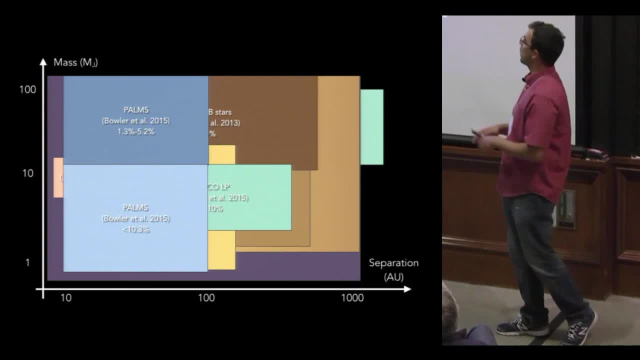 and that is mostly due to the fact that they targeted different samples. So, going back to this distinction between moving groups and star forming regions, Okay, so the summary, again referring to Brendan's paper, the summary of all these surveys has been synthesized by Brendan. 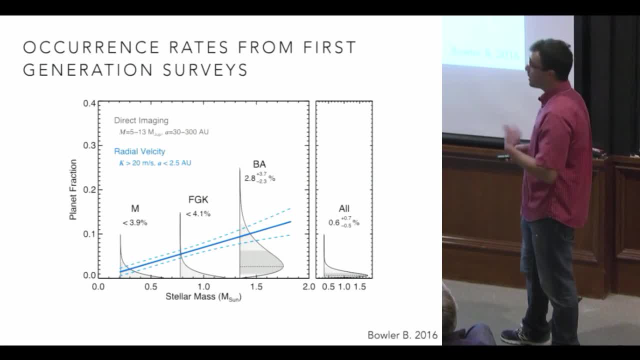 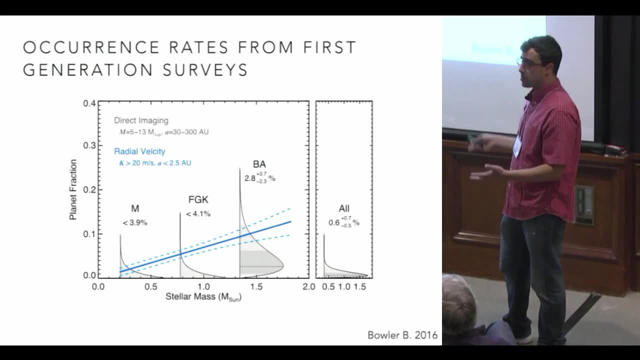 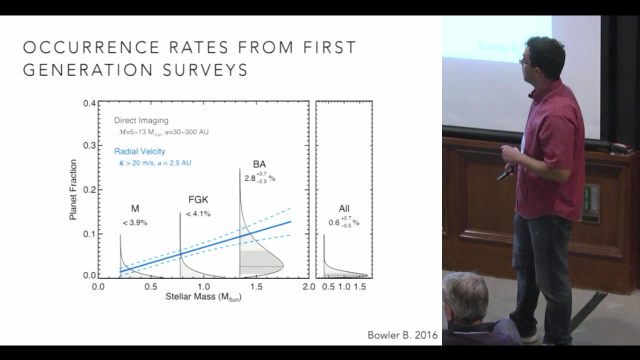 in his recent paper here And the result, the final result of direct imaging surveys, is quite depressing in some ways And the reason perhaps why we haven't discovered that many objects, the occurrence rate of giant planets, young giant planets around all the stars we've looked at. 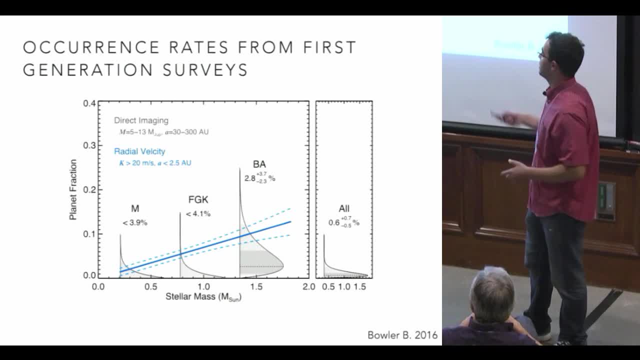 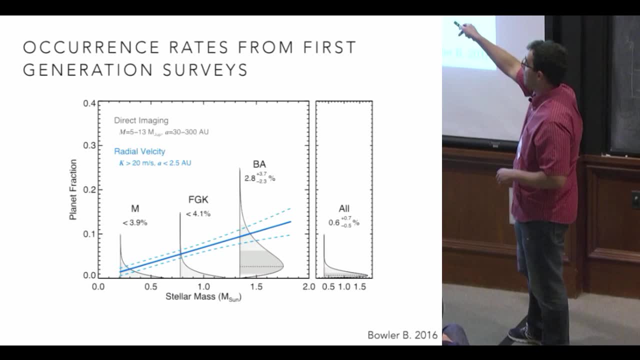 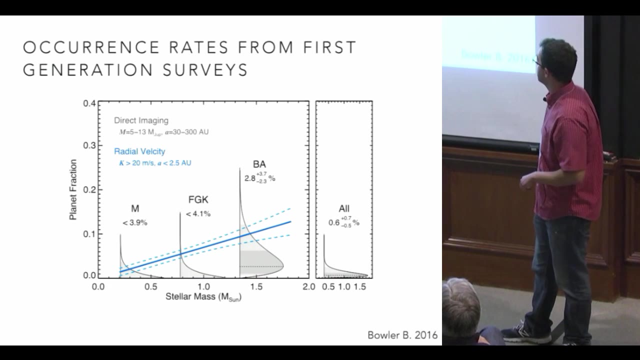 so it's about 400 stars in this particular synthesis is about 0.6%. Okay, that is in this mass range. So from five to 13 Jupiter masses at those separations between 30 and 300 AU, which is where we are sensitive to planets. 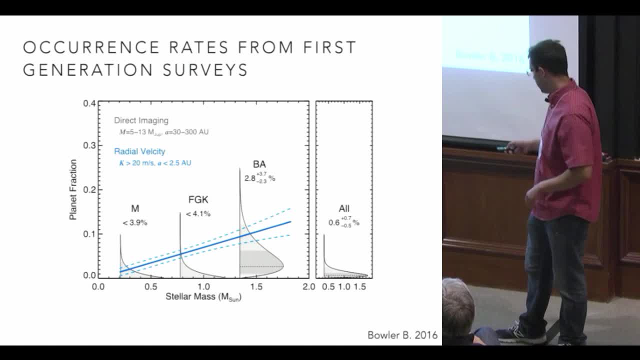 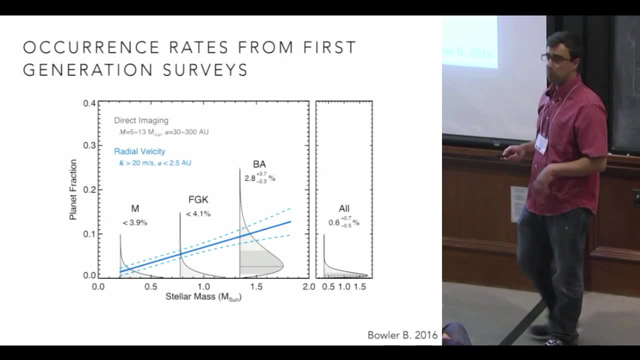 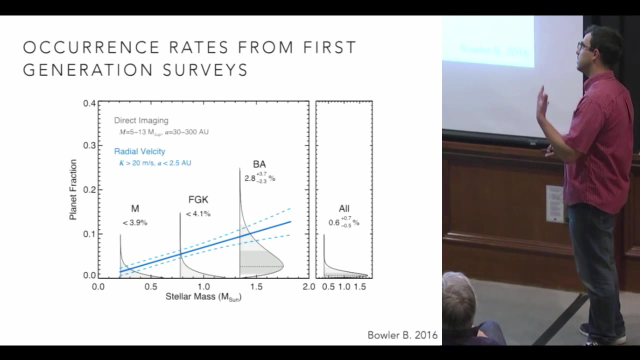 So that is maybe the take home message here. The occurrence rate of young giant planets is extremely small, So nature is not efficient at producing these large separation objects, which tells us something about their formation mechanism that is unlikely to be the one we assume for our own solar system. 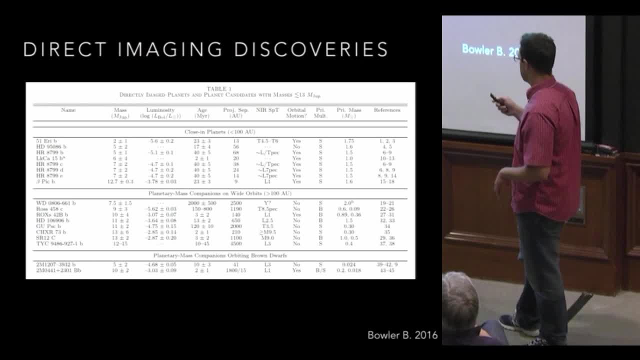 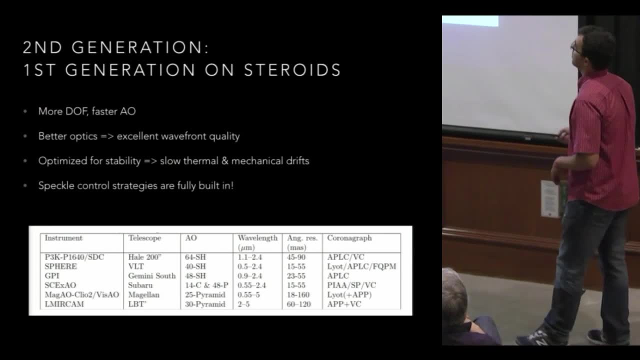 So this is here a summary of all these objects. So I refer you to Brendan's paper for a complete list. So I'll quickly go over second generation adaptive optics system, which are now starting a new generation of surveys that are more sensitive. 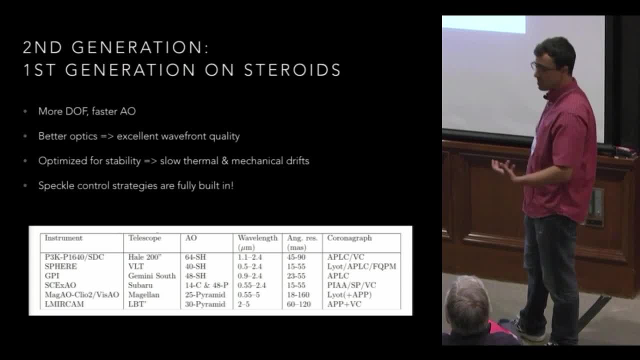 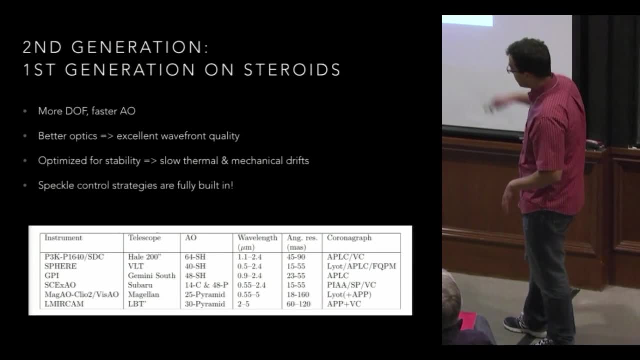 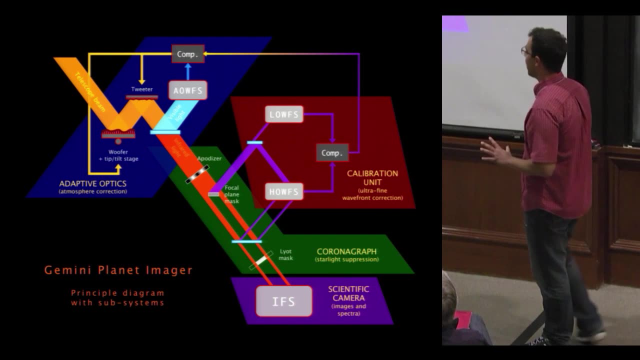 So these surveys use extreme adaptive optics systems. so it's adaptive optics systems on steroids that are optimized for stability. This is here just a list of different surveys for you to read after my talk. This is to show you quickly how complicated these instruments are. 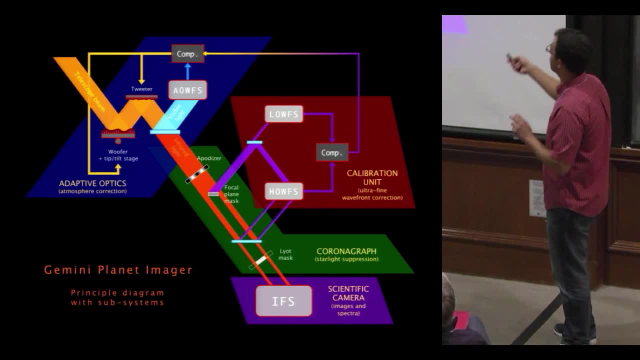 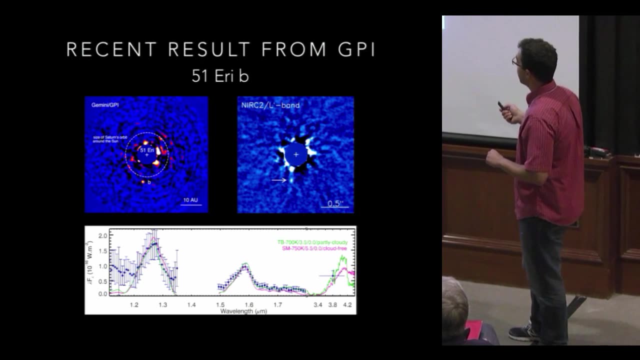 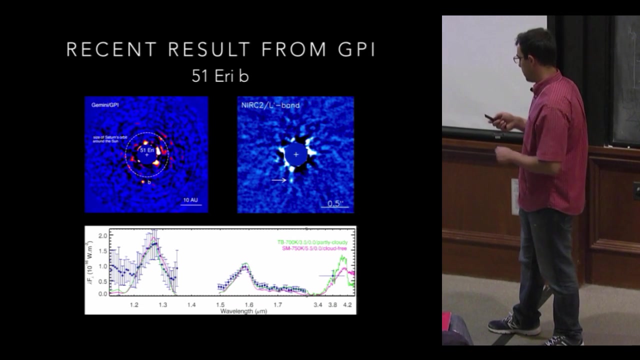 with different modules of adaptive optics, calibration units, coronagraphs and then the scientific camera- This is here an example- the Gemini Planet Imager. A few highlights from these surveys: early results: so GPI has discovered one of the smallest exoplanets. 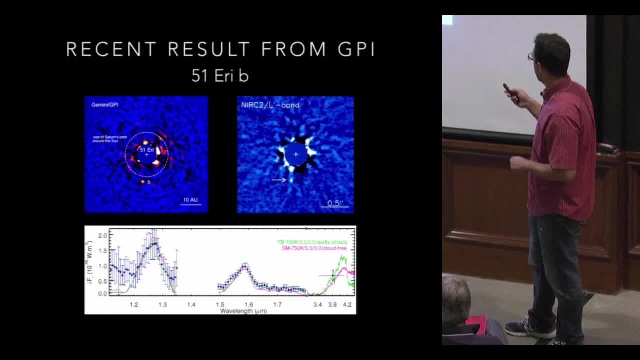 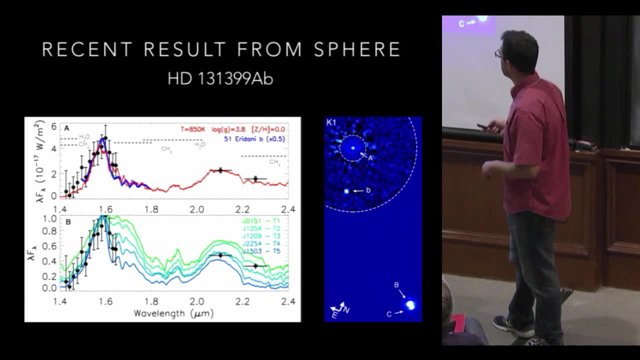 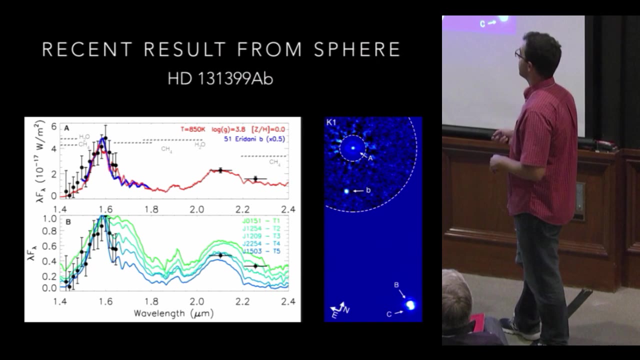 discovered by direct imaging to date, which is 51 Eridani b. SPHERE has recently announced also a very light planet in an amazing triple system. so a lot of surprises coming from direct imaging, especially these second generation surveys. The future of direct imaging is. 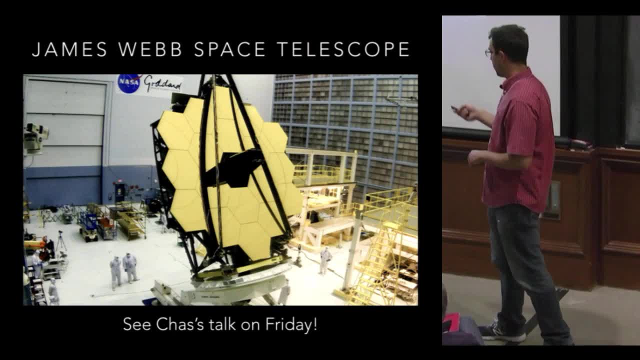 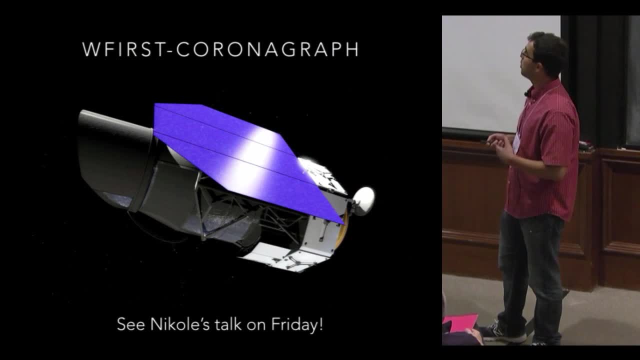 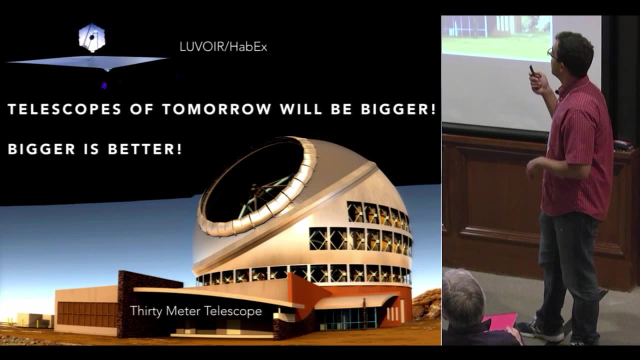 first the James Webb Space Telescope, and I refer you to Chas's talk on Friday. Of course. then, after JWST, we'll have WFIRST, which will be equipped with a coronagraph. There is a talk on Friday about this as well by Nicole. 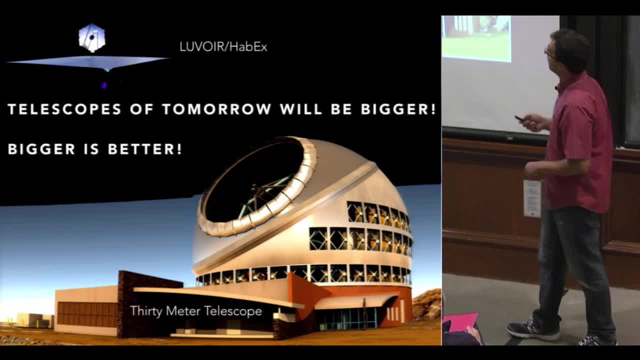 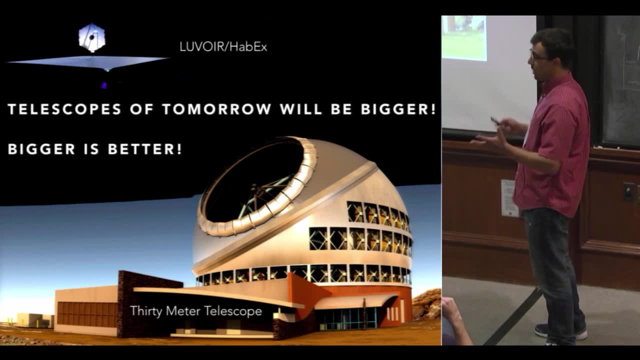 And then in 10,, 15,, 20 years from now- maybe 30 years, who knows- we'll have a new generation of space-based telescopes. So I don't know if we'll hear about that here, but there is LUVOIR and HABEX concepts. 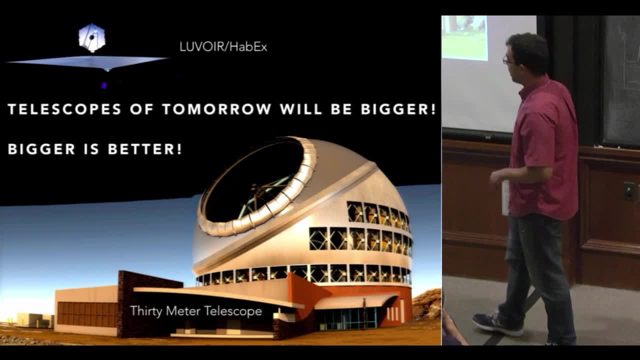 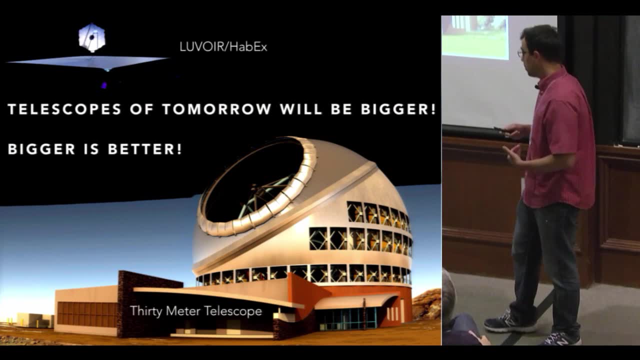 that are currently being studied by NASA And on the ground we'll have a new generation of giant telescopes, which will allow us to go way beyond what we can currently do, and the reason is that we collect many more photons and we'll have much better adaptive optic systems. 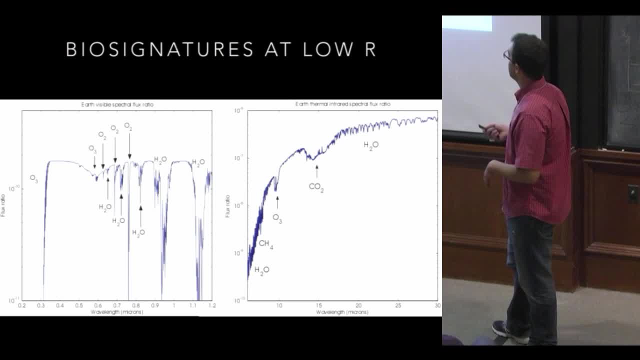 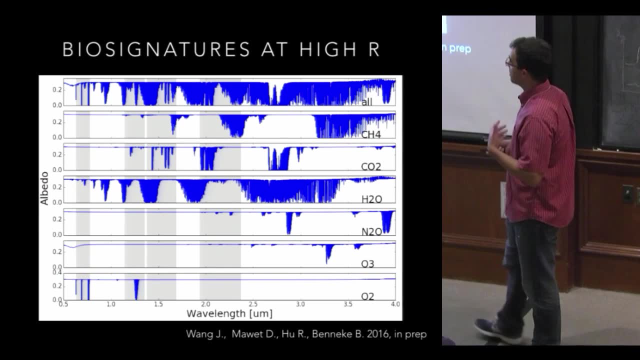 So the ultimate goal is to go after these biosignatures. So this is what they look like in the visible and infrared at low spectral resolution. This is what they look like at very high spectral resolution. So you see that that is very enticing. to go to red wavelengths. 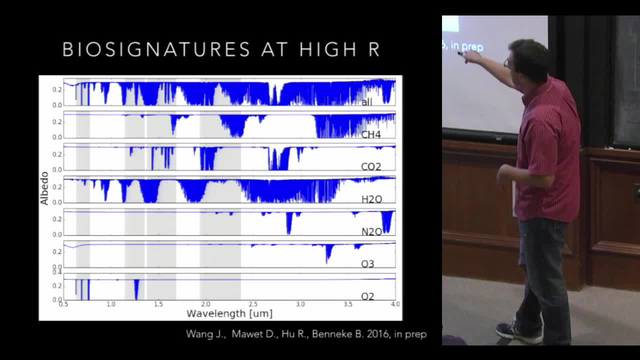 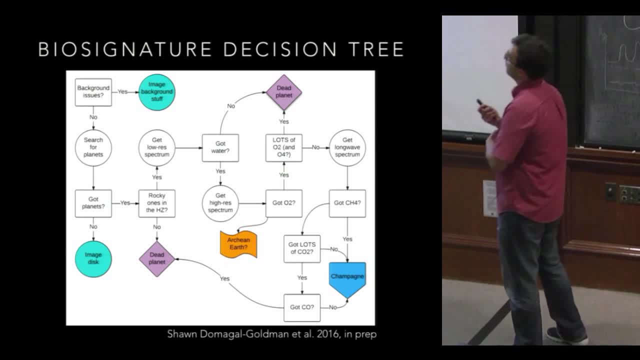 to study and characterize exoplanets, even though there are a few markers in the optical wavelengths here, like oxygen. This is a chart that is very amusing, so I just leave it there and you can see it in the slides later. This is from a paper in preparation. 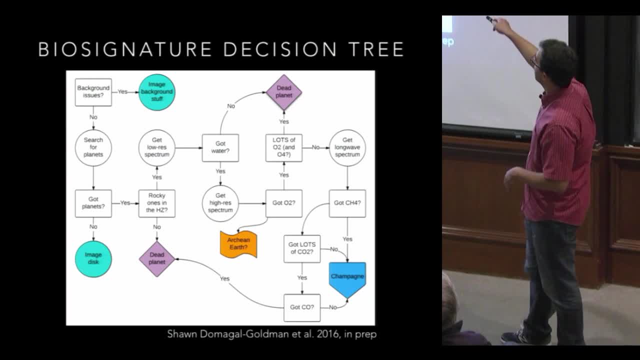 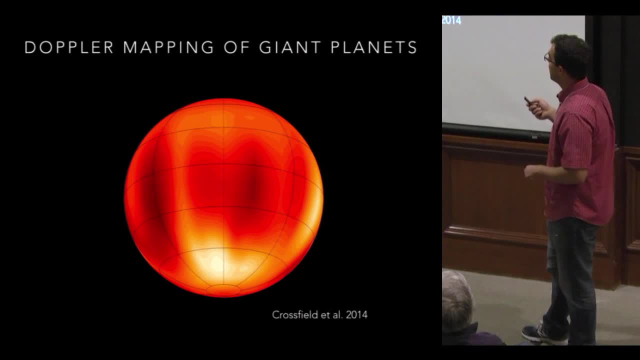 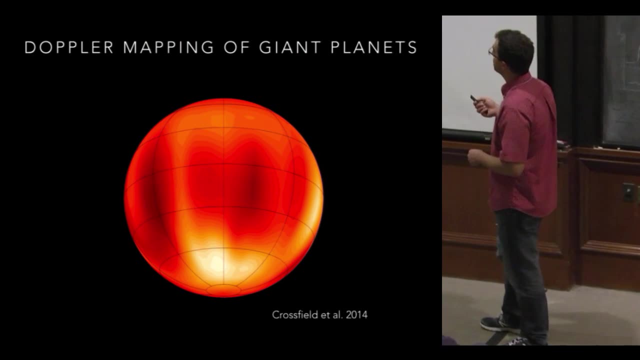 by Sean de Magal-Goldman here that shows you a decision tree when you look for biosignatures. Perhaps one of the most exciting applications of direct imaging in the near future is to do maps of extrasolar planets. Ian Crossfield a couple years ago. 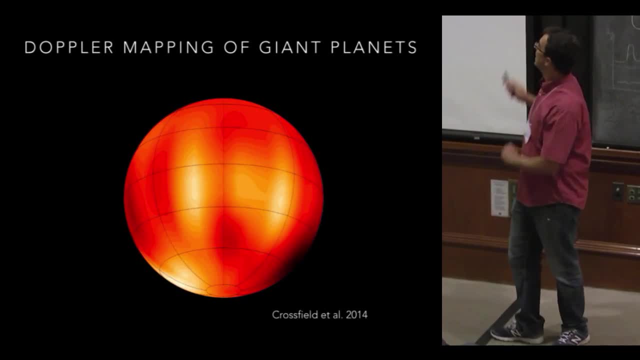 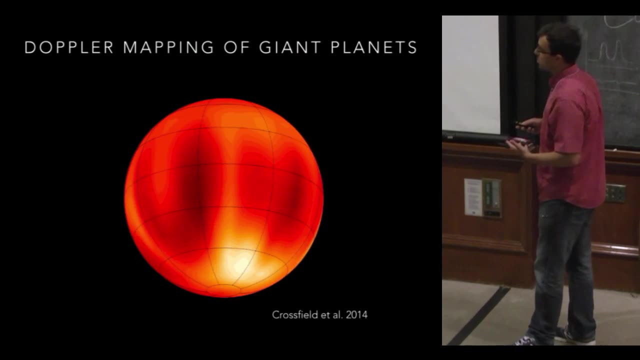 has made a map of a brown dwarf. I'm almost done. This is something that, with this giant telescope, we might be able to do someday. So, using very high spectral resolution, spectroscopy and direct imaging techniques, where one can isolate the signal of an exoplanet. 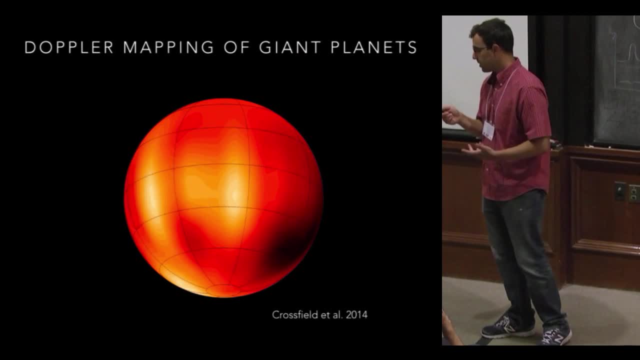 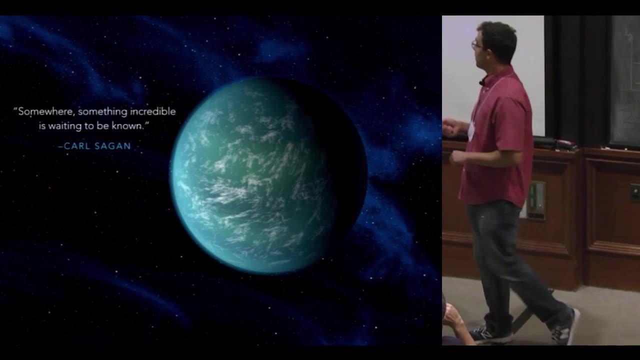 we will be able to do these maps- Doppler maps of the surface of exoplanets, like Ian did for brown dwarfs. Okay, so I've just finished on this quotation quote from Carl Sagan. This is the Sagan workshop after all. 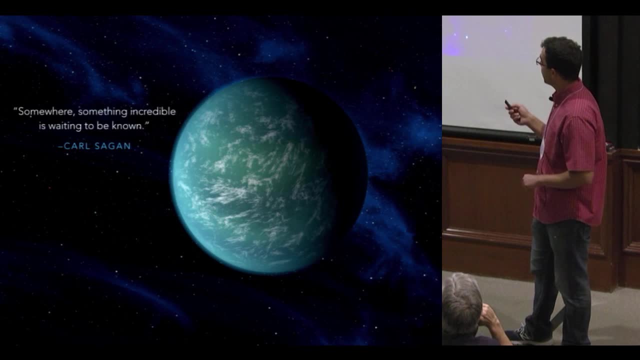 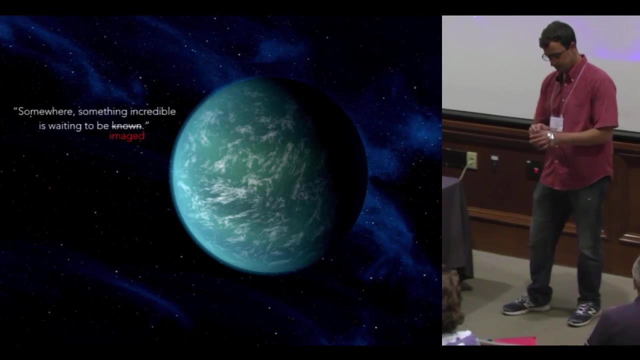 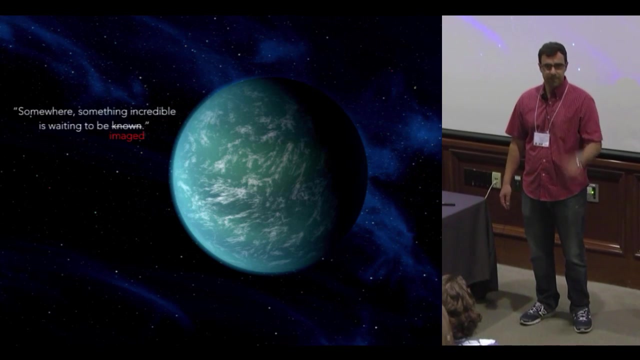 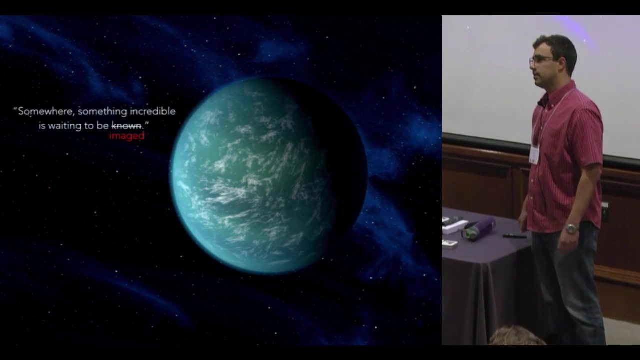 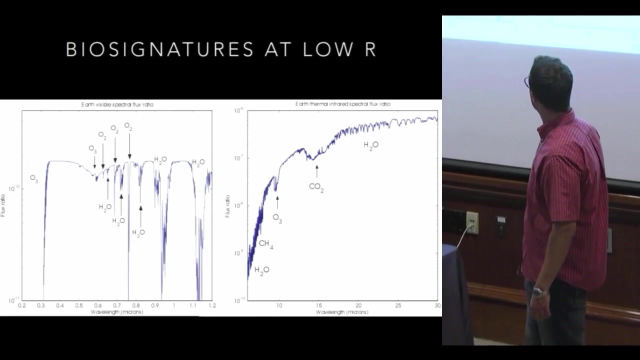 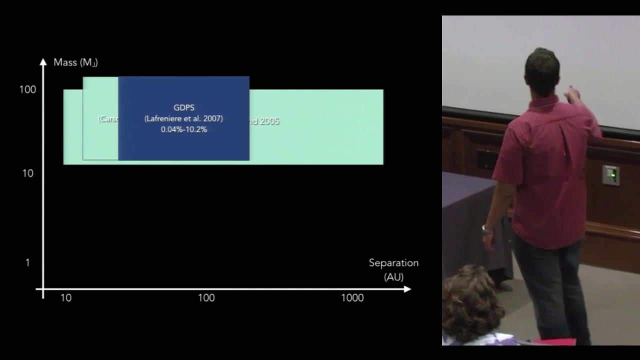 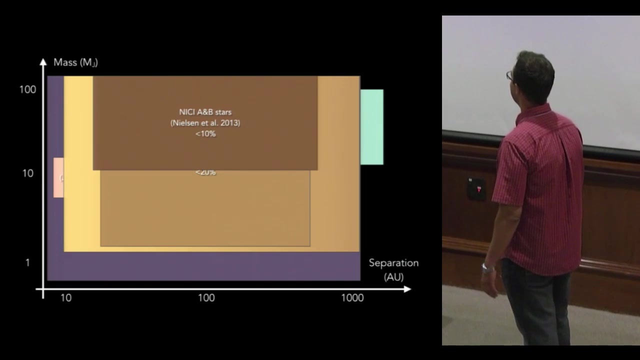 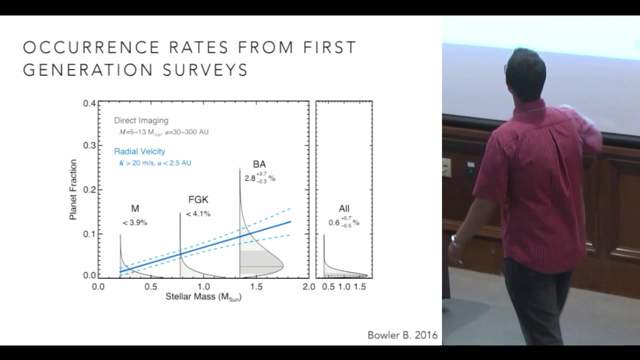 I just modified it slightly. So somewhere, something incredible is waiting to be imaged. Thank you Questions: We have a couple of minutes. Yes, This one, Yeah, Oh, no, Sorry, A lot of work. One has to show respect to 20 years of work. 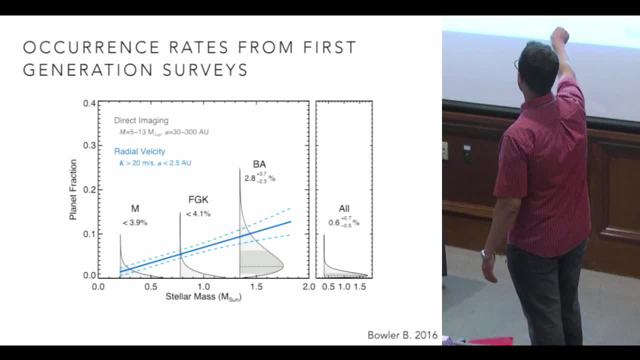 So these are the posterior distribution of the occurrence rate of planets around different spectral types. So this is for M, FGK and AB stars And you see here where the distribution peaks is the occurrence rate. So you see that we haven't found any planets. 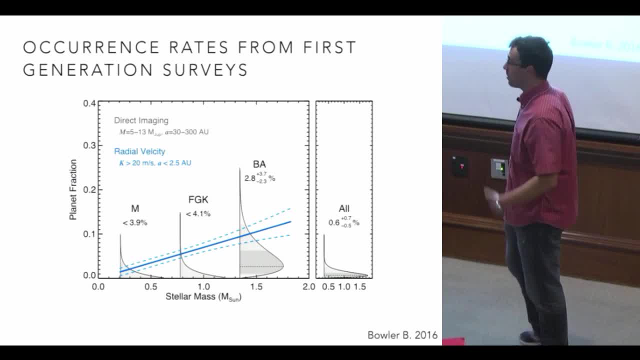 around M-type and FGK stars. So we have only upper limits there, And so you see the tail of the distribution only, And so this is just integrating over all spectral types. Okay, So planet fraction is a function of stellar mass here. 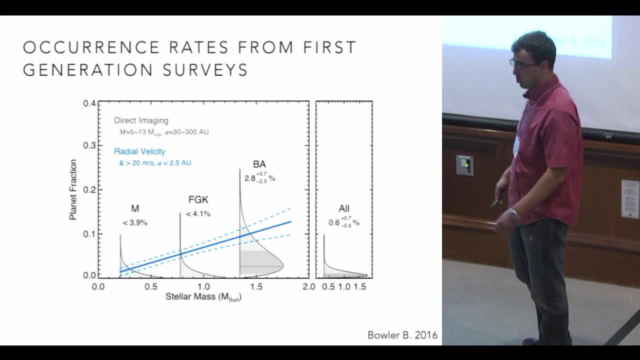 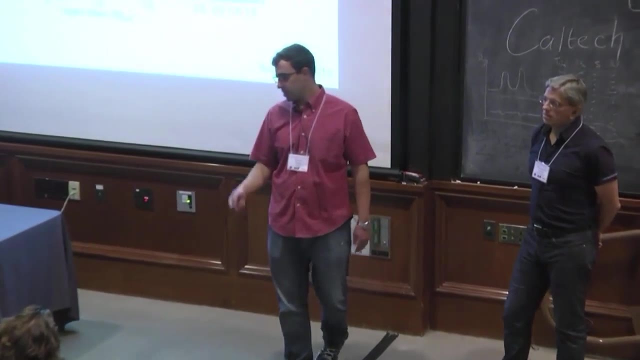 And this is the combined result for all spectral types that have been probed. Okay, So you see that that plot actually indicates that we found planets only around A-type stars. Describe that a little bit. Absolutely Excellent question. So these isomasses plots? 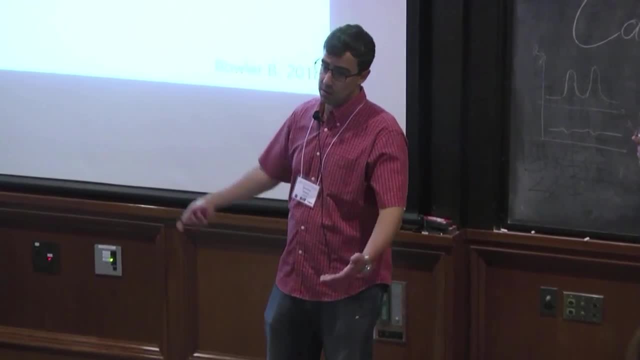 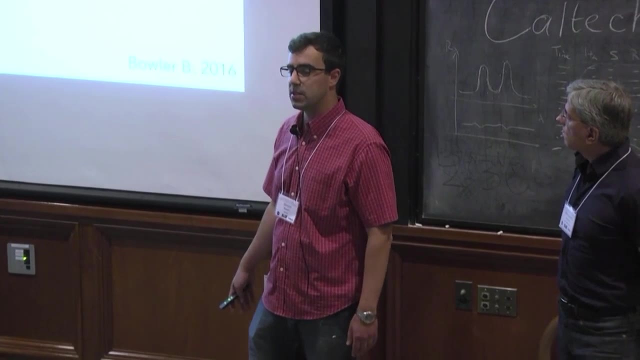 are heavily dependent on models, which is also another issue, is that this boundary here is heavily dependent on models, And so there is also an uncertainty there based on due to the fact that if you change a model, sometimes the result can change dramatically. 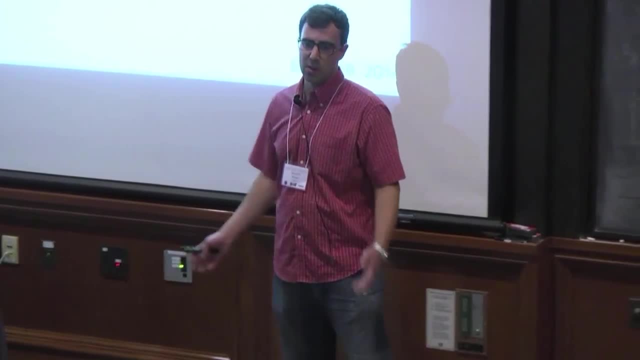 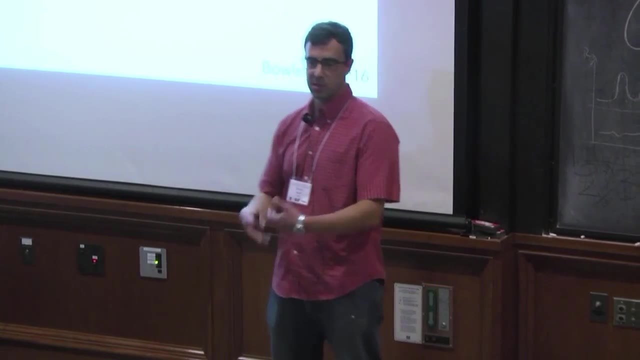 And, in particular, there are two families of models. There is the hot start model, high entropy models and there is a cold start model that are closer to representing what happens in core accretion, for instance. And the difference between these two families of models. 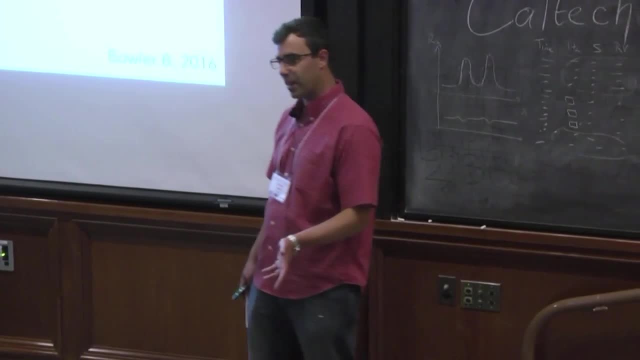 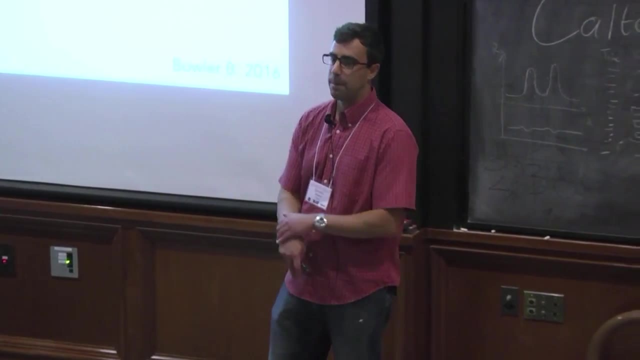 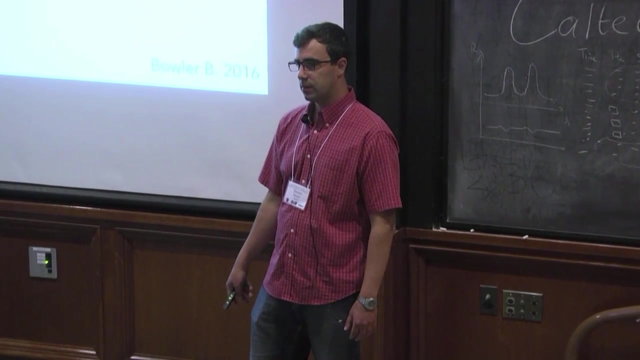 as a function of age is quite dramatic. So we don't really understand well how planets evolve in the first few million years. And all these results are subject to these uncertainties. One only last quick question: The model was also always seen as a planet.